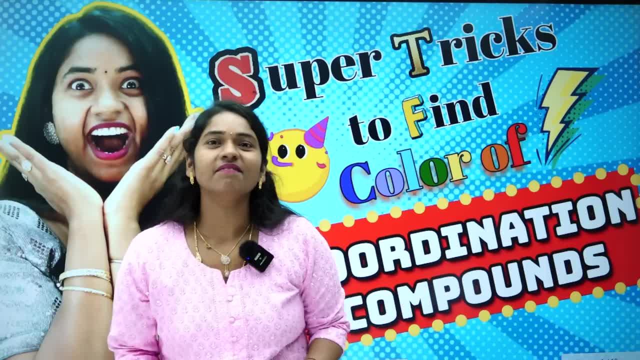 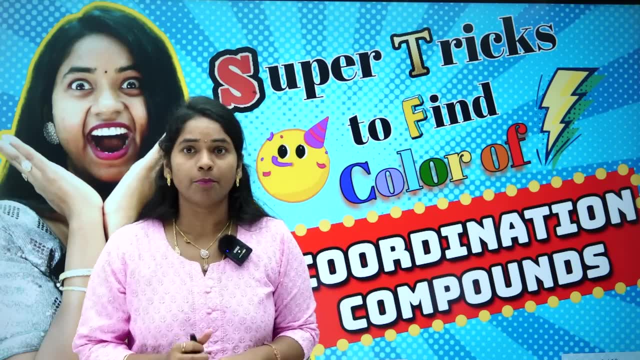 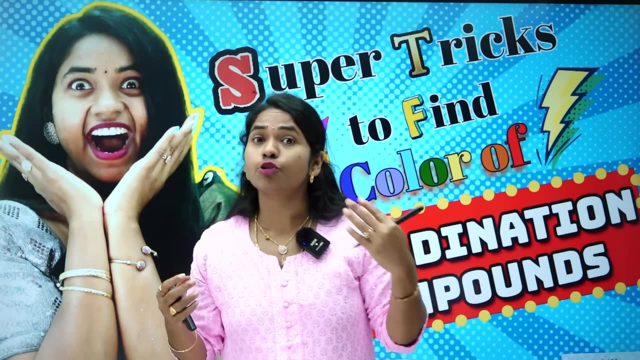 Hi students, I'm your Komali ma'am In this session I'm going to teach you super tricks to find color of coordination compounds. Actually there are many colors. If you see the coordination compounds, there are so many metals, so many ligands. different colors are possible. So how to? 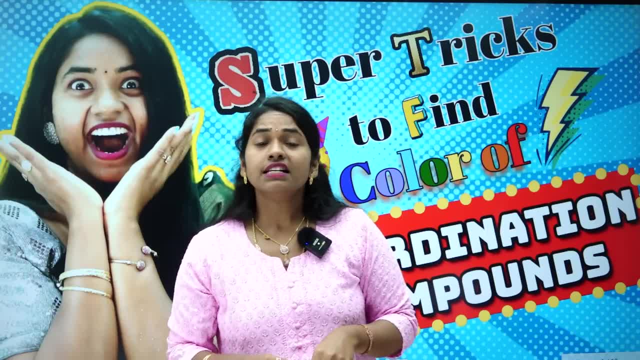 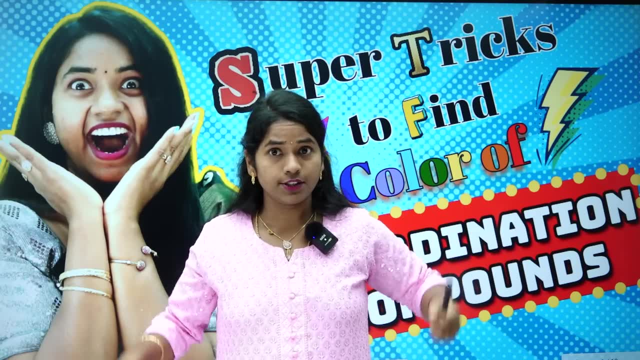 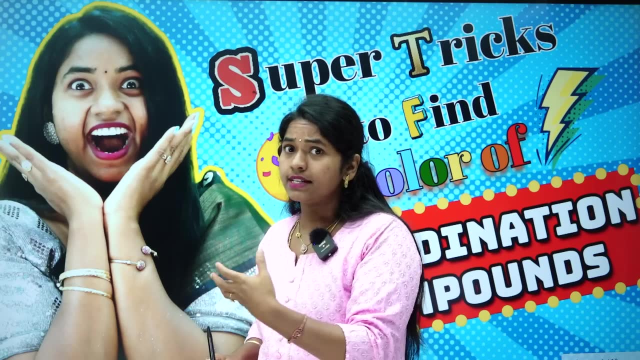 find the color of a coordination compounds. See, there are many complexes, many colors. You no need to worry that. to remember all the colors of the coordination compounds, There are certain techniques and strategies. If you know this, whatever I'm going to cover in this video. 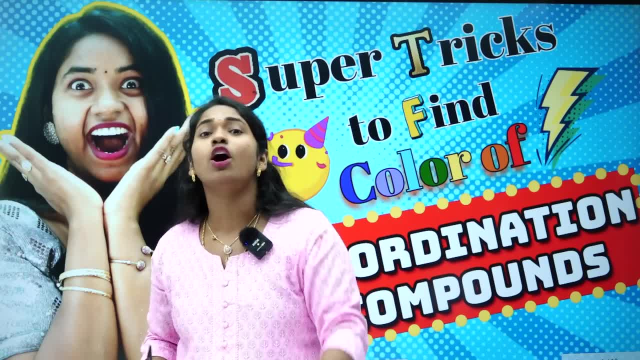 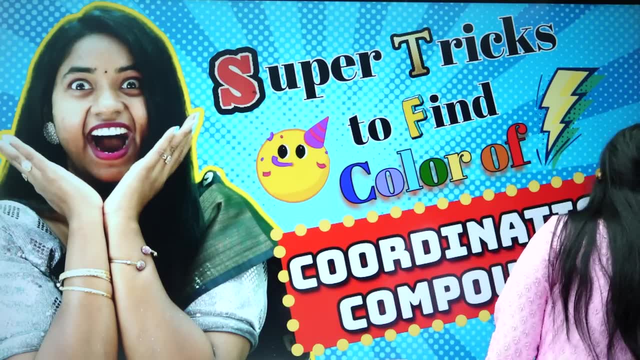 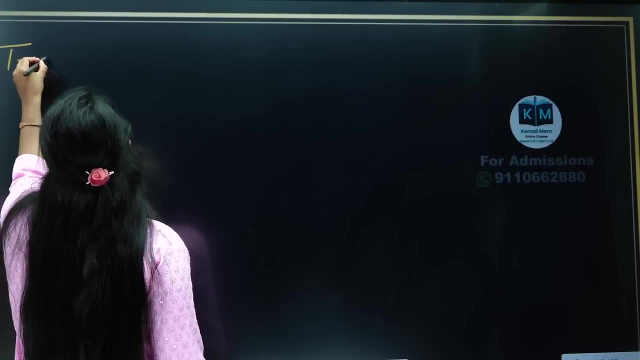 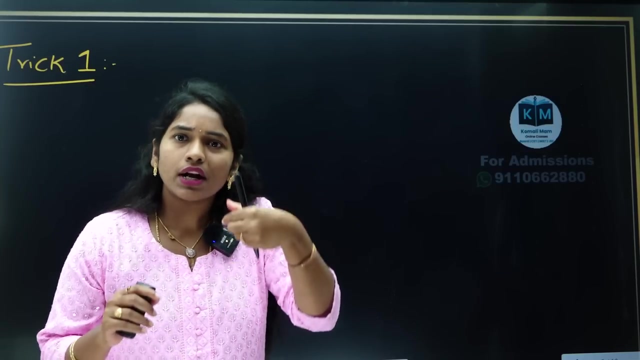 that's enough. Any question from coordination compounds you are going to solve very easily. Let's begin the session. Are you ready, everybody? Let us see trick number one Here. in this I'm going to tell you few important things. In trick number one I'm going to teach you what is a primary color, what is a secondary color. 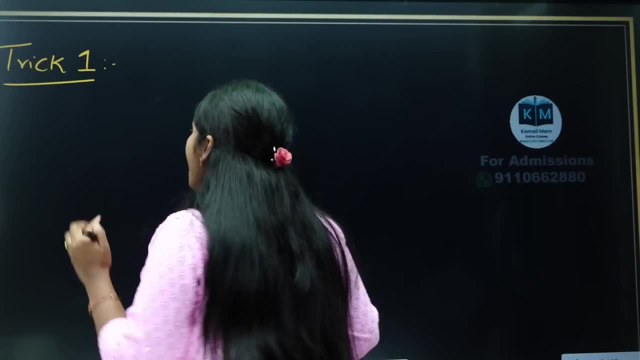 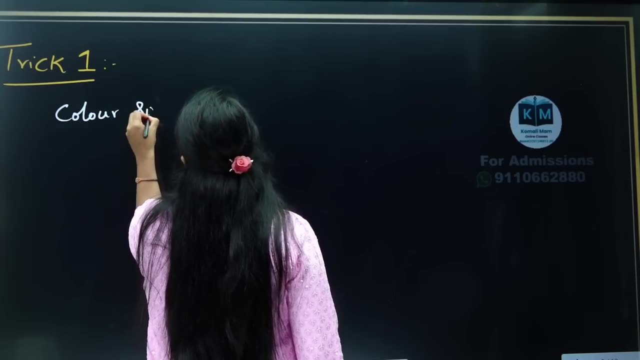 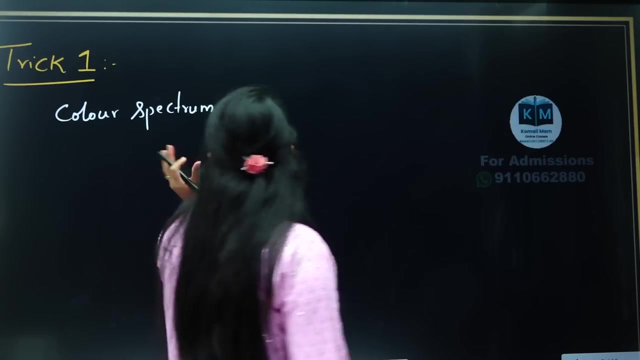 what is a tertiary color? what is a color spectrum? See color spectrum, color spectrum. color spectrum means our human eye can see only visible part of the electromagnetic radiation, Only visible region we can see, that is Vibhgi, or only this color. 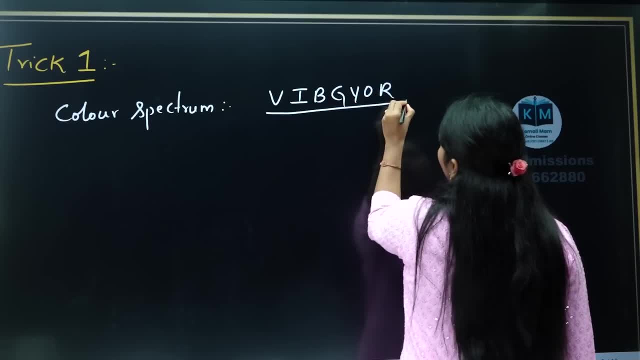 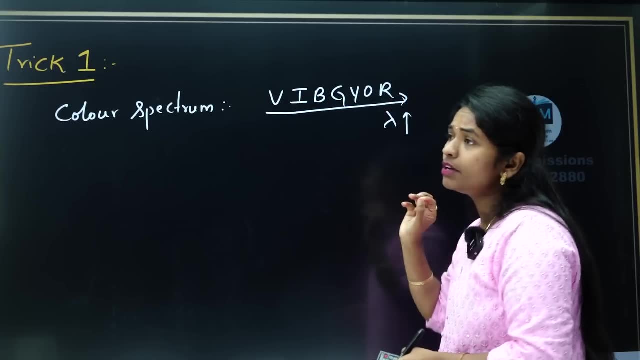 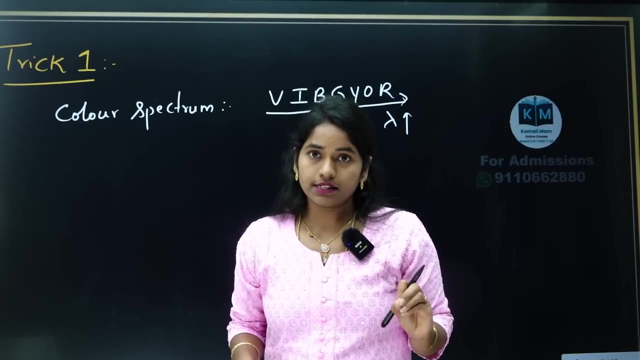 we can see Vibhgi or okay. This Vibhgi or is in the order of increasing wavelength. Increasing wavelength means red is having more wavelength, Okay. And in this Vibhgi or of seven colors, there are some primary colors. means what is the meaning of primary color, These colors? 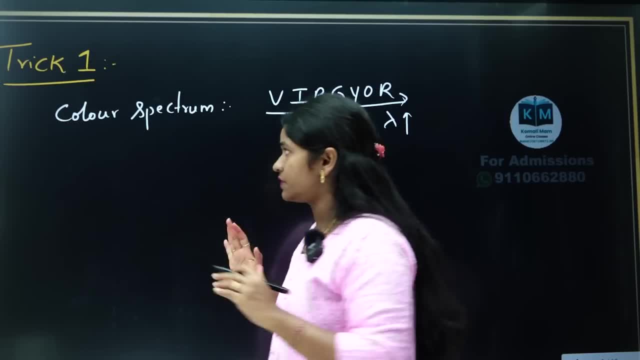 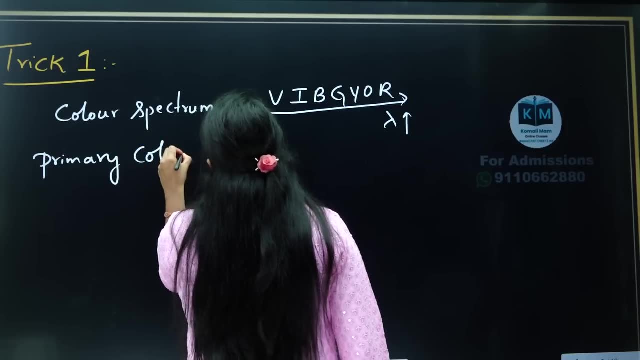 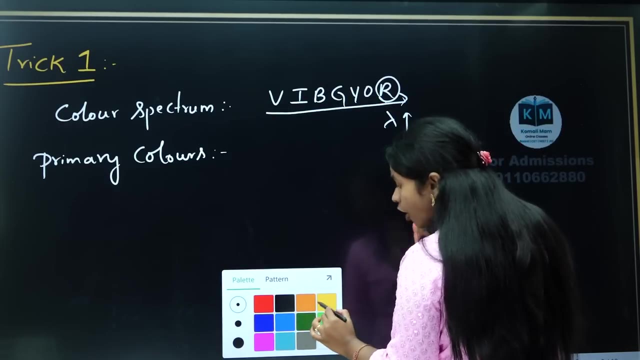 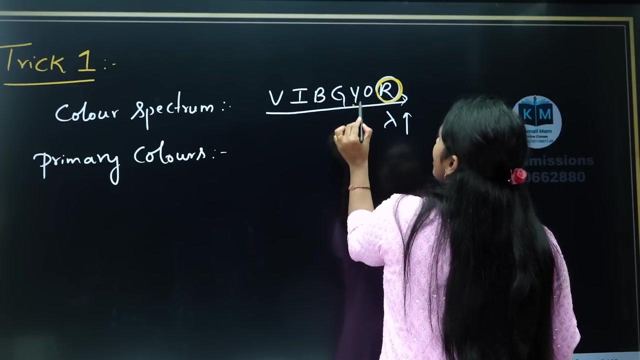 cannot be obtained by mixing any of other colors. For example, let us see primary colors. primary colors: What do you mean by primary color? Students, tell me which is obtained, which cannot be obtained by mixing any other colors. See how easily you can remember. are red color: leave orange and take next one. leave green, take next one. 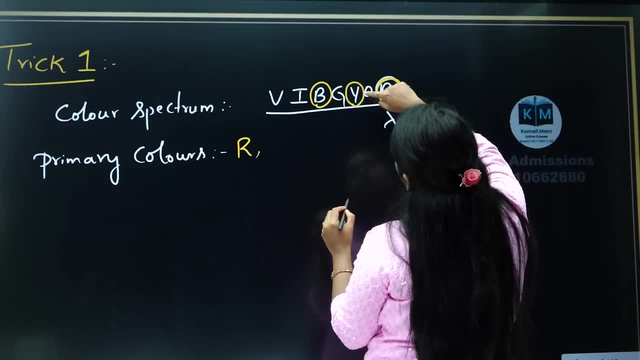 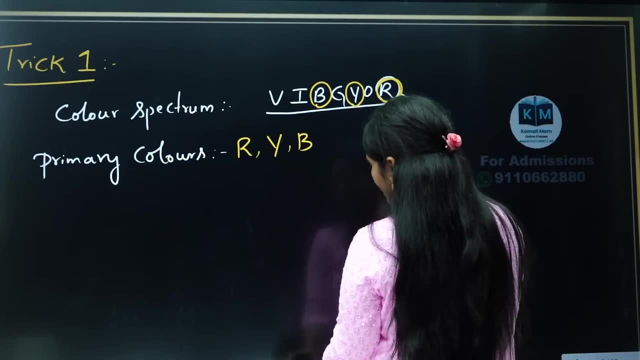 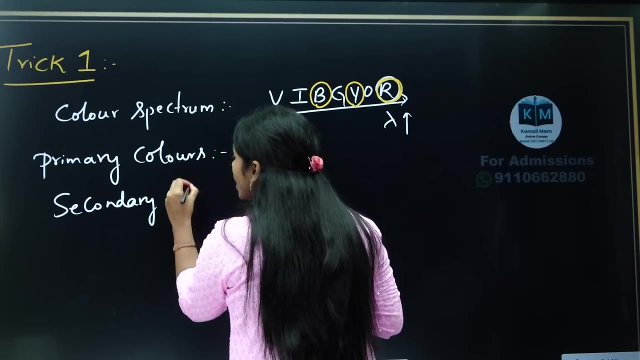 So, red color, leave the next one, take yellow, leave the next one, take blue. These are red, yellow, blue. These are primary colors, See the next one Secondary colors: What do you mean by secondary colors? These are the colors which are obtained by mixing. 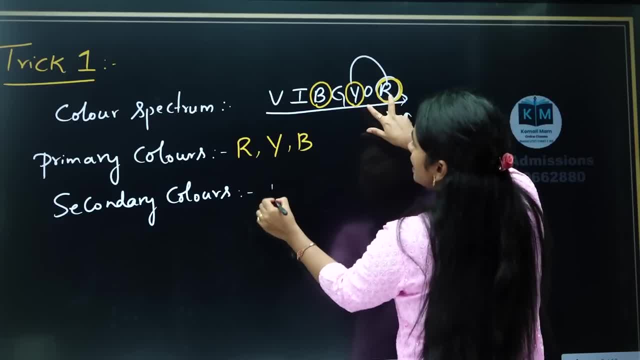 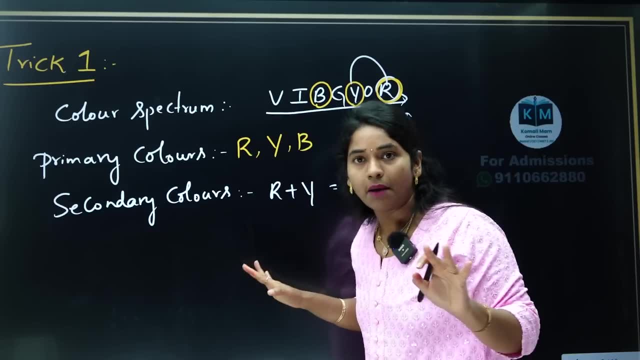 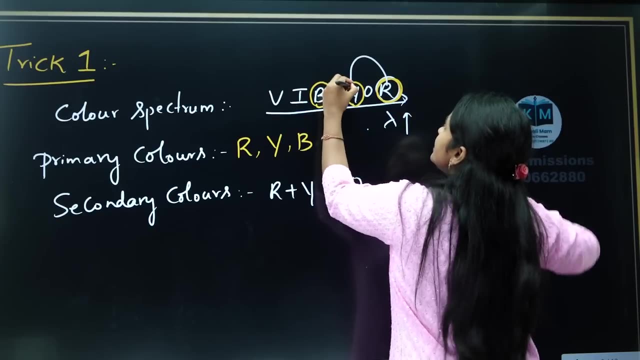 of primary colors. Now take the combination of these two: red plus yellow. See how easy it is. Follow me how I'm doing. Watch this video up to the end. you will be very happy. Red and yellow: mix these two, You get the middle color. What is that? Orange. Now mix these two. 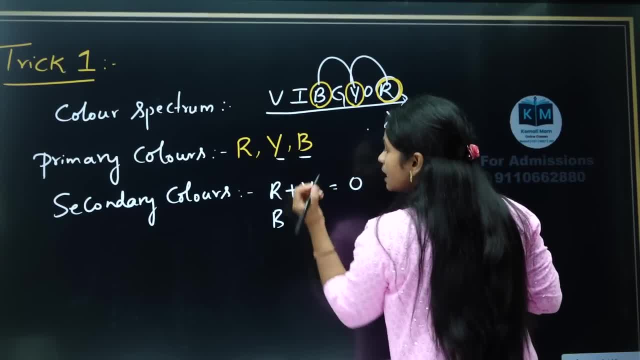 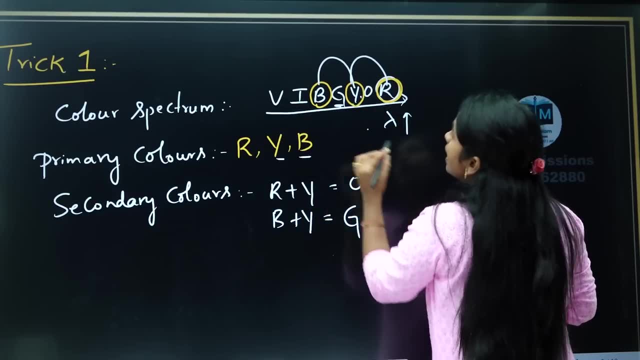 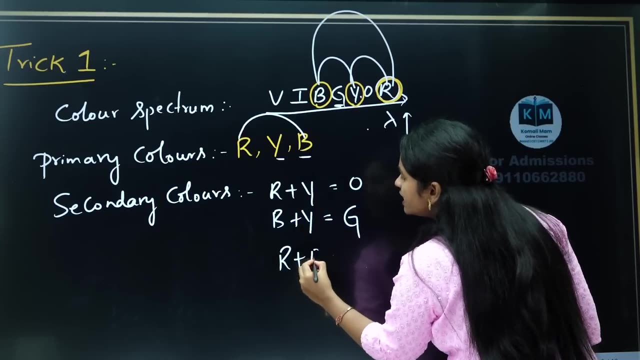 Blue and yellow. See blue and yellow. these are primary colors. Mix these two colors. If you mix blue and yellow, you get middle color. What is this color? Green color. Now you mix these two. What are those two? Red and blue color. Mix red and blue. These two are primary colors. If you mix these two, you get a violet color. Understand. 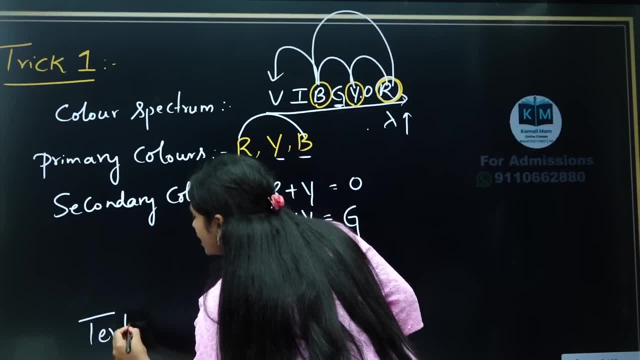 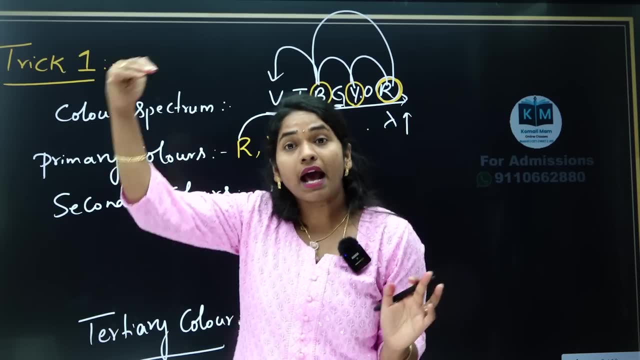 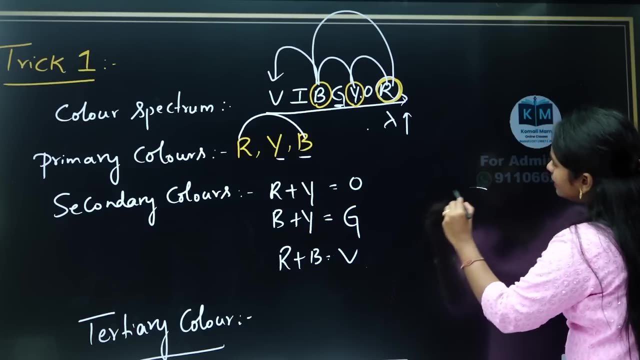 Now let us see tertiary color. Tertiary colors are the colors which we get by mixing primary colors with the secondary colors. So you take any of this color and you mix. For example, I will write the color wheel. This is a color wheel. Okay. 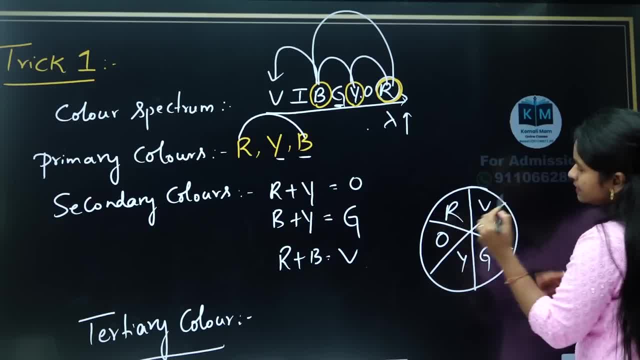 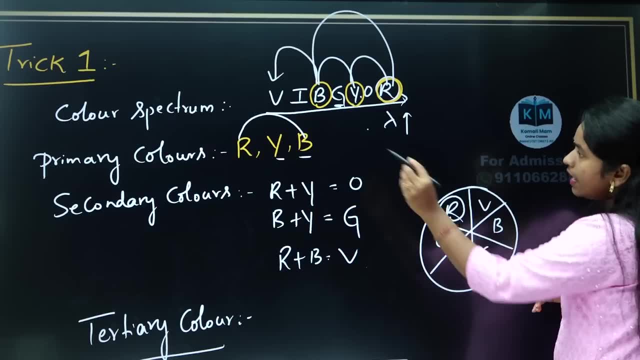 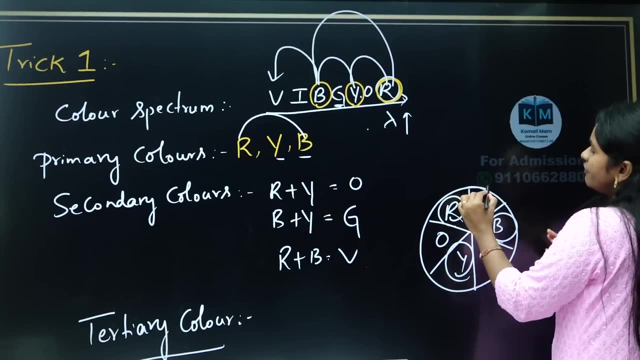 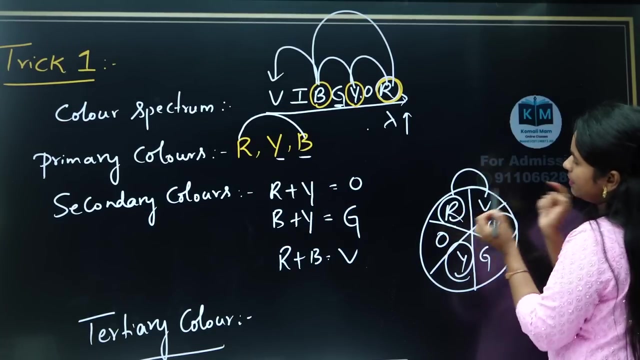 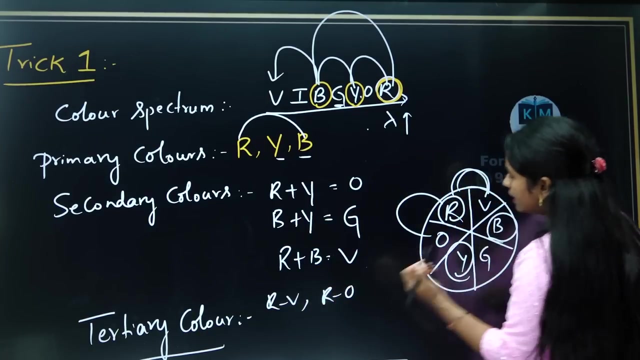 Vibgi or This is a color wheel: Vibgi or This is a color wheel. Now what I am going to do is I am going to mix any two colors. See, red is a primary color and yellow is a primary color and blue is a primary color. So now you take any of the two combination, For example, adjacent These two: This is a secondary color, violet, Red is a primary color. Mix these two: Red violet One color. Red orange One color. Yellow orange One color. 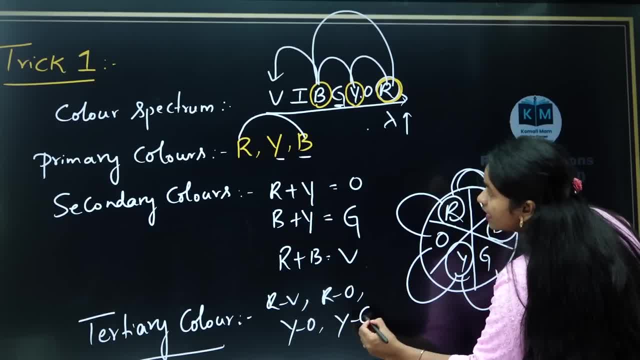 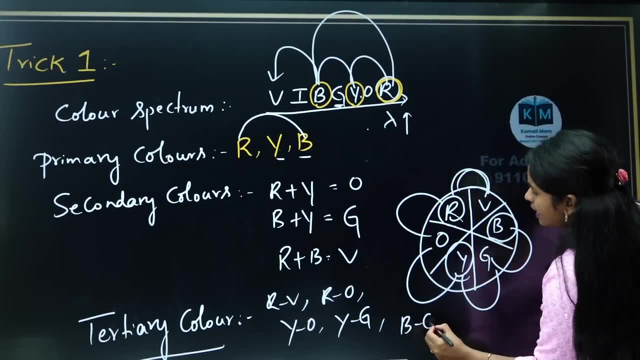 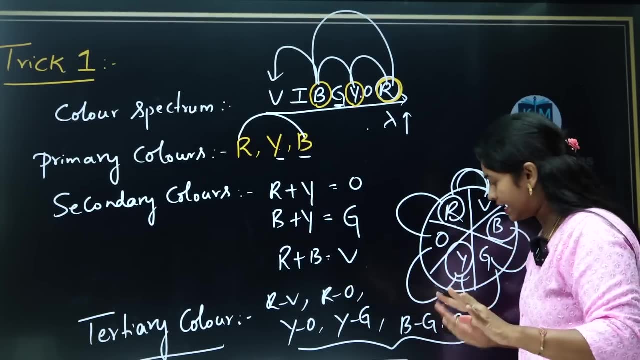 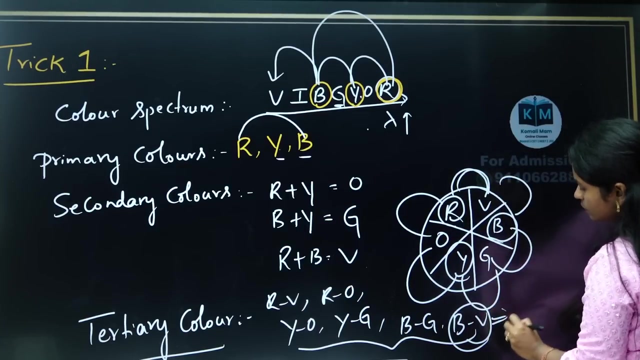 tertiary color. Next, these two combination: yellow, green. See here, yellow is a primary color, green is a secondary color. Next, blue green, Next one, you see, blue violet. These are total six secondary tertiary colors In this blue violet combination. we call it as indigo. So tertiary color: blue plus. 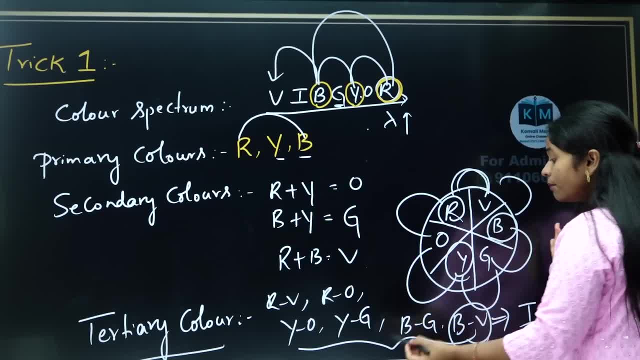 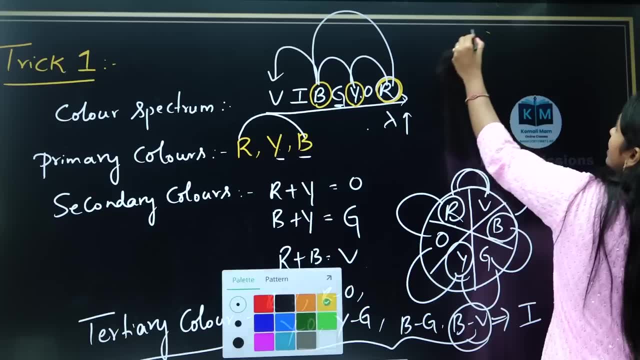 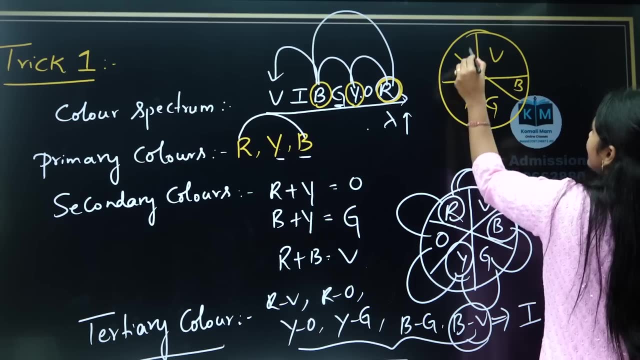 violet combination is called as a indigo. So what I am going to do here is I am going to: I did not write that indigo in the color wheel. See here, I did not write indigo in the color wheel with gr. I wrote. You also write like this. and here I want to tell you the complementary color, Just 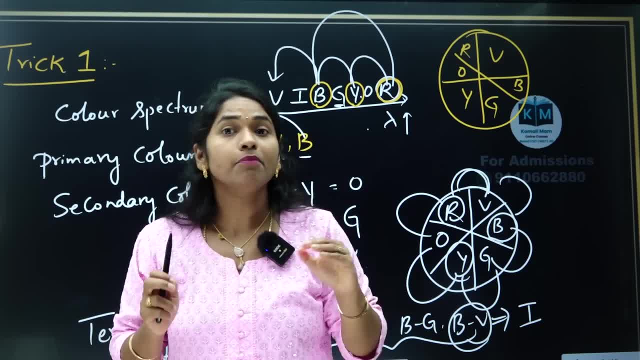 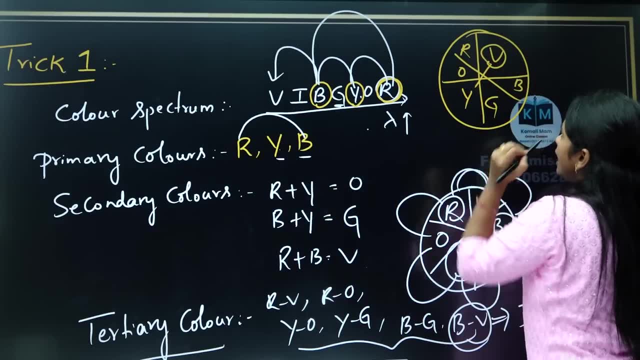 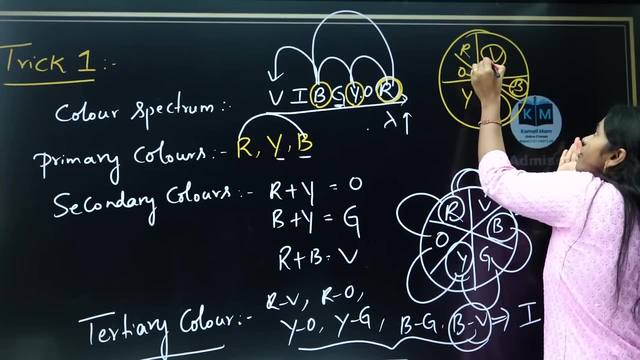 see what is complementary color After some time. I am going to tell you how to find the complementary color. Are you observing? Violet opposite color is yellow and blue, opposite color is orange. Green opposite color is red. Are you understanding? So violet color complementary is yellow, Green, complementary is red, Blue. 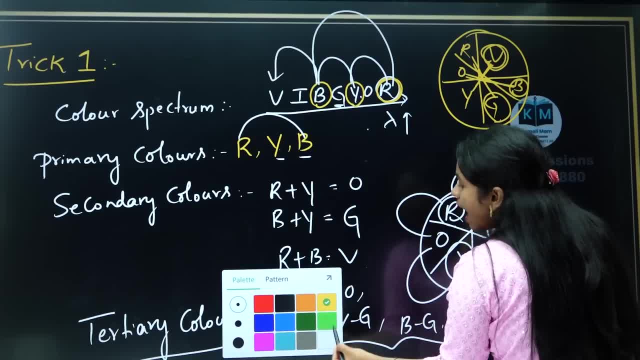 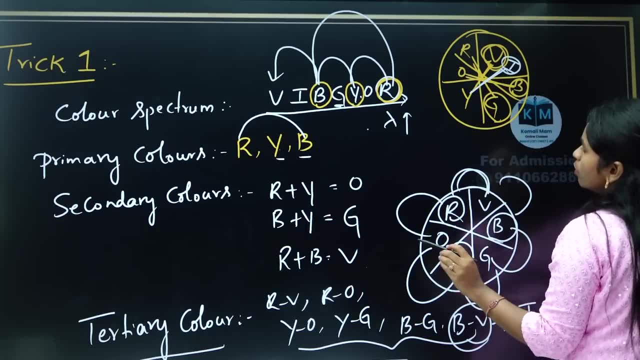 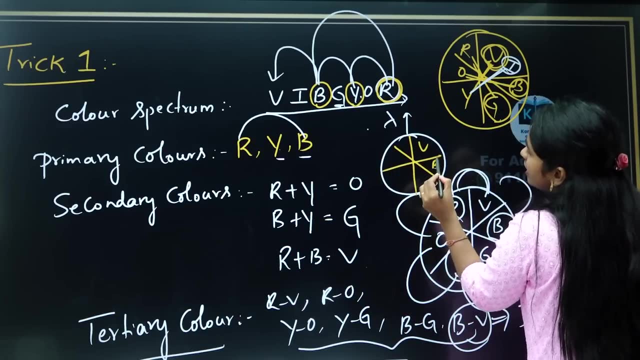 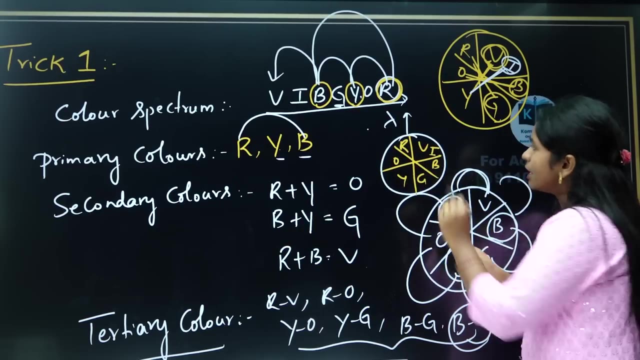 complementary is orange. And now what I am going to do is I am going to place this indigo also next to violet, because it is a complementary color, also yellow. So how you should write, students, tell me You have to like this. First write v, b, g, y, o, r. You can write later. i also along with a v, because for both complementary color is yellow. 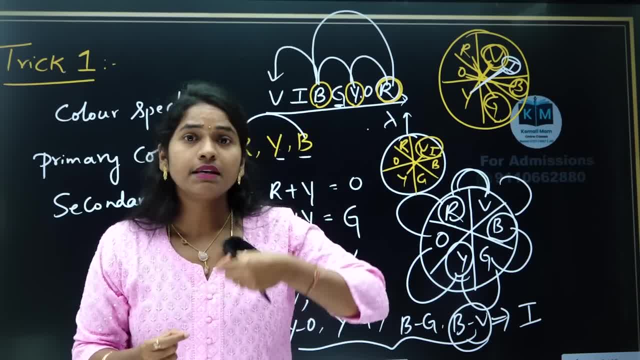 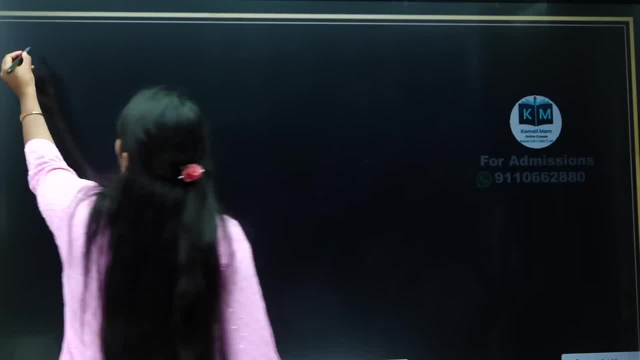 Till now, I did not tell you what is complementary color. What is the meaning of complementary color? Now I am going to tell you under trick number 2.. In a trick number 2, I am going to tell you how you can get the color of the. 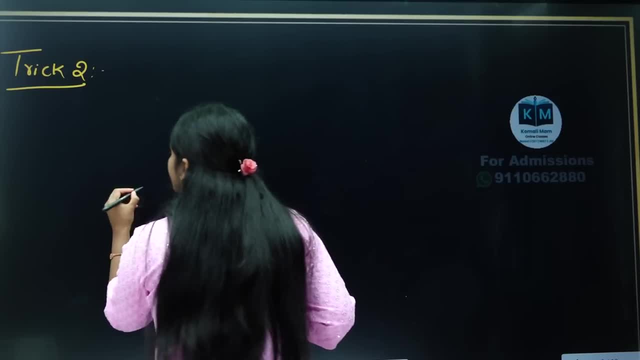 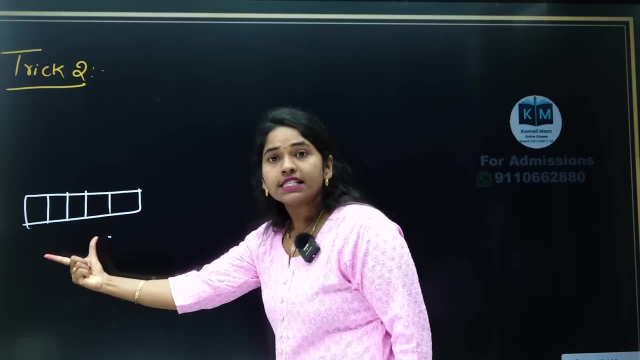 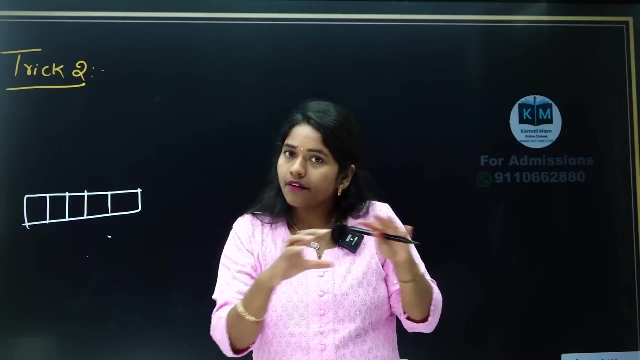 compounds. if you see metal orbitals, metal have 5d orbitals: 1, 2, 3, 4, 5. all the 5d orbitals are having same energy and when light falls on this or see, all are having same energy, right? so these? orbitals. we call it as degenerated orbitals. what is the meaning of degenerated orbitals? orbitals which are having same energy, but when ligand approaches, these d orbitals loss their degeneracy and these 5d orbitals goes to the excited state we call them as a barycenta. this 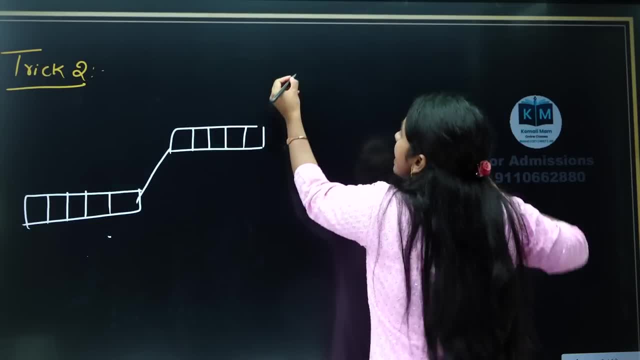 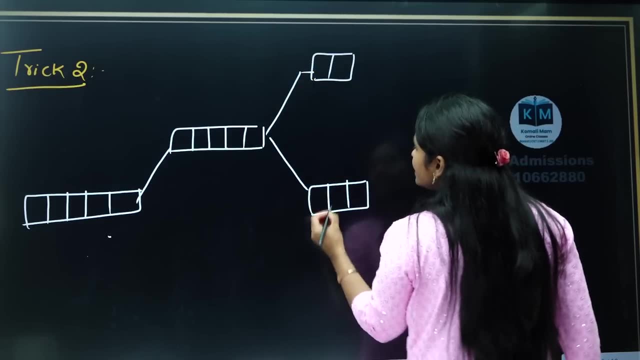 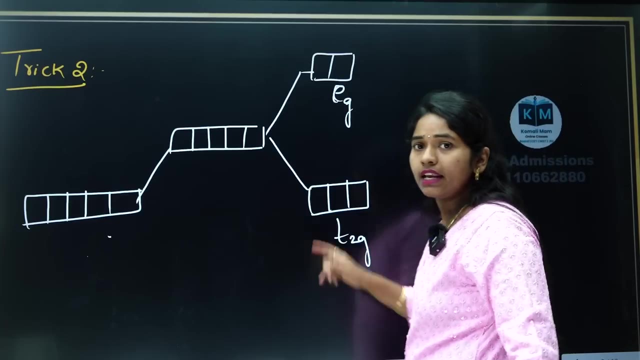 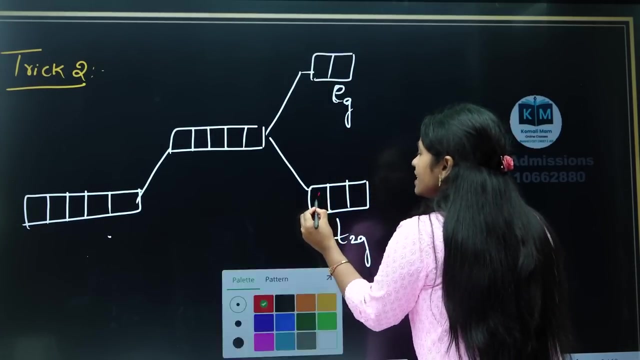 is barycenta, which means it is about to split. it splits up into actually two sets. what are those two sets? one is t2g set, another one is eg set. this is the concept which you studied in c, c, c, F, T, crystal field theory. there I explained you about this, and here electron, if any electron is. 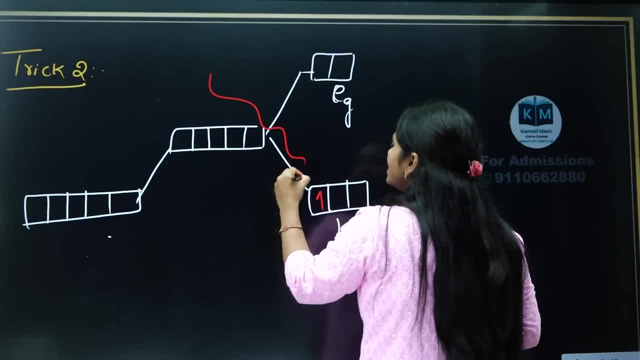 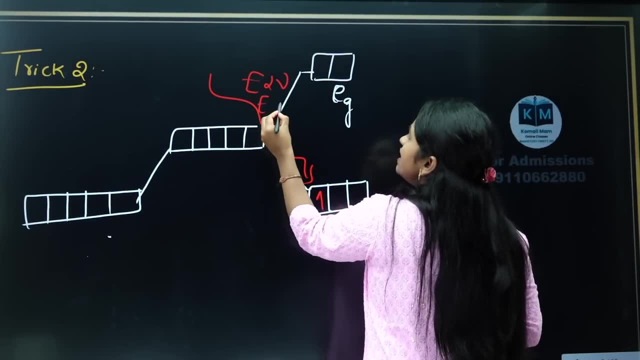 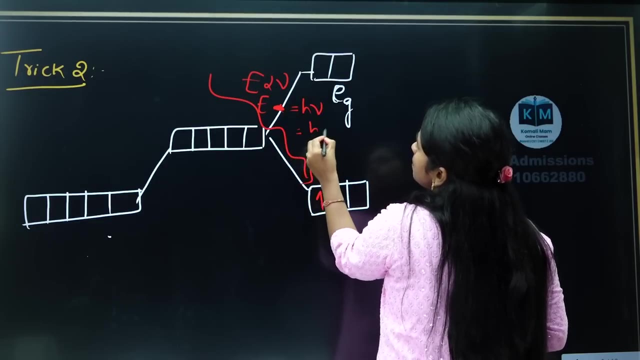 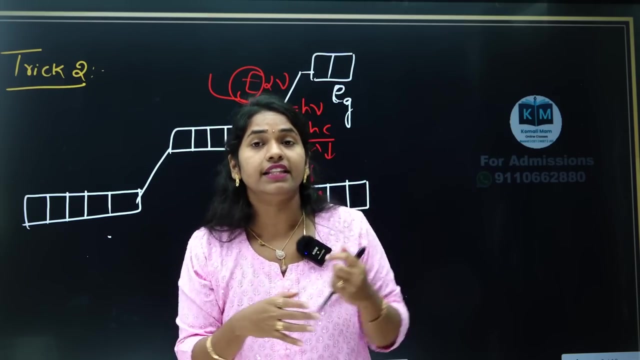 present in t2g. if light with a certain energy falls, energy is directly proportional to frequency. energy is inversely proportional to wavelength. so remove proportionality. put planks constant, h, nu, nu is nothing but c by lambda. so more energy, less wavelength. more energy radiations, less wavelength if any light falls on this electron. 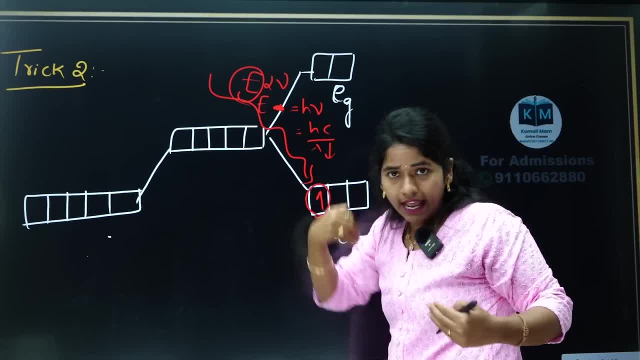 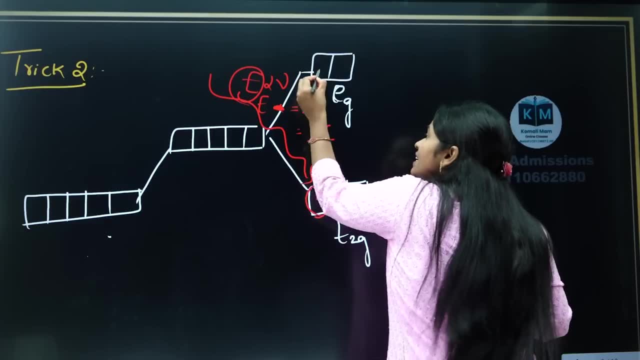 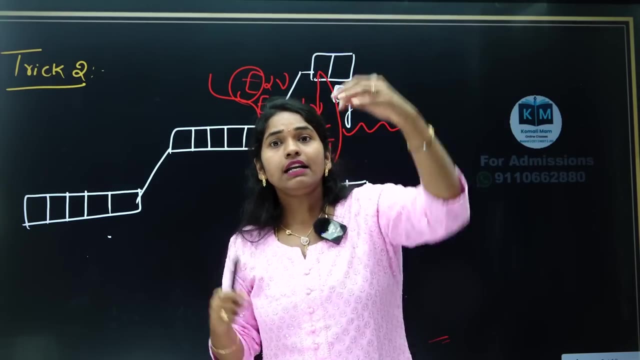 then this electron absorbs some part of that energy and it goes to the excited state. it is not stable again. it tries to come back. when it is coming back, it emits the radiation whatever it is absorbed. see, if you pass the white light. white light is a combination of seven colors. what is? 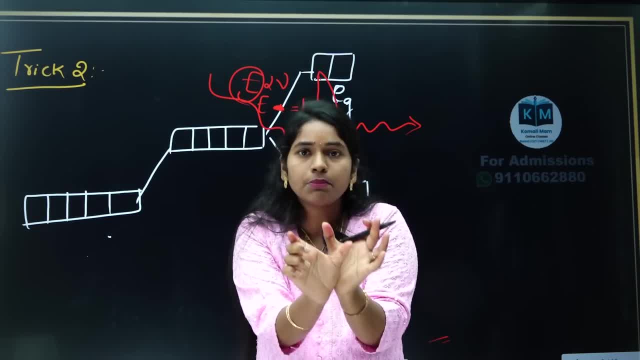 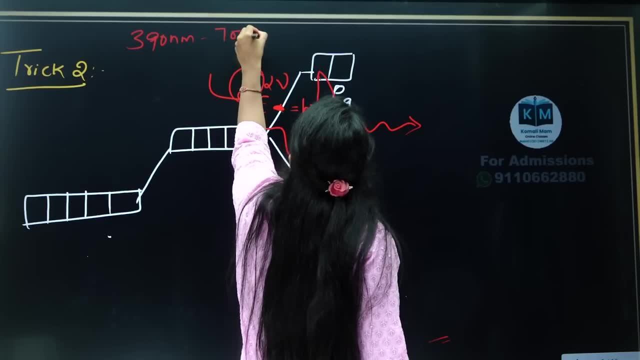 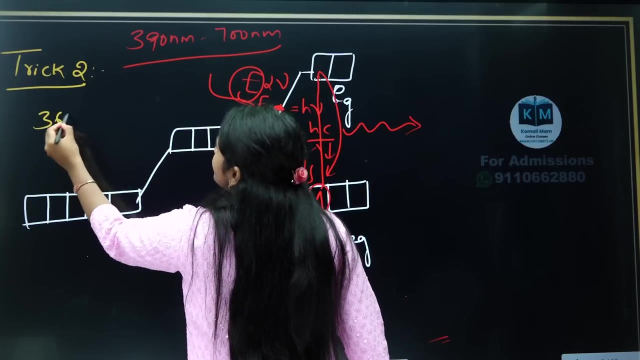 that with gear? with gear only the white light is the combination of seven colors. what is that with gear? with your? only we can see that is a visible part. visible part, radiation nano, 390 nanometer to it is around 700 nanometer. you know it varies. little bit variation will be there few day authors they mention it is. 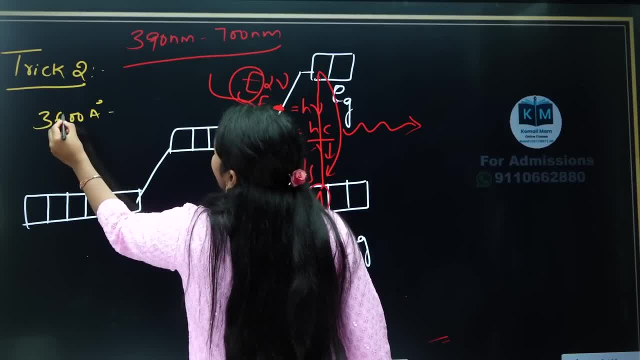 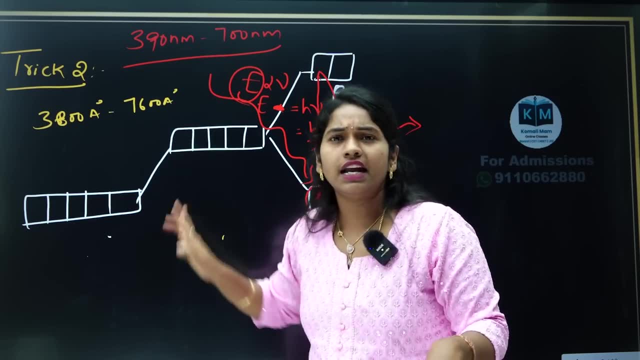 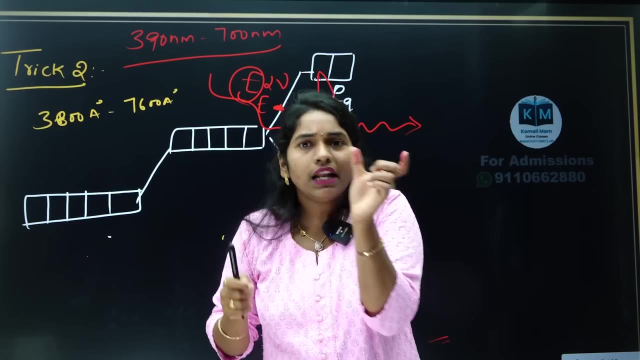 three thousand six hundred angstroms to three thousand eight hundred angstroms to seven thousand six hundred angstroms or few. they say seven, three thousand six hundred to seven thousand eight hundred. this little bit variations, few. they mentioned three hundred eight nanometers to 760 nanometer. like that small variation will be there, but this in this region. 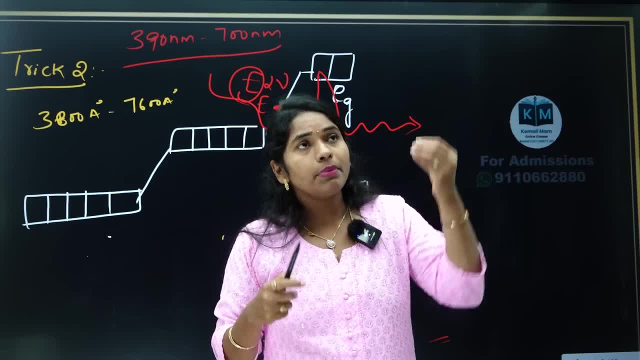 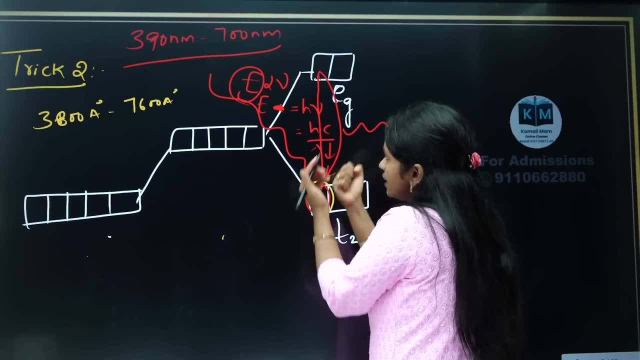 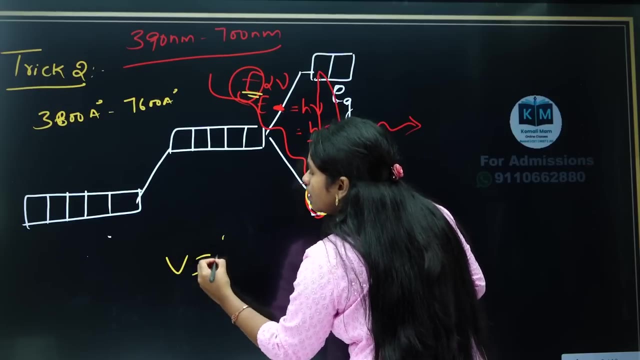 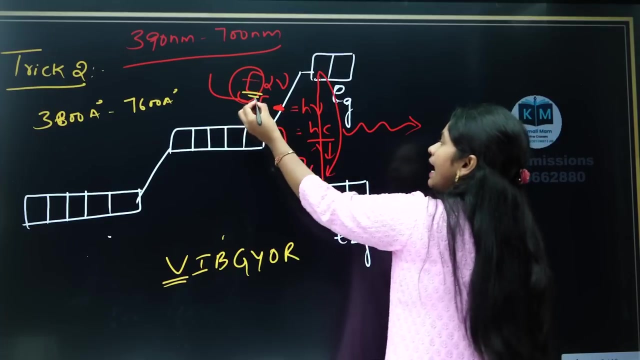 only our eye can see those colors. what happens is when light falls on this electron, on this cell, it absorbs some energy in that radiation, electromagnetic radiation in with gear. it with gear, with gear, for example, it is absorbing violet radiation. this light, is this electron absorbing violet radiation? then in the color will it? 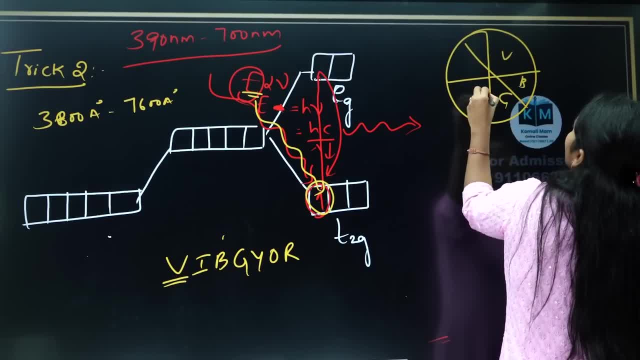 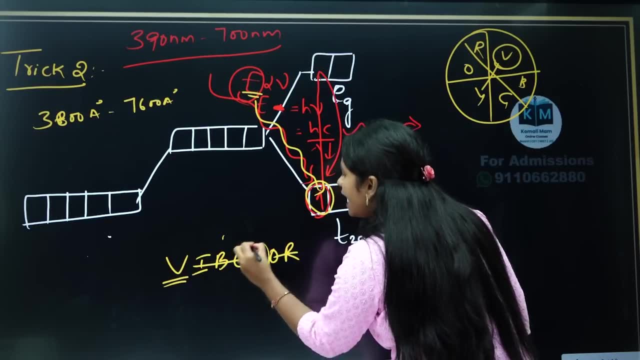 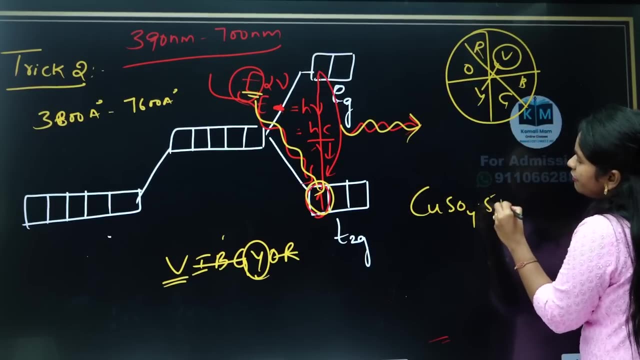 is very easy for you to find: wave GR. what is the color will here? violet? opposite is a low, so all these radiations will be neutralizes, a low light it will emit, for example, copper sulfate. if it is in blue color, it is appearing as a blue color. 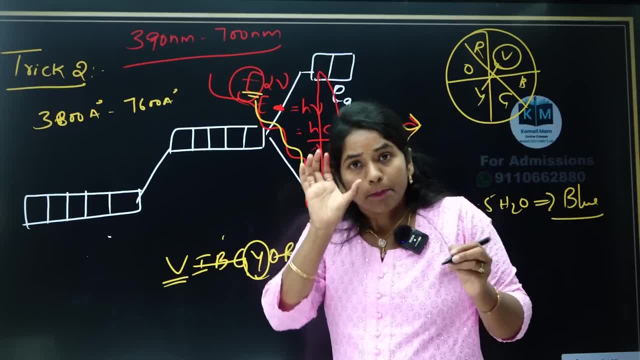 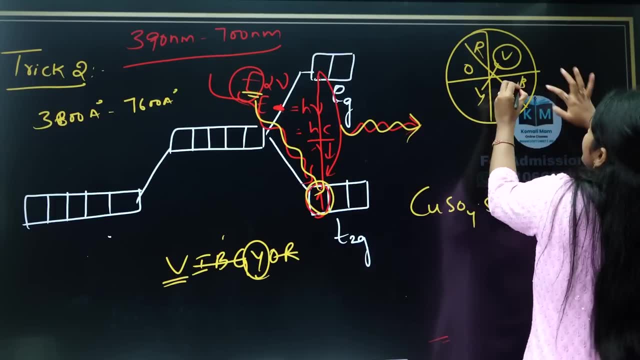 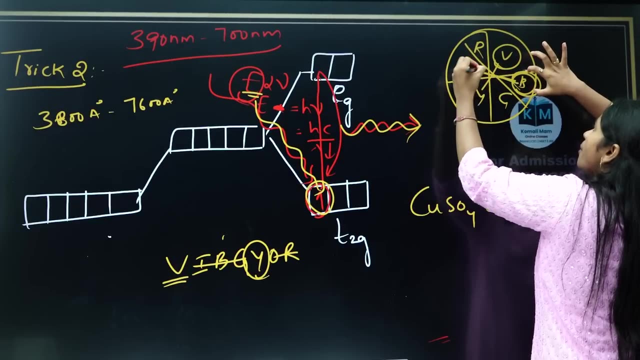 which means it is. it is appearing as a blue. blue color means complementary color. is a blue color, which means it is absorbing which color? they'll ask you question very easy: it is appearing blue color means it is absorbing which color. students tell me what is the complementary color: orange color. 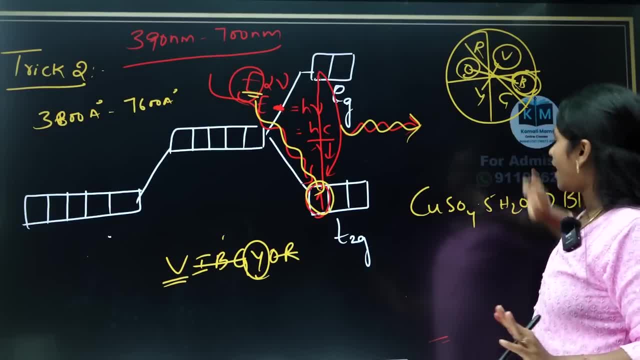 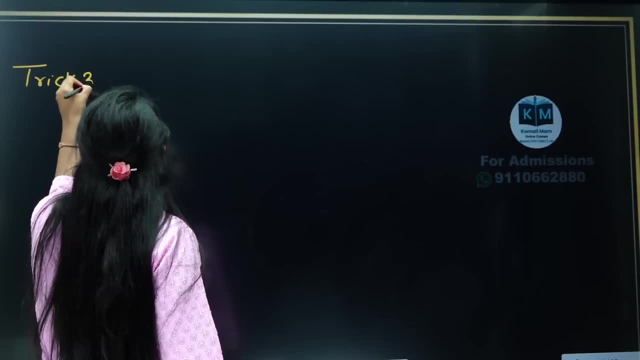 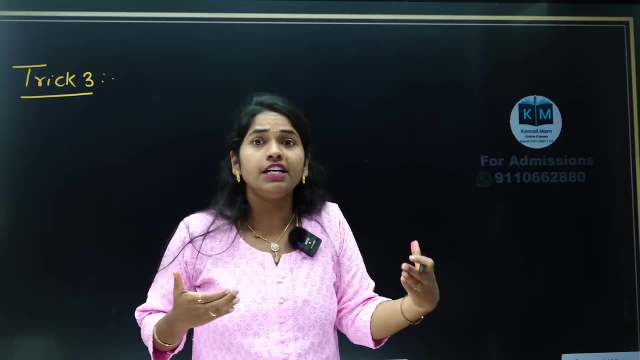 is it clear. so in this way you have to find the complementary color and trick number three is here. you should remember spectrochemical series. i will so much big spectrochemical series will be there. many different ligands, combination will be there. but in this session i am going to cover 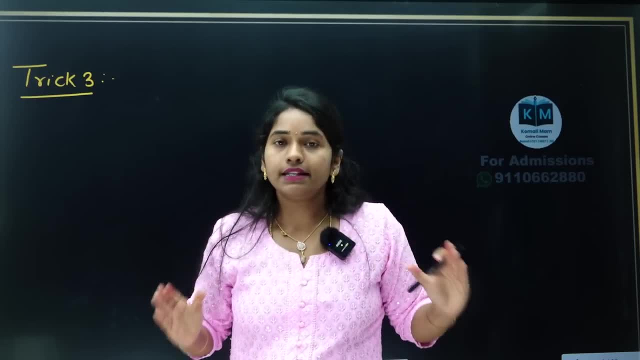 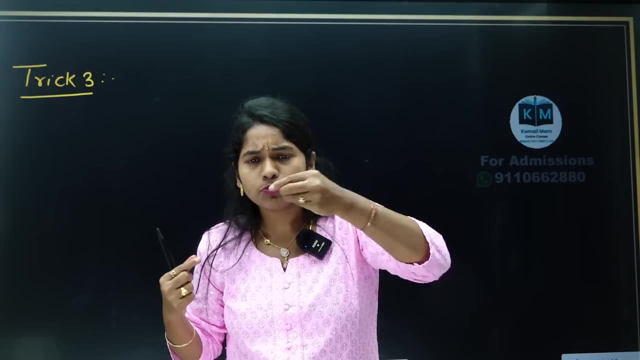 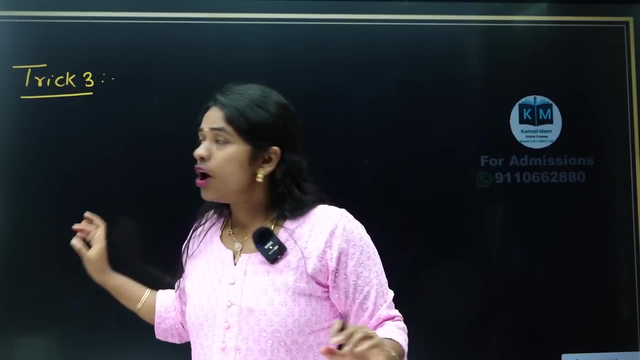 ncrt spectrochemical series. if you remember ncrt spectrochemical series, you solve questions if any important ligand which comes most times means you introduce it. otherwise, most of the cases, you solve the following questions: this spectrochemical series is enough. What is this spectrochemical series? Let us see. 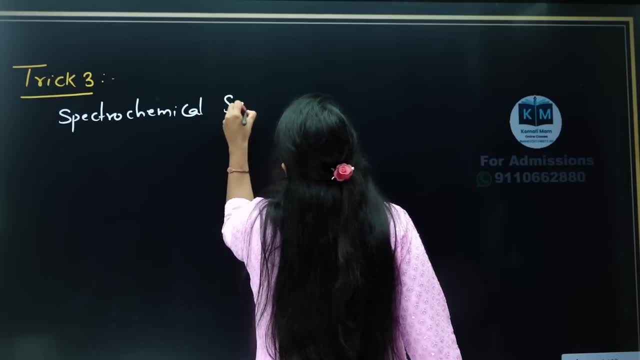 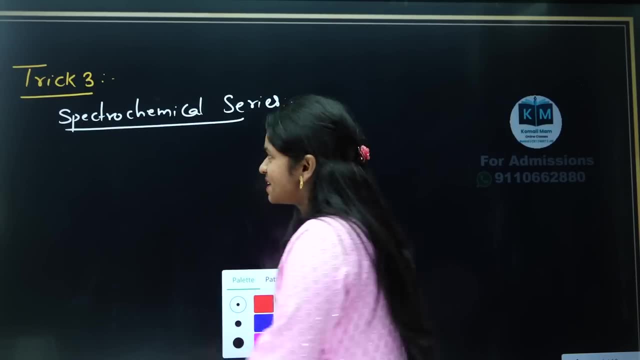 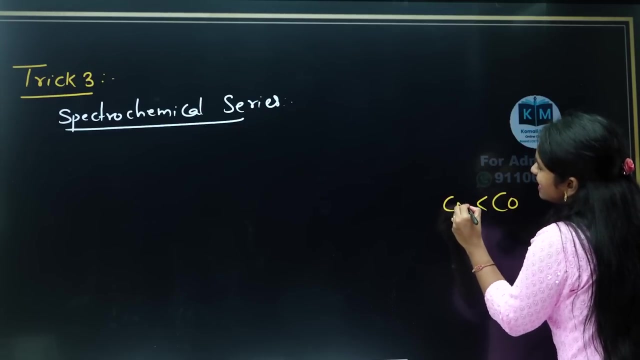 Spectrochemical series. If you are comfortable with my speed, you can keep 2x speed and you can watch it Better. if you write also, it is very good. Now let us say C-O, C-N minus E-N. 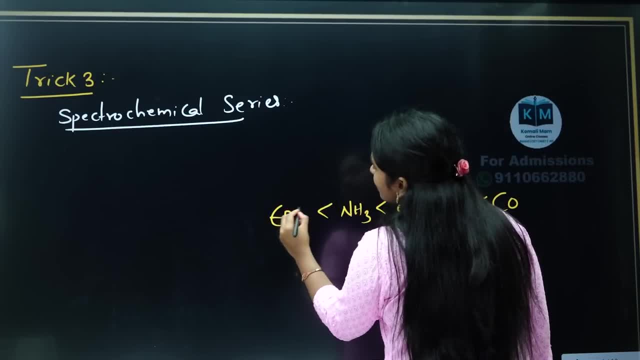 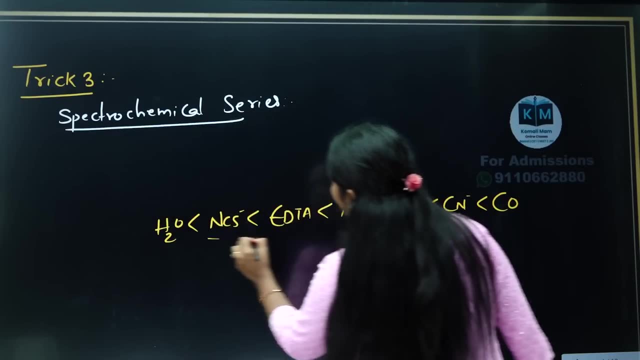 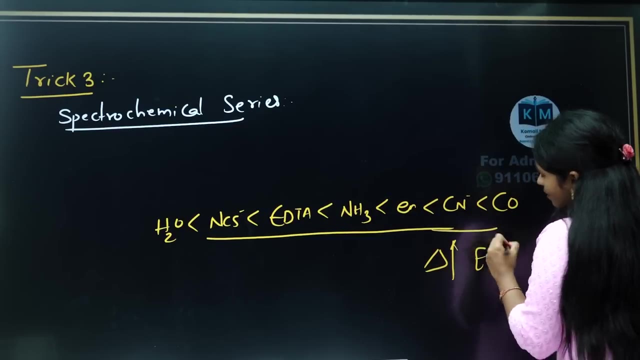 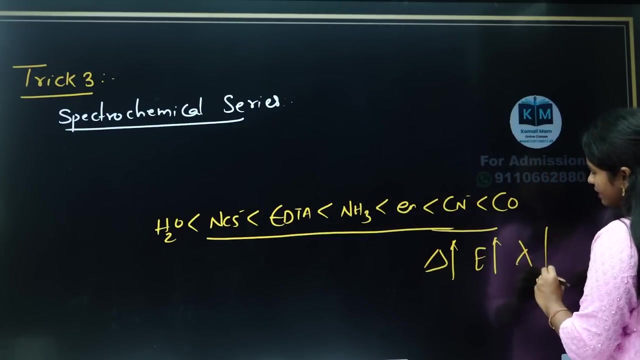 ammonia, E-D-T-A, N-C-S, minus here water molecule, all before whatever there before water. all are strong filigons. more energy, more splitting, more splitting will be in the present Presence of strong filigons. more splitting, more energy then less wavelength Now before water. 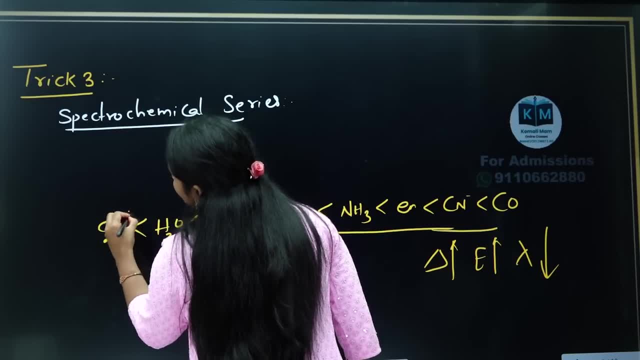 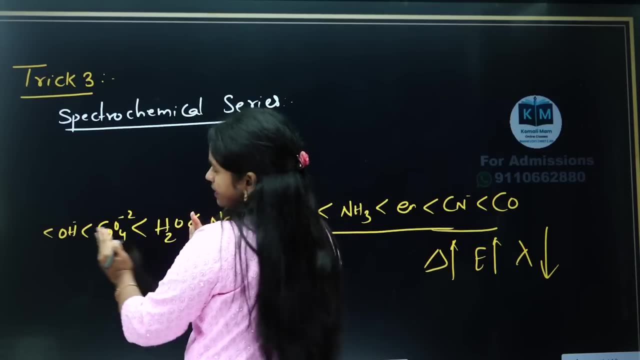 are weak filigons: C2O4 minus 2, OH minus. see how I am writing these are: oxygen is a ligand. oxygen is a ligand: see 3 sequence: oxygen ligand, next fluorine next. I am giving some gap. 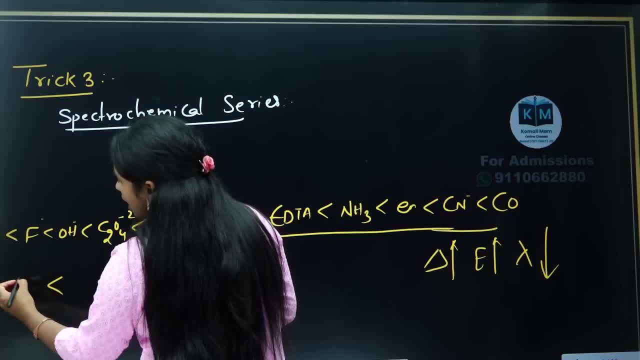 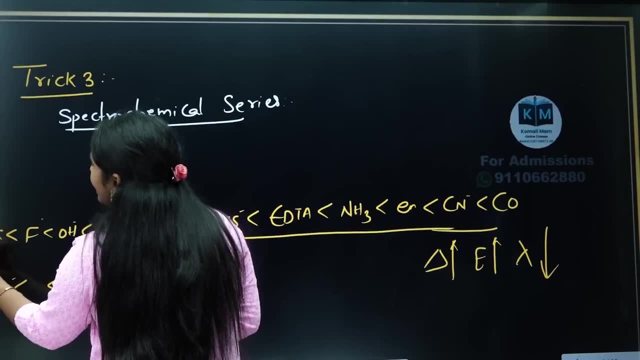 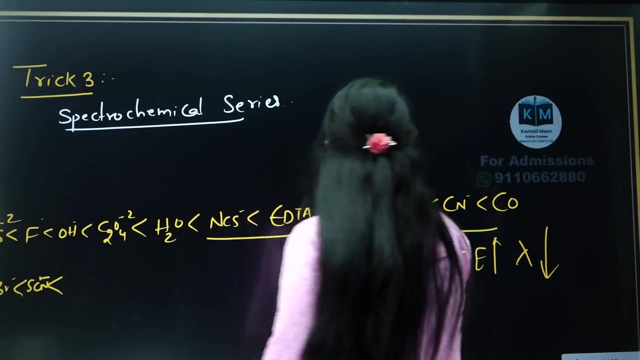 I am going to write chlorine. next continuation, I am going to give one gap and bromine iodine. bromine iodine: here I will write S minus 2, here I will write S-C-N minus, see starting N-C-S minus. 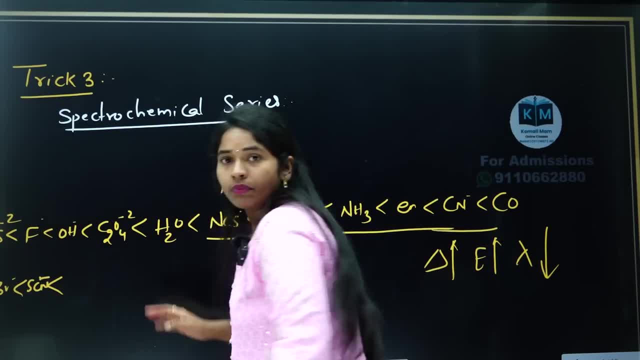 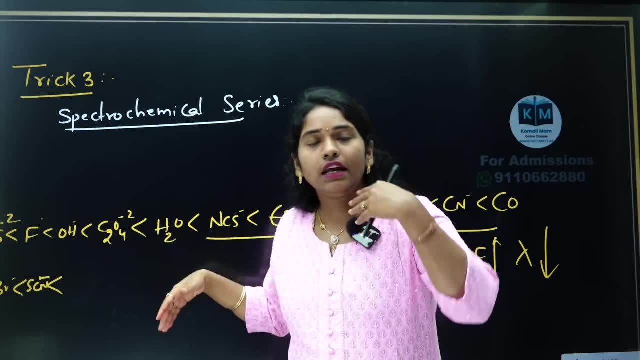 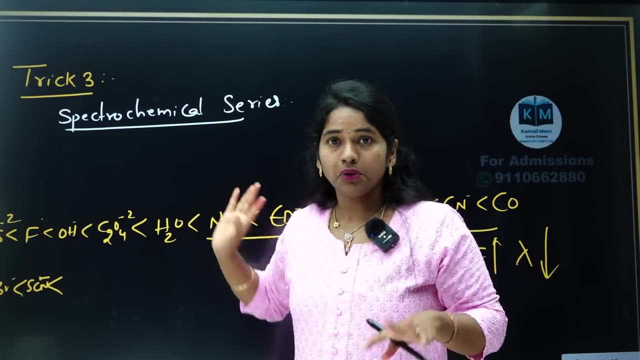 came here here, S-C-N minus, understand clear Spectrochemical series. you should have an idea this. you should remember any mnemonics you will keep or any memory techniques you keep. this order you remember, suppose, ma'am, I can't. 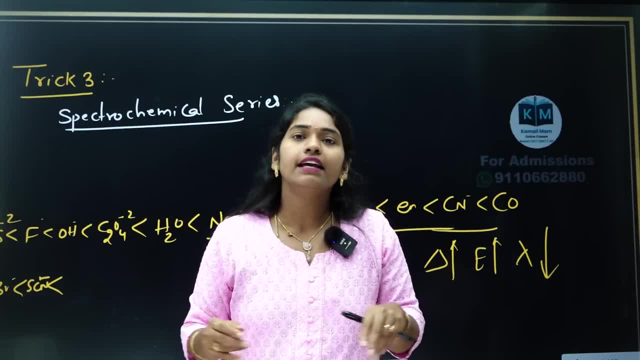 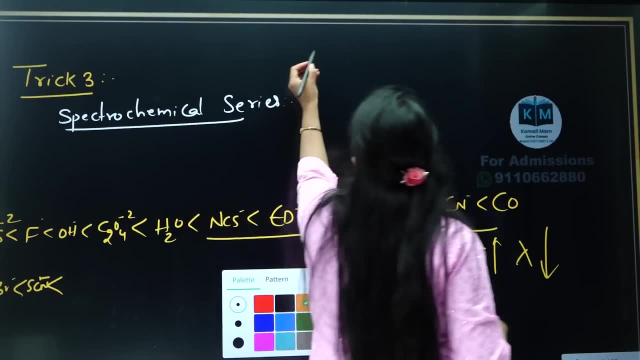 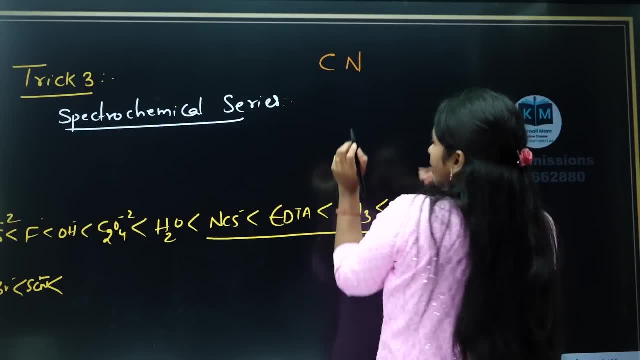 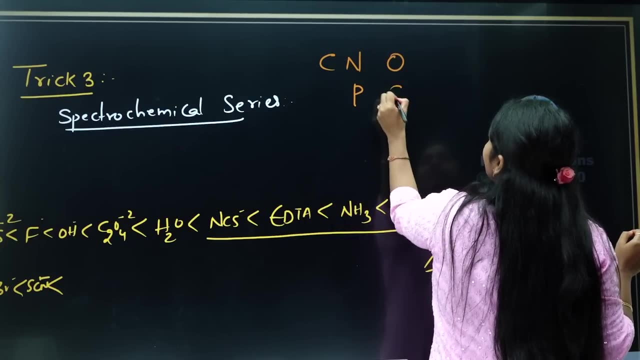 carbon nitrogen. I am writing periodic table: carbon nitrogen next to nitrogen phosphorus. this is oxygen, right. sulfur here, all halogens, fluorine, chlorine, bromine, iodine, like that. what I want to tell? 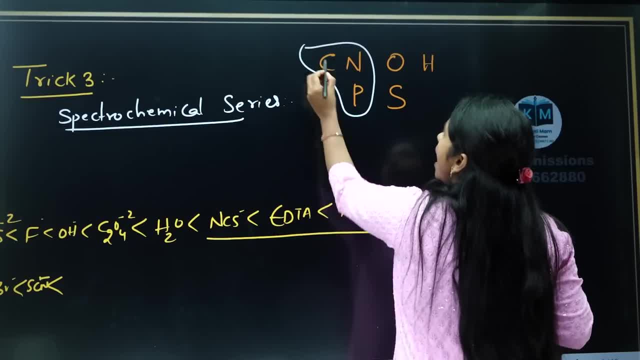 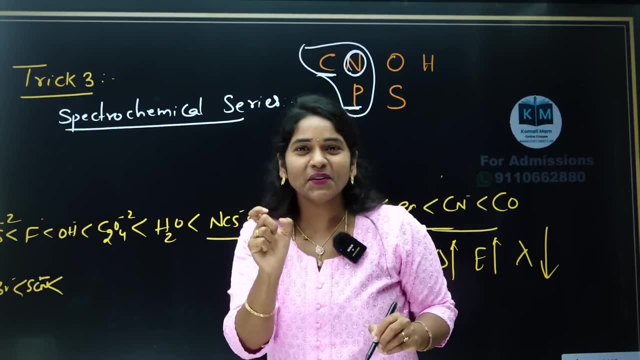 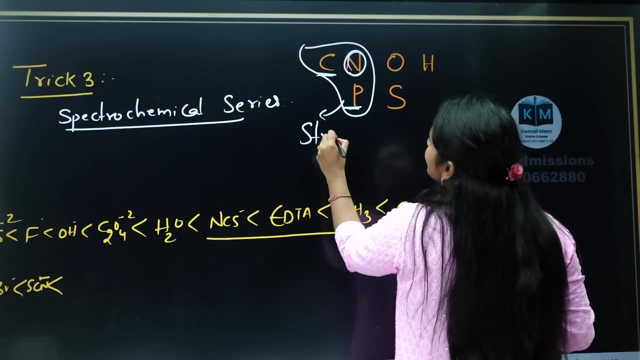 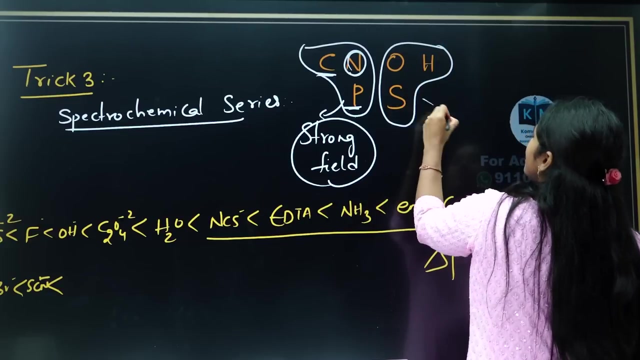 what I want to tell you is: these three are carbon nitrogen, phosphorus. see, say no to chemistry and physics, say no to chemistry and physics. so these are strong. actually, can't say no to chemistry and physics. these are strong filigons, strong filigons and see hostile. hostile like H-O-S halogens. 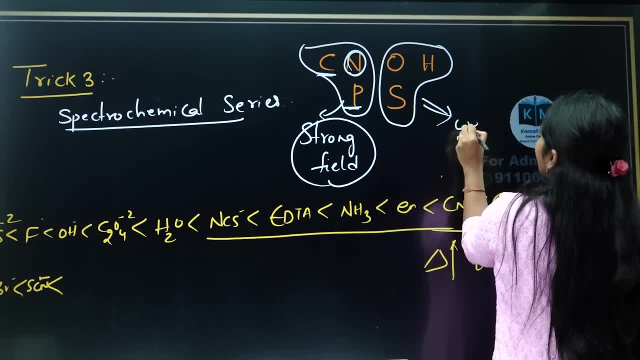 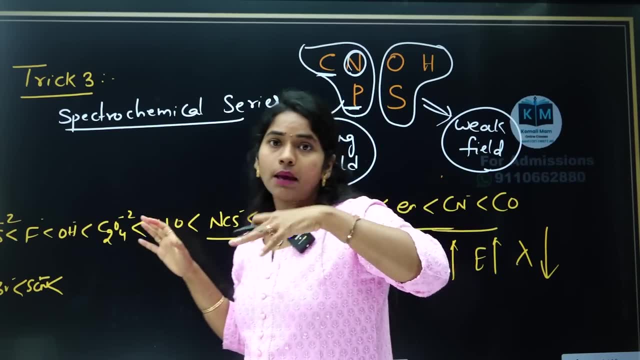 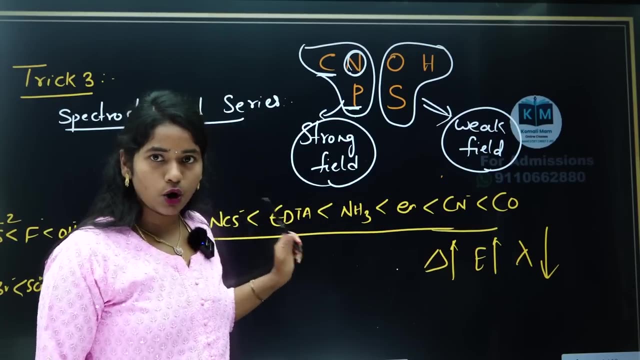 oxygen sulfur. these are weak, weak filigons, weak filigons. but this will help you to solve direct- I mean ligand based- questions. if comparison wise questions means this is, must, you should remember this trend. okay, and now trick. 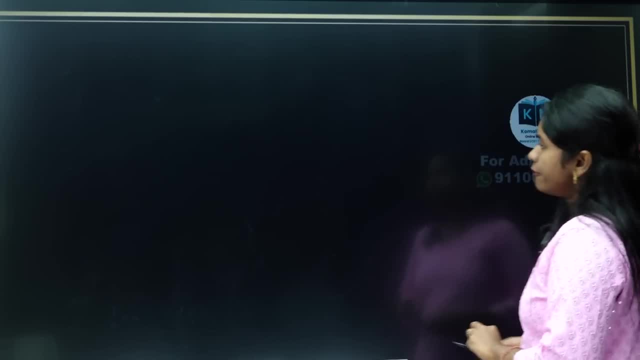 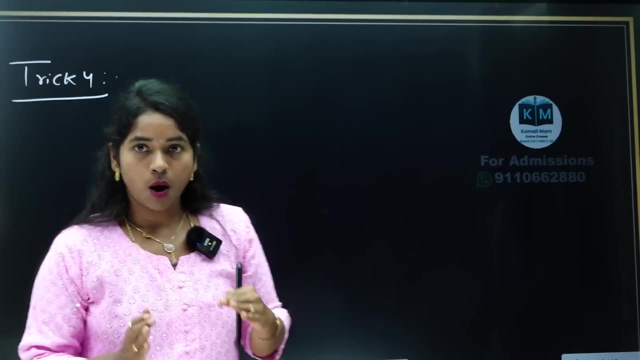 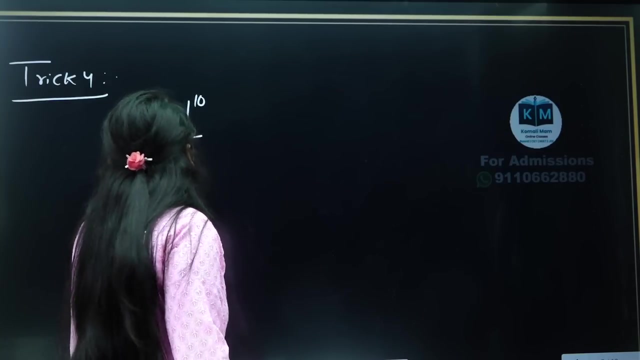 number five. trick number four. sorry, trick number four. here I want to tell you some colors, if any. coordination complex in that if metal, metal is having D0 or D10, I mean there is no D electrons- or completely filled, then it is usually. 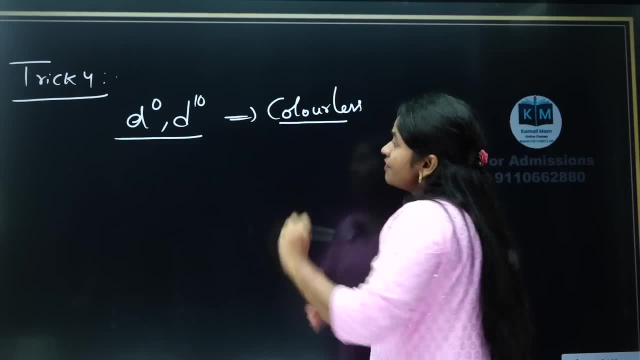 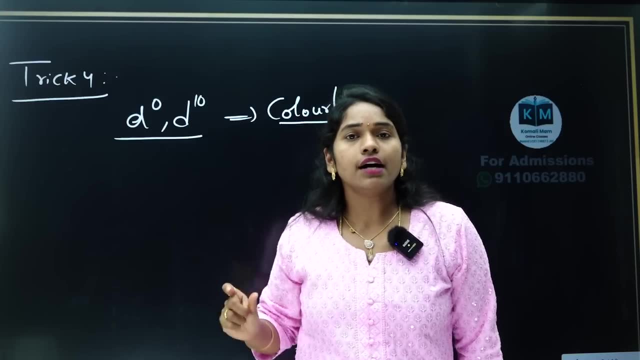 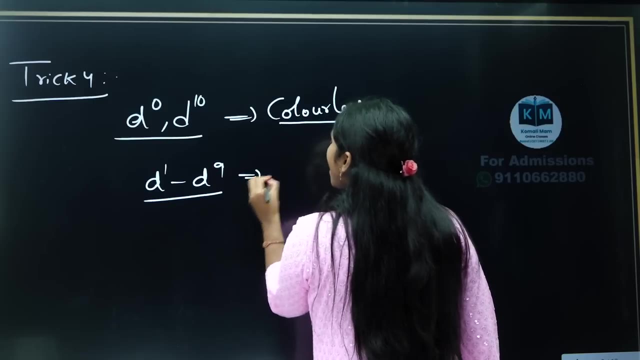 colorless. if it is colored, whether D0, D10, it should be colorless. if it is colored, then it is due to charge. transfer transition now: D1 to D9,, D1 to D9, these are colored, these are colored. 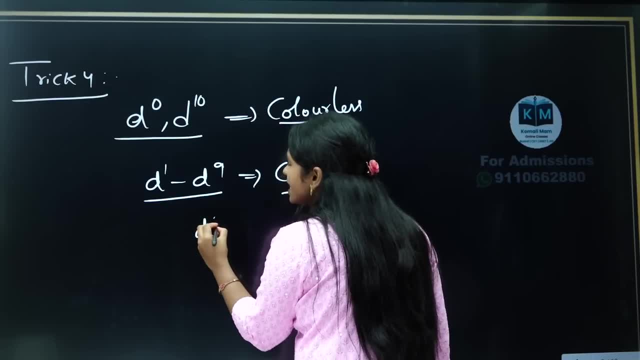 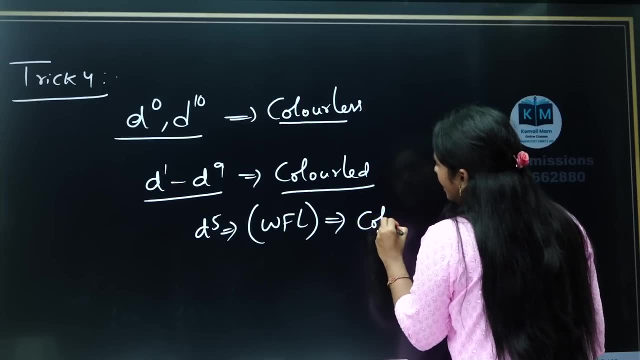 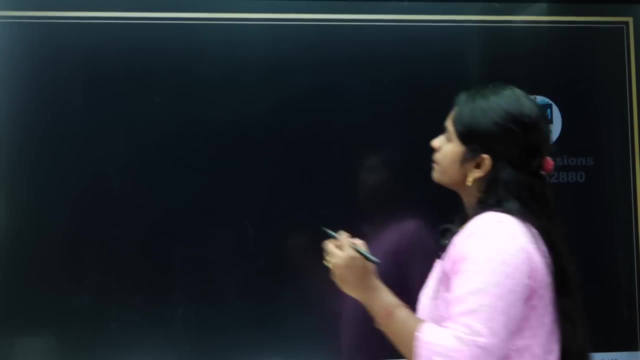 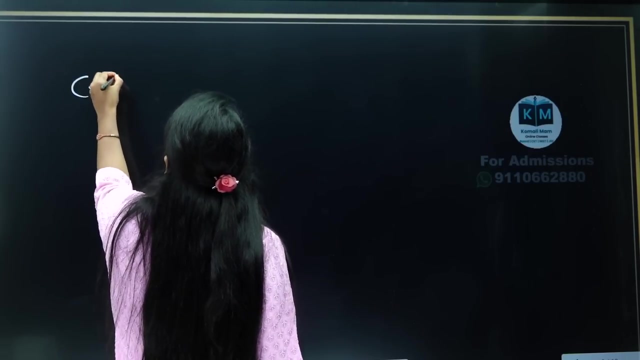 that's it. if you know, this is enough. if some cases, some cases, D5 combination with weak field ligand, it is colorless. it is colorless here I want to tell you some colors. just go through these colors once. take paper and pen and write this: it is very important. suppose chromium 2 plus and 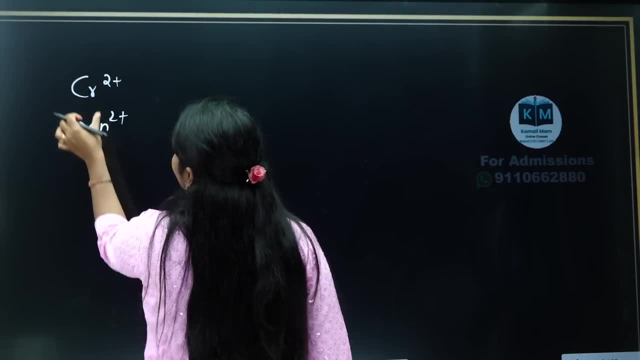 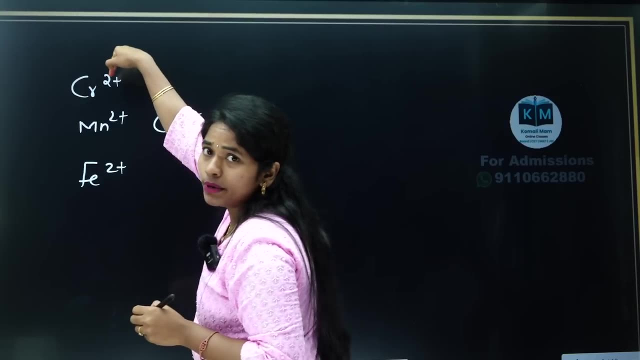 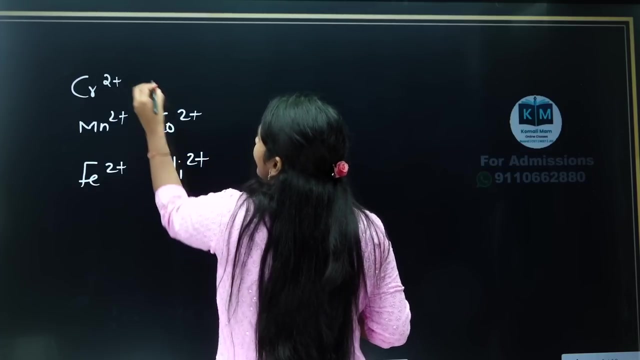 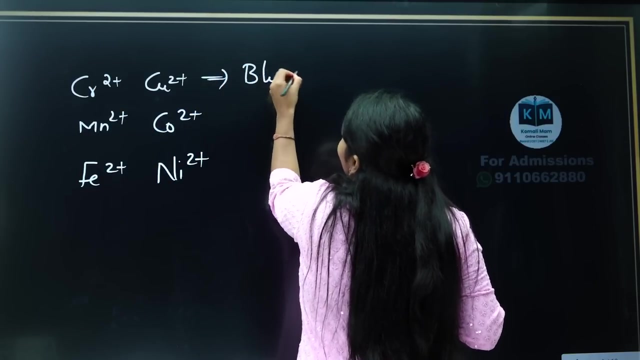 see how I am writing manganese 2 plus manganese iron, next time, starting from here, cobalt. see, i started from chromium cr2 plus manganese 2 plus iron 2 plus cobalt nickel. i'm writing here and here i'm writing copper. so this combination, you see, this is blue, this is a pink, light pink. okay, light, light pink. 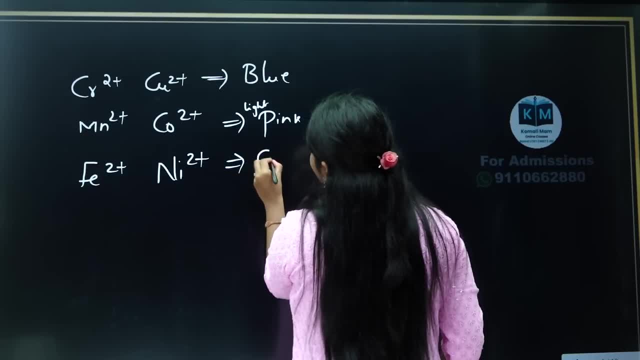 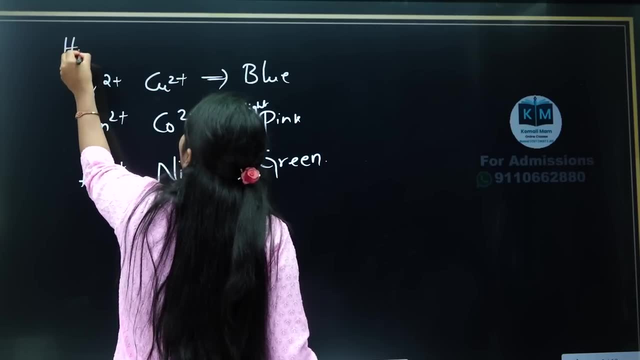 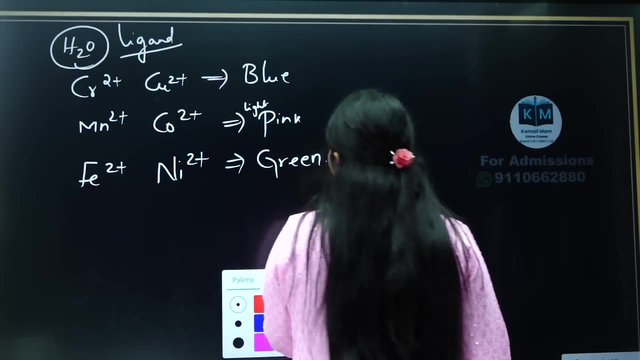 this is blue, pink and this is green, and what i want to tell you is this is the mostly with water. this, these colors are with a water is a ligand. understanding following everybody this. this cases are when when water is a ligand. water is a ligand if you change the ligands color of. 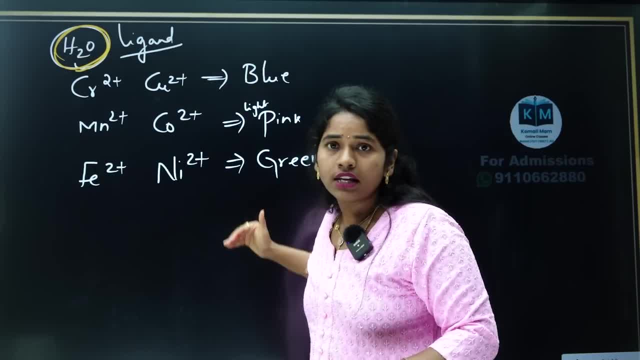 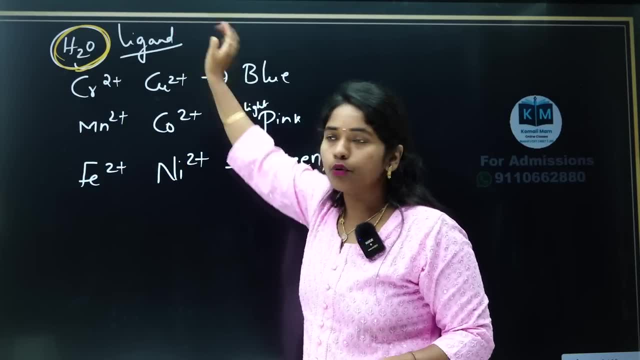 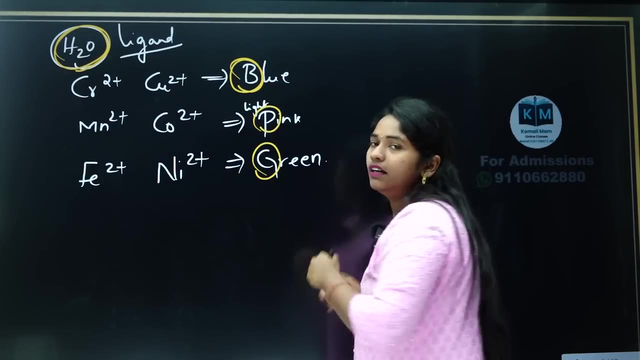 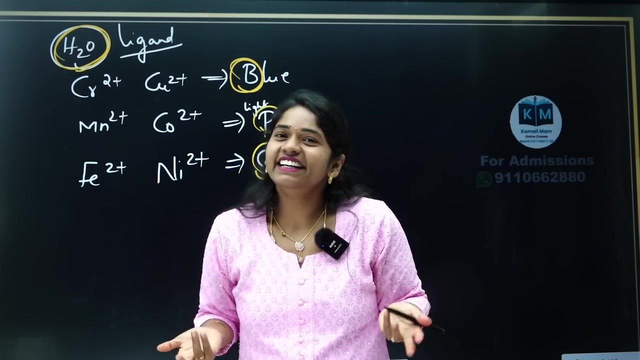 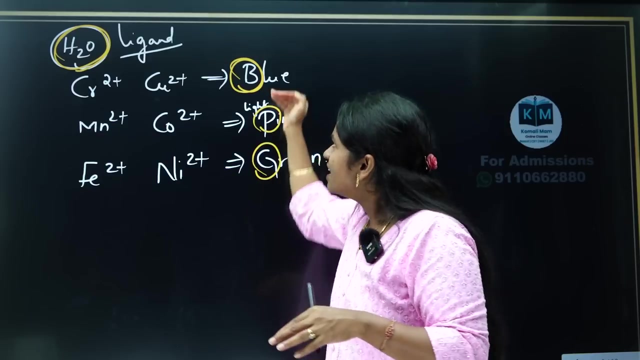 the complexes will change. are you following? this is when water is a ligand. see how to remember this. chromium, manganese, iron- i started here- cobalt, nickel and copper. i wrote here one blue, beautiful pink girl. beautiful pink girl. oh, beautiful pink girl. oh, nice na. haha. simply, i told beautiful pink girl. so this is easy to remember. okay, beautiful pink girl. 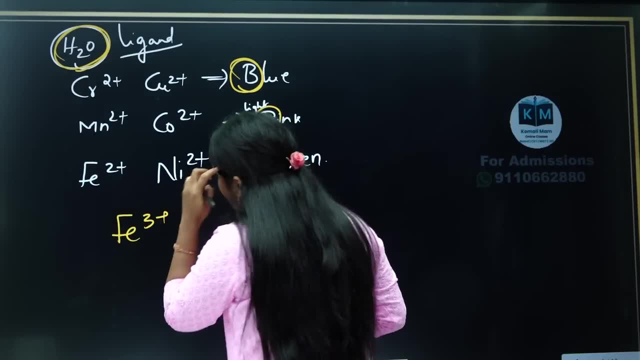 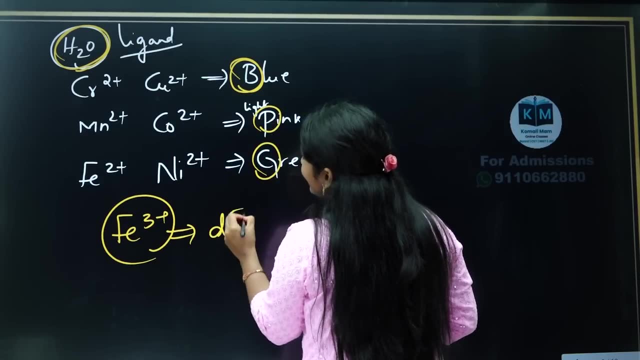 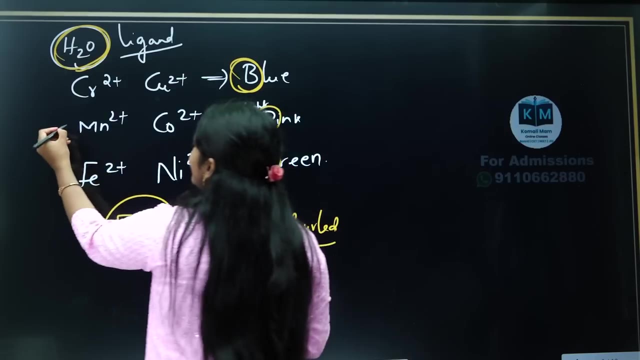 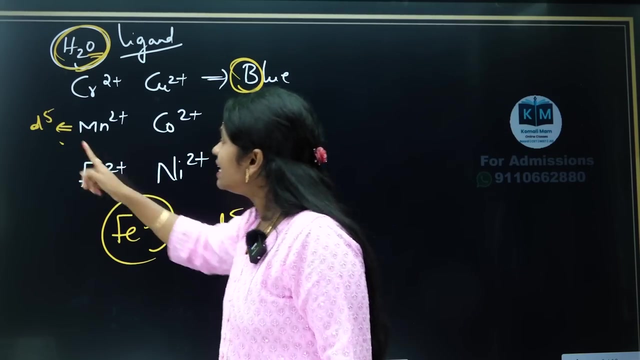 right now, f? e three plus. if f? e three plus, then what happens is this is actually d five, combination d five, but it is also colored. you no need to remember the colors. but here i want to tell you: manganese, also d five combination water in water oxygen is a weak field ligand, but manganese and f? e three plus. 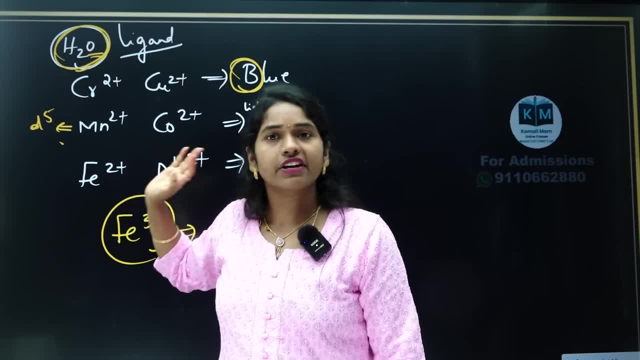 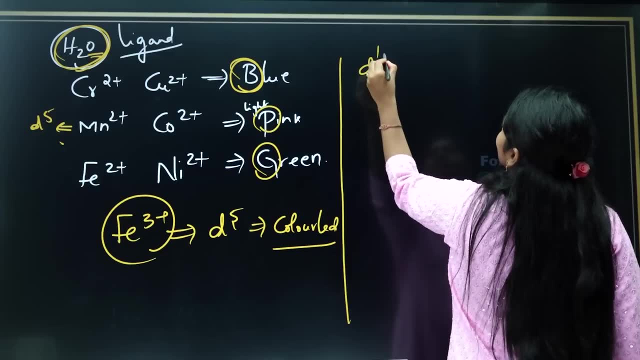 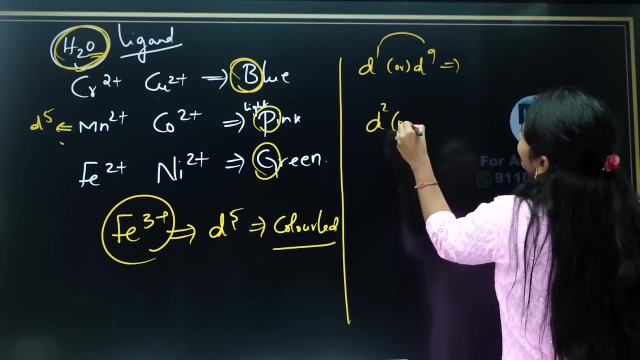 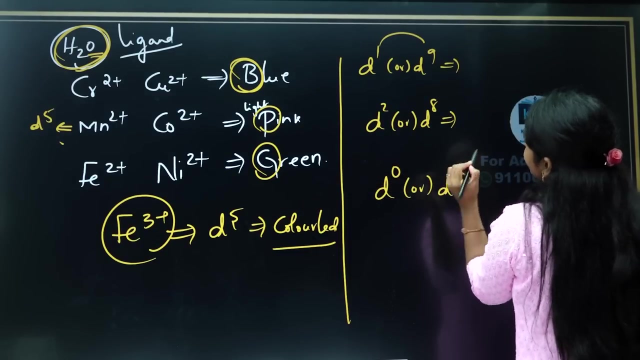 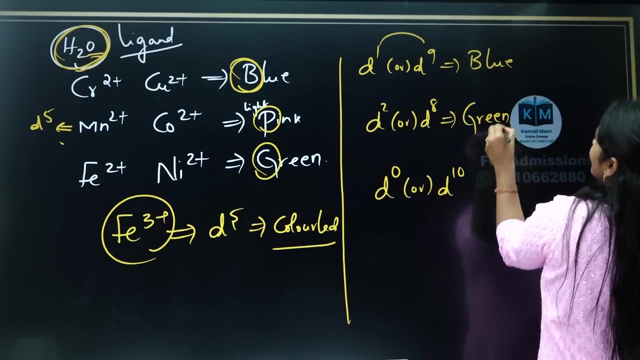 these are colored even though water is a weak field ligand. this is the energy line. so here you have to doubt you or you have tank in your mind and come into that. any one: d nine nine plus 110, combination d V or d eight and D d zero or deep in these combinations e carefully, this is blue color. 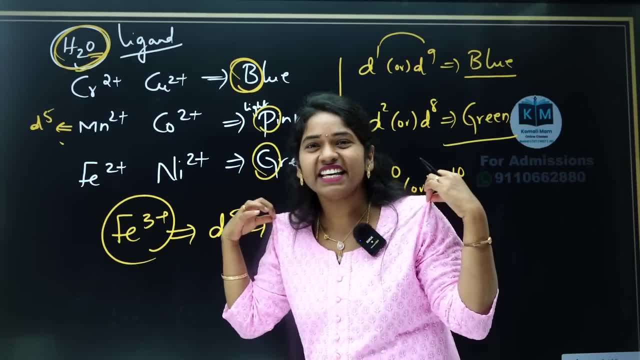 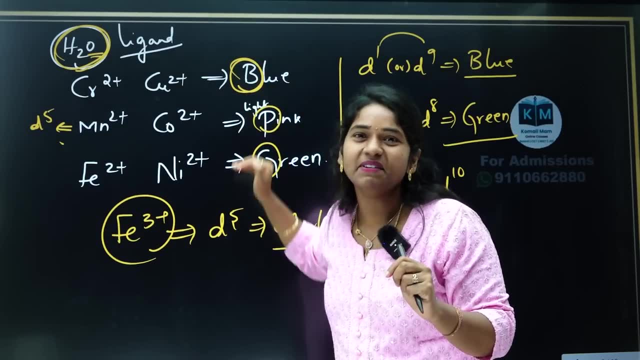 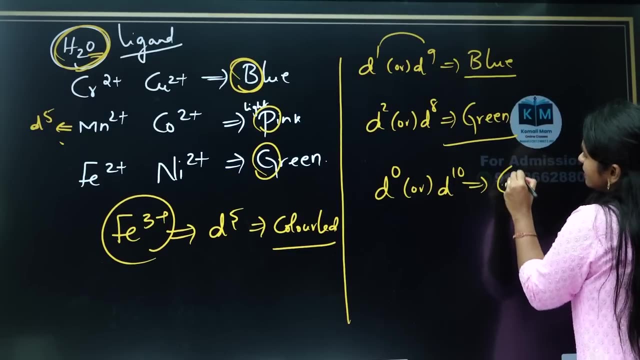 and this is green color. beautiful girl, beautiful girl. this is beautiful, get it. so this is beautiful girl, beautiful, much beautiful الي��. this is beautiful pink girl, so this is beautiful pink girl. ma'am, you are girl, no, no. so simply for remembering, I am telling you this. and this is d0 or d10. it is colorless, there is no d electrons. 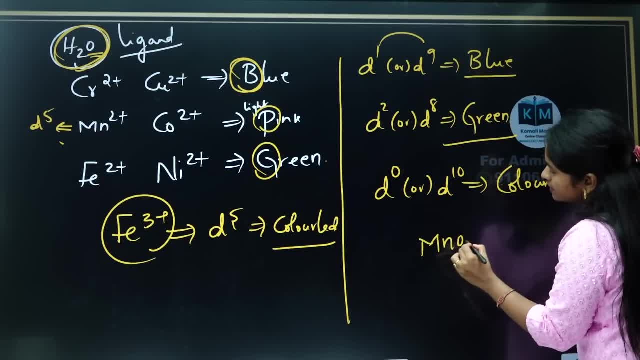 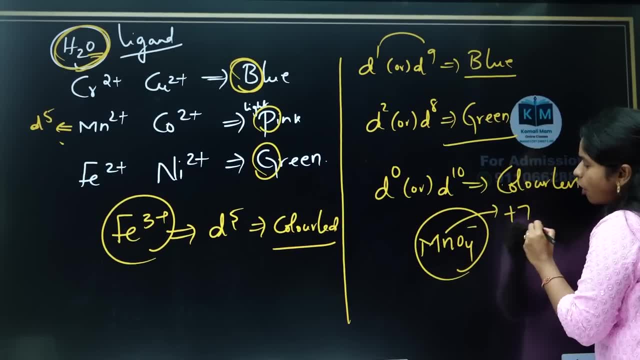 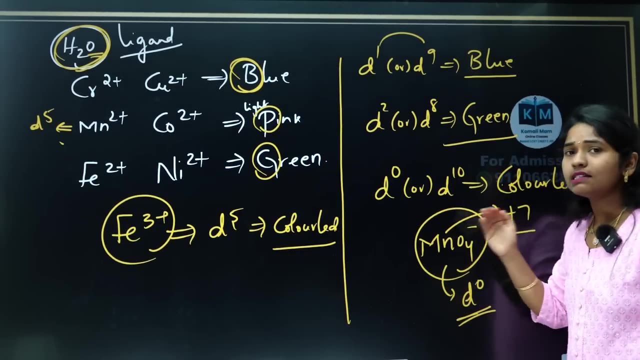 but if you see MnO4 minus, this is, you know, purple color. you know this is in this. manganese is plus seven combination plus seven oxidation state. plus seven means d0. there is no d electrons. but why it is colored? because charge transfer transition. in this session I am covering only 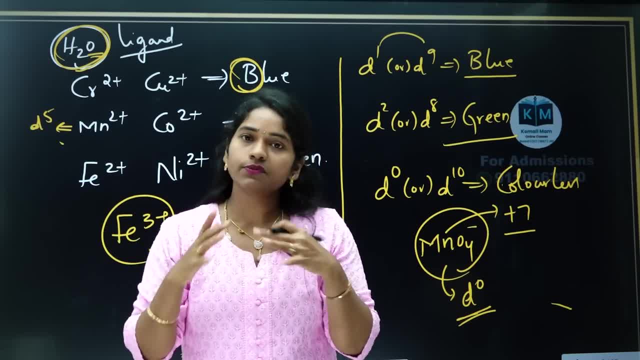 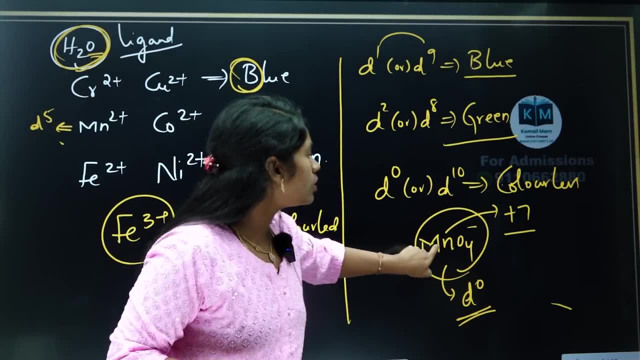 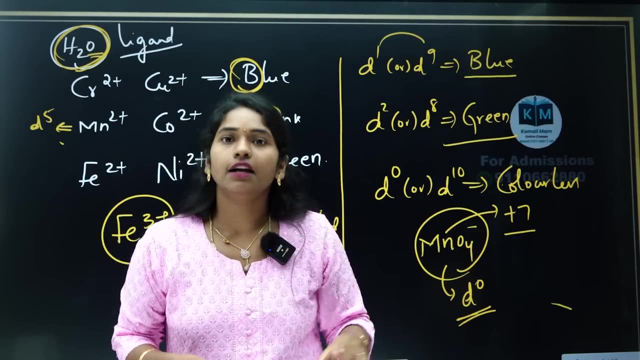 dd transition means, sir, sir, if they, it is very easy, you can easily identify. if you cover this, you can solve question very easily on charge transfer transition, because if there is no d electrons or d10- if still they are asking that why it is colored means you can directly take it it is due to charge transfer transition. now let us solve some. 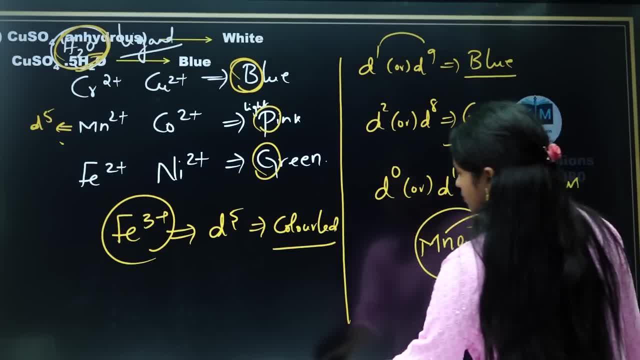 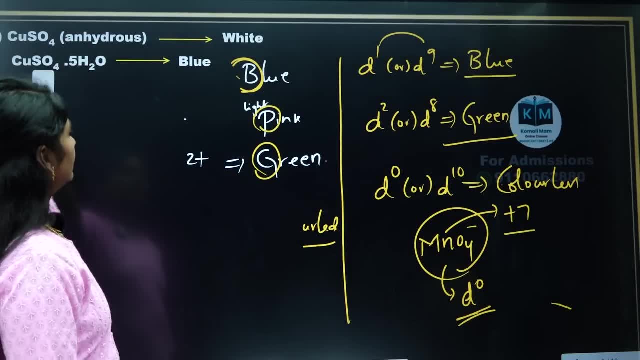 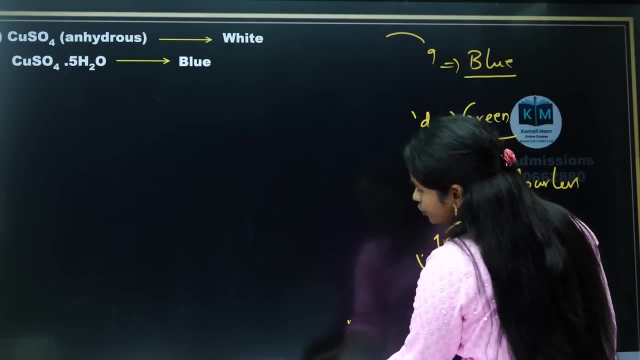 questions. let us solve some questions. see this question here. copper sulfate is white color and copper sulfate with water is blue color. what is the reason they were asking us? what is that, students? copper sulfate is blue color. only copper sulfate is blue color. only copper sulfate is blue. 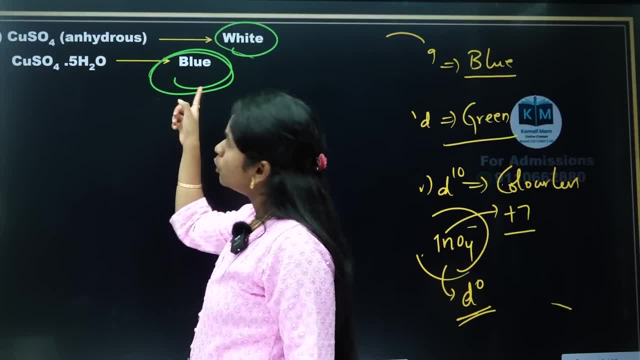 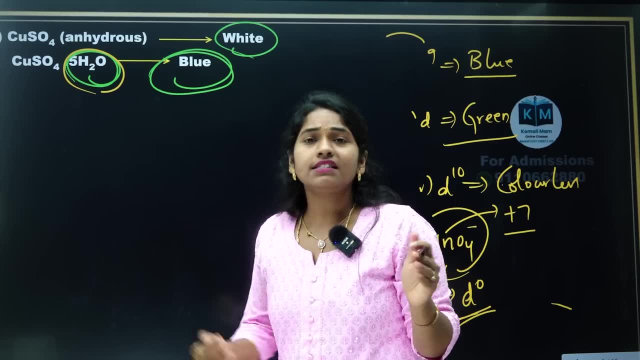 if it is white color, no color, it is blue colored because here there are 2 ministers: 2, 92, 3, 13, 14, 15, 16, 17, 18, 30, 40, 41, 42, 43, 44, 44, 45. 47, 48, 47, 48, 49, 51, 52, 53, 54, 52, 53, 54, 56, 56, 67, 68, 69, 69, 70, 70, 61, 61, 69, 72, 72, 73. 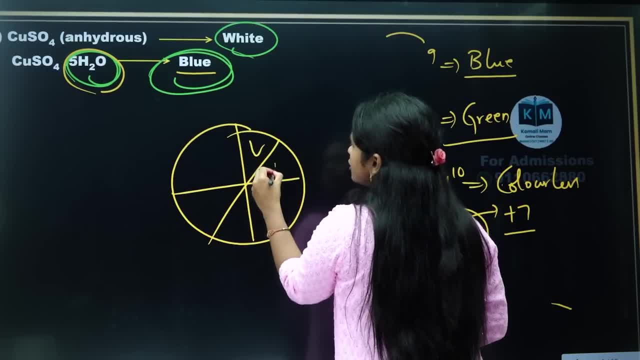 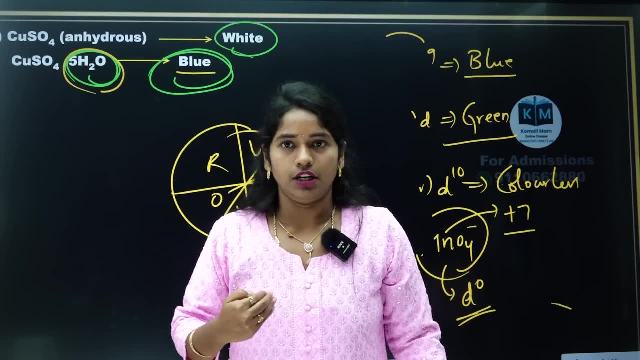 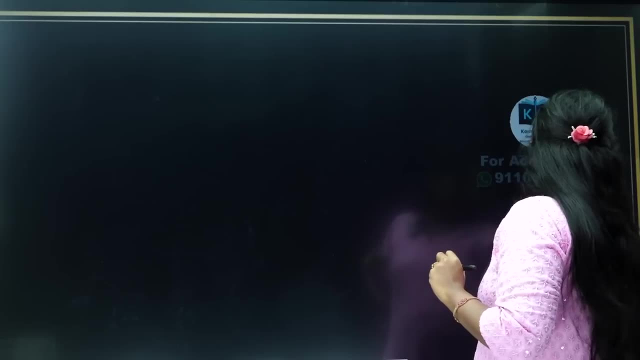 72, 73, 74, 74, 75, 75, 74, 69, 70, 79, 70. blue color means it is absorbed orange color, I mean appearing as a blue means it absorbed orange color. Then see the next question. They were telling that FeSO4 is anhydrous, is white color. 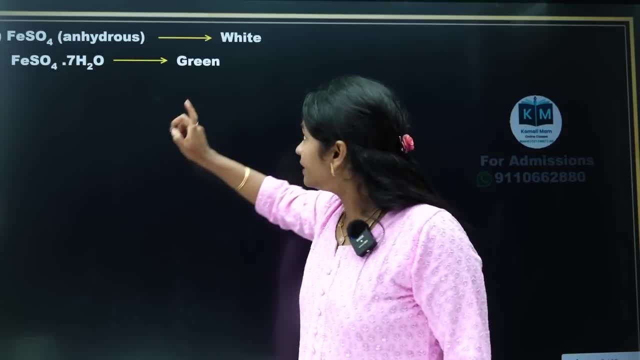 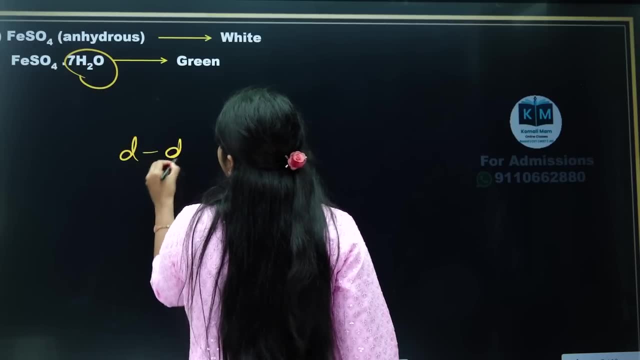 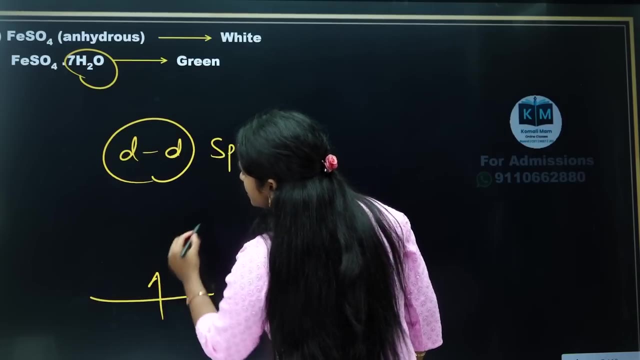 but when water molecules you added, then it turns green color. Can you tell me what is the reason? Because of ligands. Ligands, D-D transition is happening, D-D splitting is happening, D-D splitting, Whatever the here electron is present when radiations with a certain energy, which is 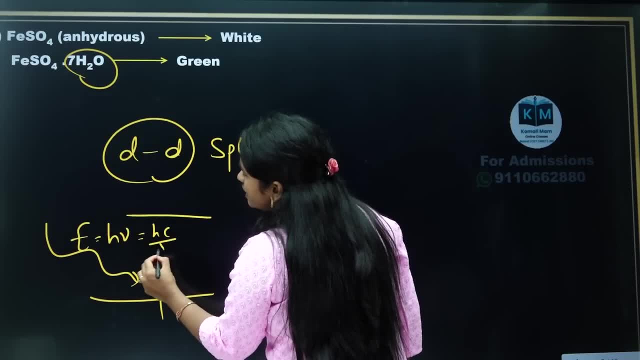 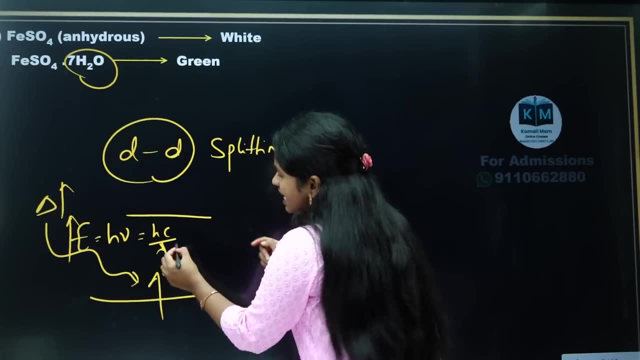 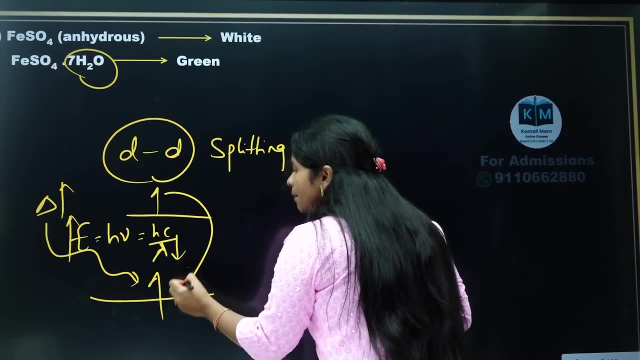 directly proportional to frequency, which is inversely proportional to wavelength: More energy, strong field ligand, more splitting, more energy, less wavelength. It absorbed, It goes to this electron, It goes to excited state. When it is coming back, it emits the radiation. This emitted radiation is: 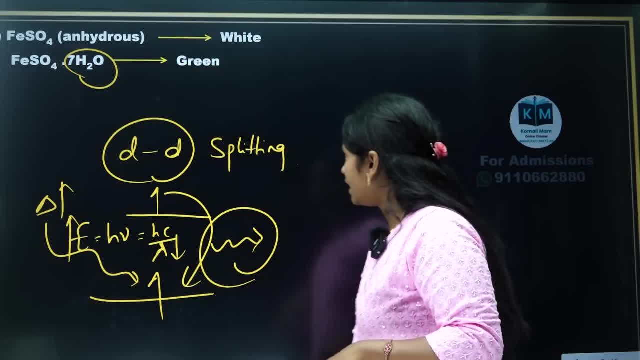 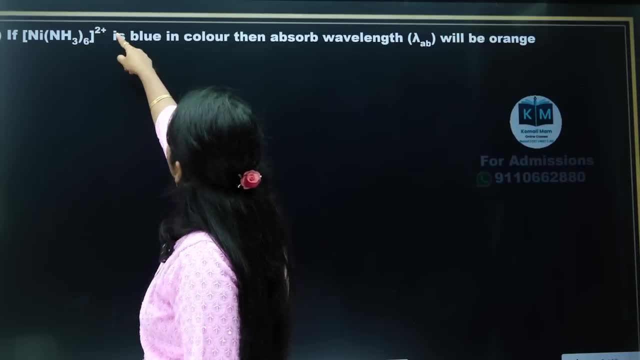 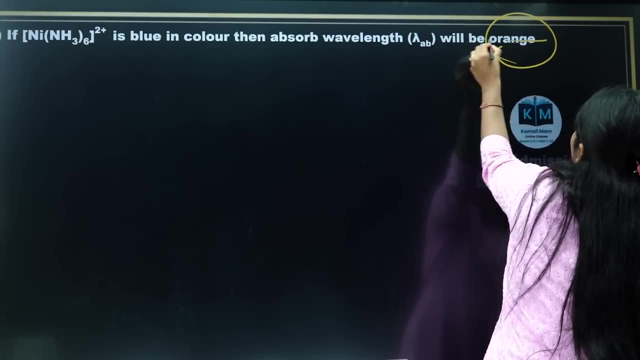 a complementary color which I discussed with you, Clear everybody. See the next question: How easily you can solve these questions. If NiNH362 plus is blue in color, the absorbed wavelength will be orange. Can you actually? this is blank. You should say which color it is Then. why tell me it is blue? 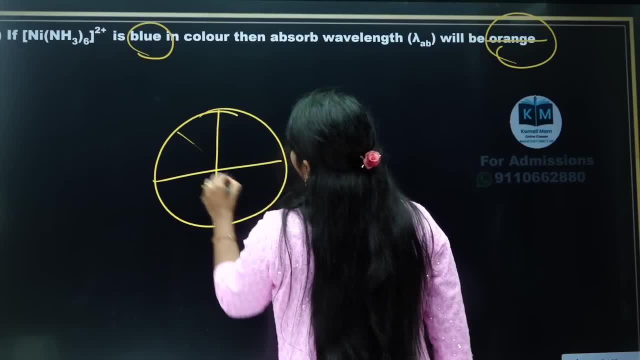 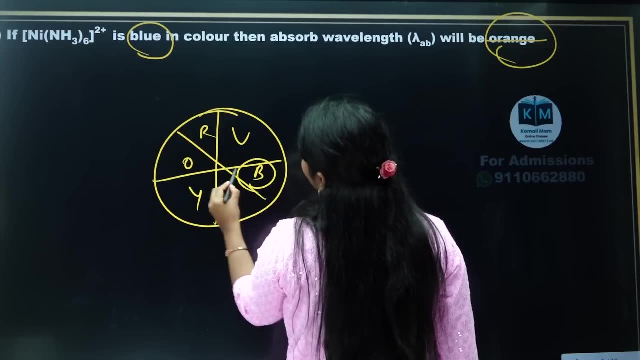 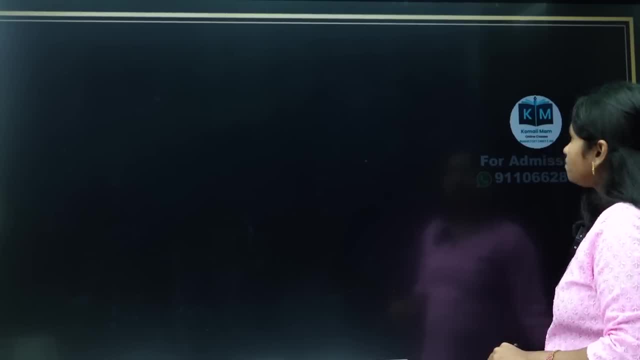 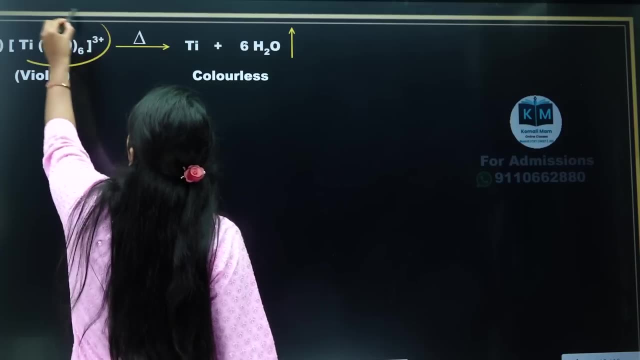 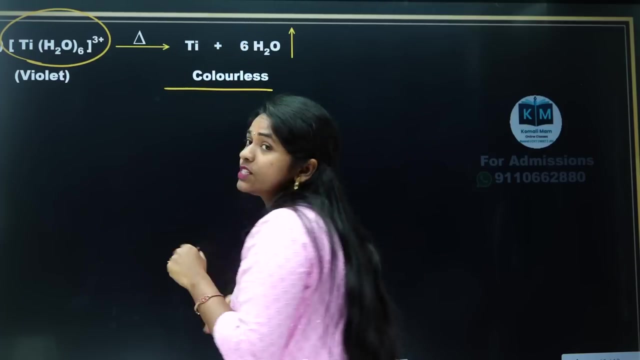 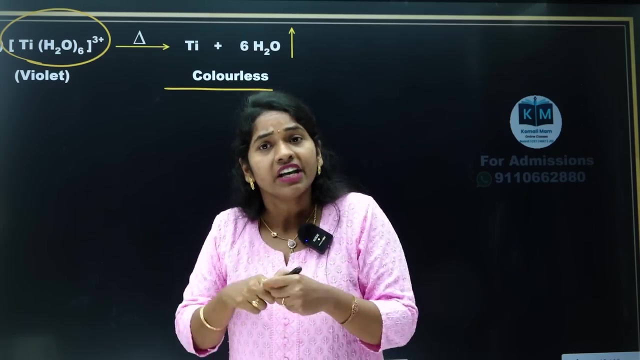 wavelength. Next, see the next question. everybody, If you see TiH2O6 3+, this is violet color. but this complex, upon heating it became colorless. Why? Because in this case ligands are there and you know, transition DD splitting happened and we got the color, but here there are no ligands, no color. 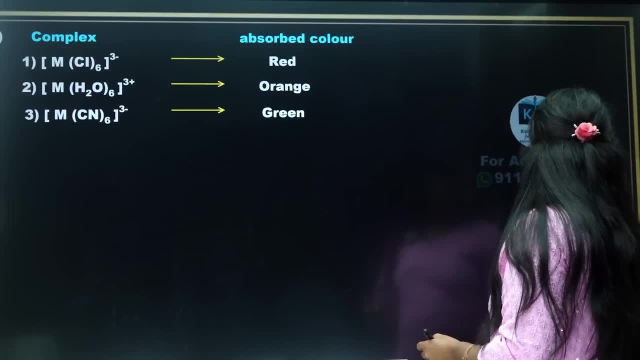 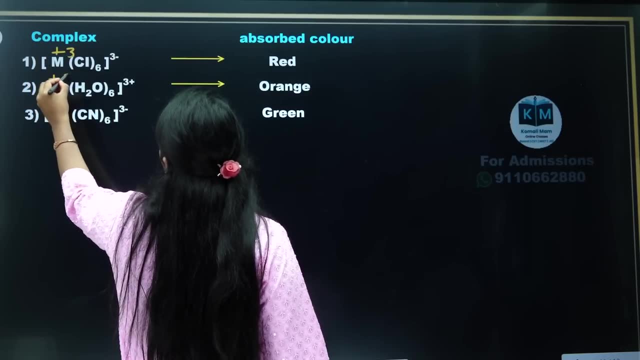 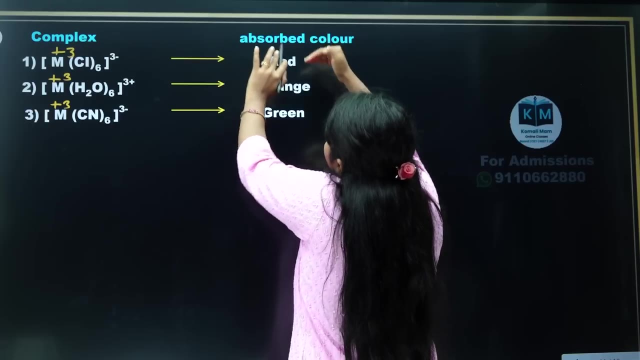 See the next question. MCl6 3- In this oxidation state of metal is plus 3, here plus 3, here plus 3.. I am not going to tell you how to find this oxidation state. I want to tell you. this is the absorbed color I want you. 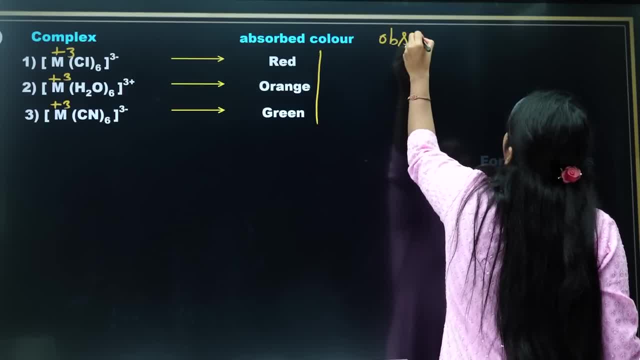 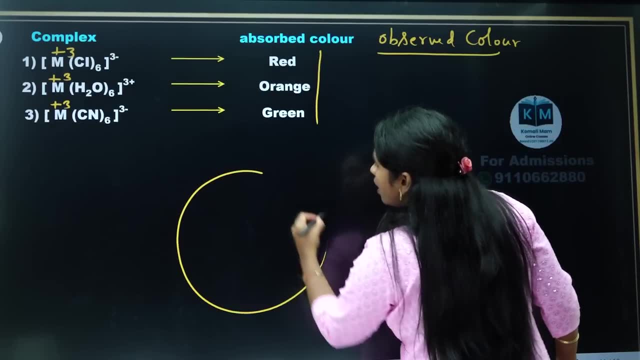 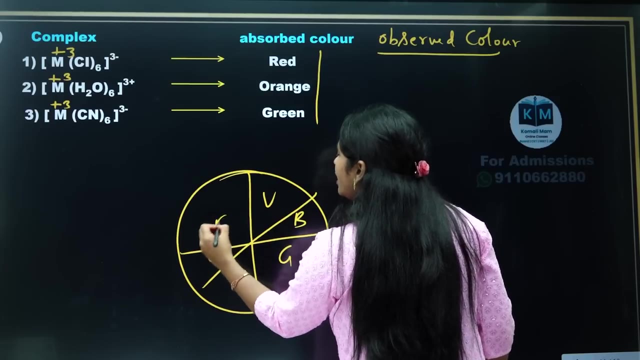 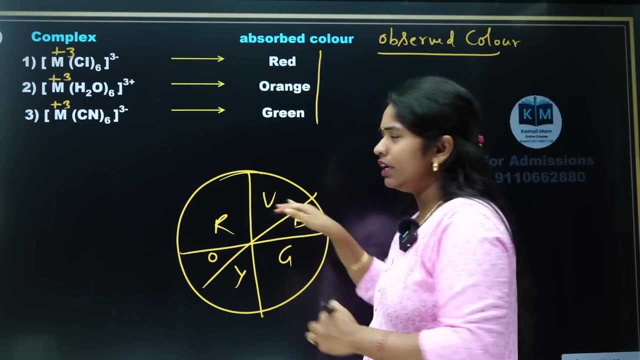 to find the observed color means. complementary color, Observed color. Can you tell me observed color? Draw the wheel. color wheel: VibGR. I am not telling you indigo here. If you want you can write indigo also, and most of the times it only come. Indigo is complementary to yellow Means if indigo. 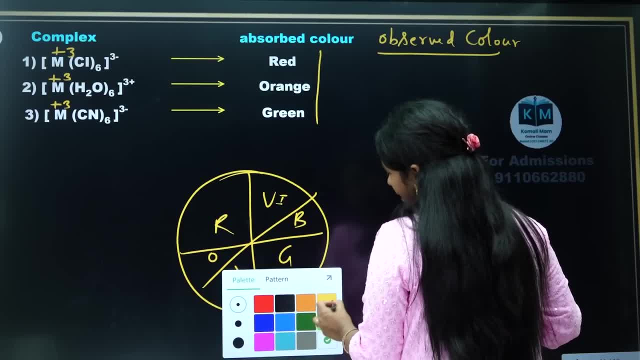 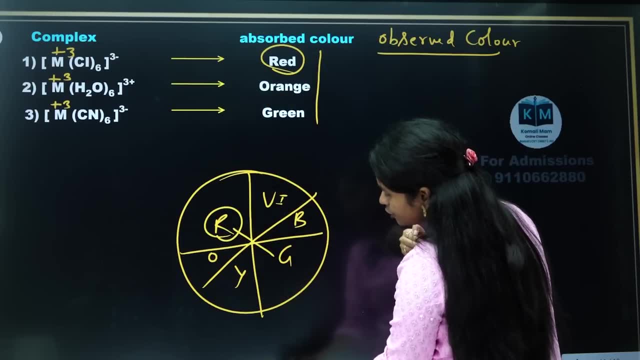 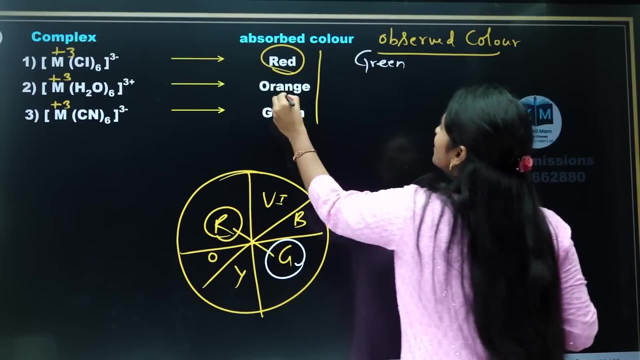 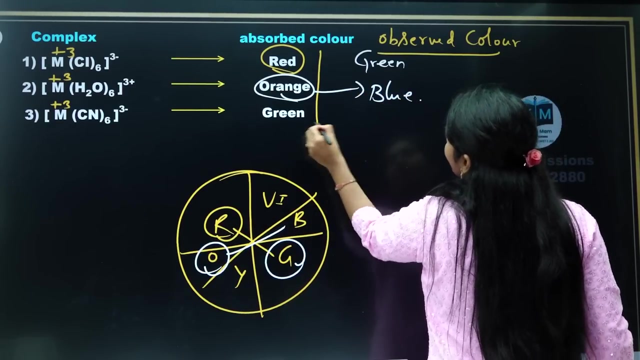 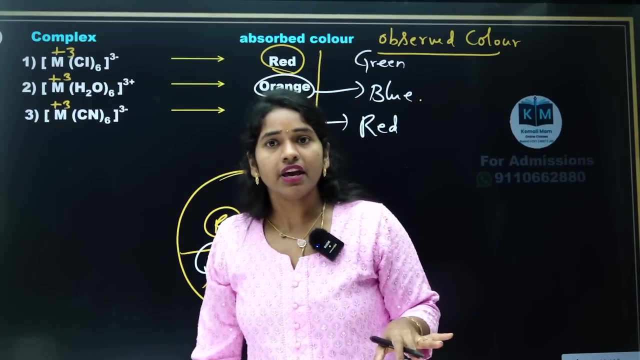 means yellow, only it is a tertiary color. That's why we don't mention usually Now, red color, absorbed color, red color: What is the complementary color? Students tell me What is the complementary color? Come on, say loudly: Green color, Green color, Very good. Orange: What is the complementary color to orange? Blue color is the complementary color, Very good. Green: What is the complementary color? Red color is the complementary color In such a way you have to solve it. Okay, Now see the next one. 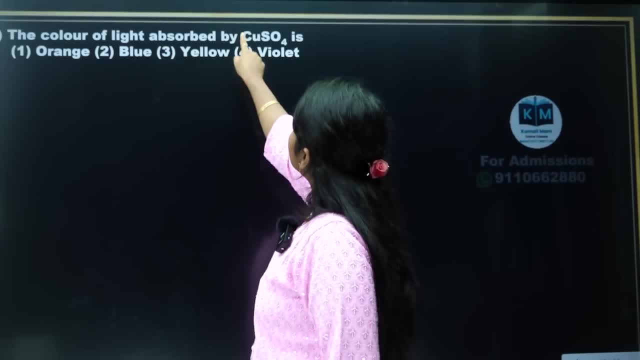 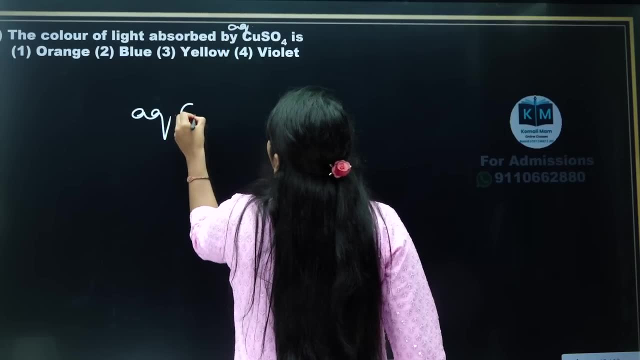 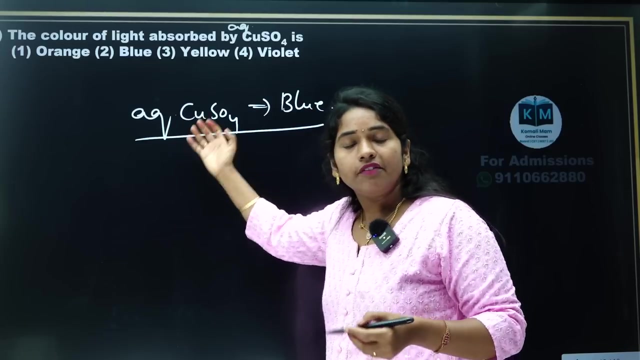 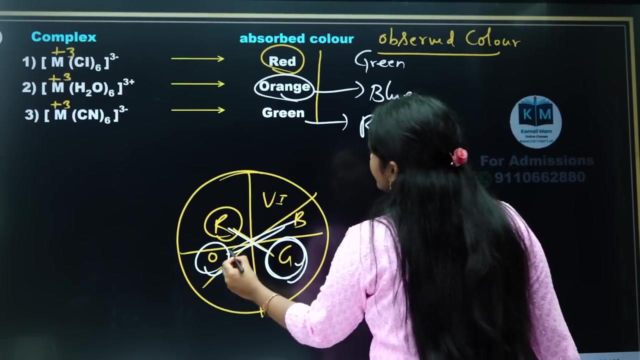 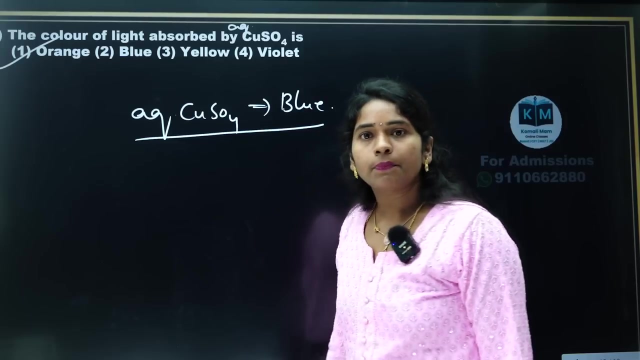 The color of the light absorbed by copper sulfate. Actually, aqueous copper sulfate, it is. Aqueous copper sulfate is blue color. Aqueous copper sulfate is- This is NCRT question- It is blue color. Aqueous copper sulfate is blue color. means which color it is absorbing. Just now I told you Blue color. complementary is orange color. So here your answer is what It is? orange color. option number one: Okay, Easy, See how easily you can solve the questions. 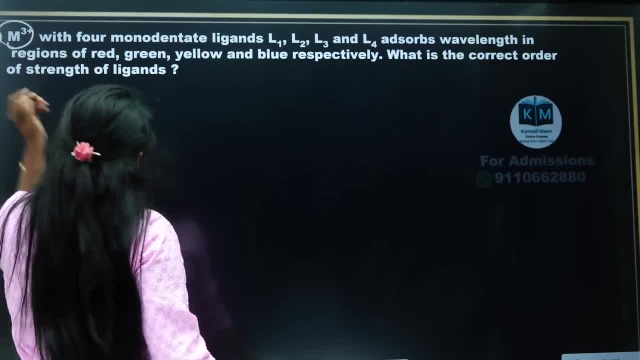 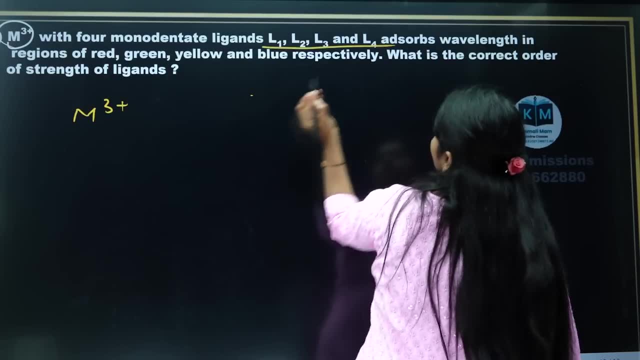 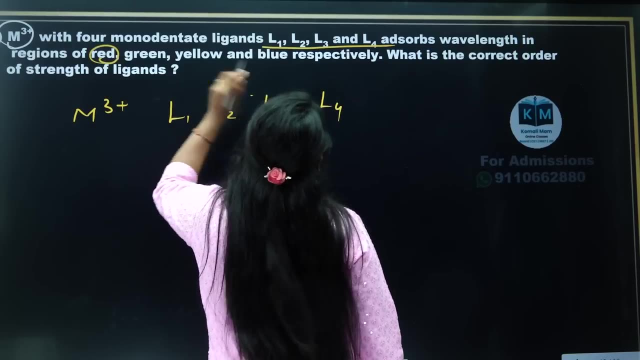 Next one, M3 plus. one metal is there. What is the metal students? M3 plus? M3 plus is the metal. It is having four ligands combination. What are those four ligands? L1, L2, L3, L4.. Now they were telling that different colors it absorbed, Like red color and yellow. 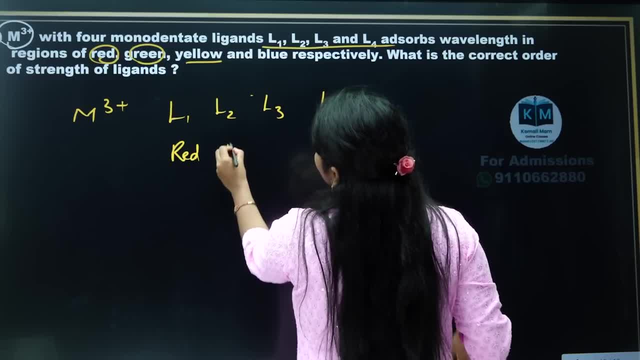 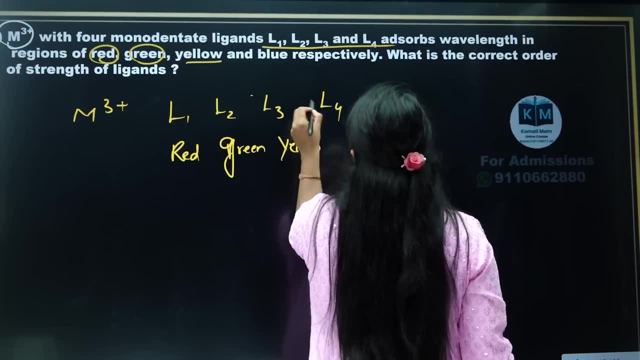 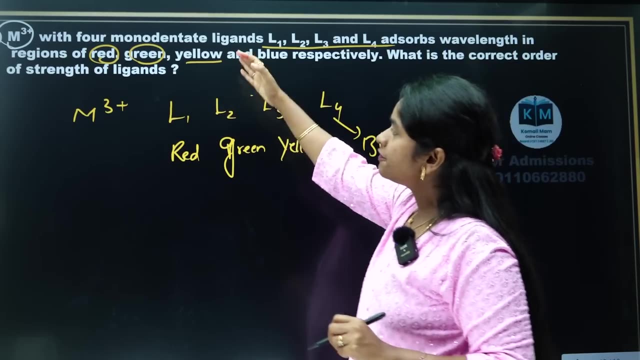 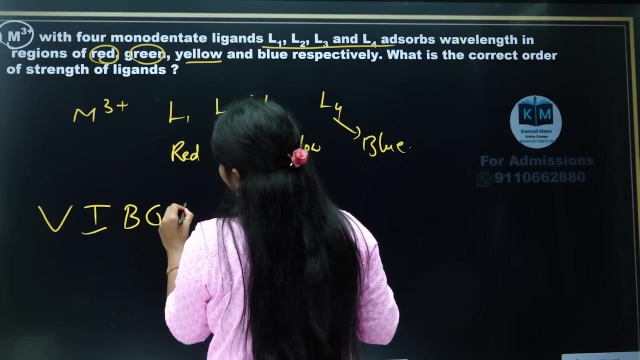 Yellow, Next one is green, Red is green, next is yellow and next one is blue. They were asking us what is the correct order of strength of ligands? Now, see here: VibGR, VibGR. Now take the colors of the complex what it is. 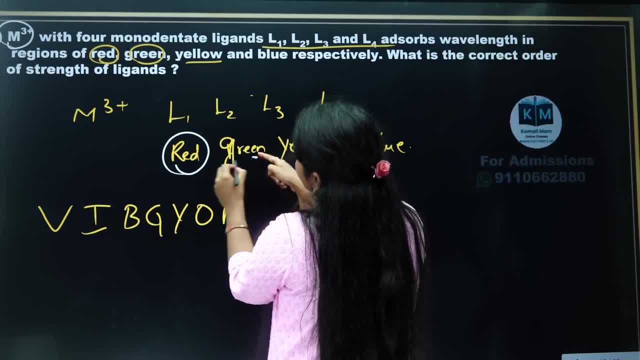 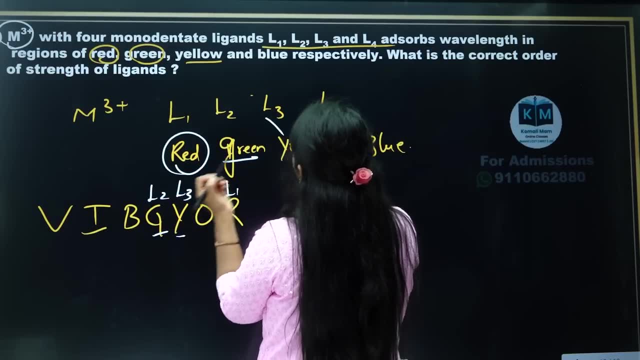 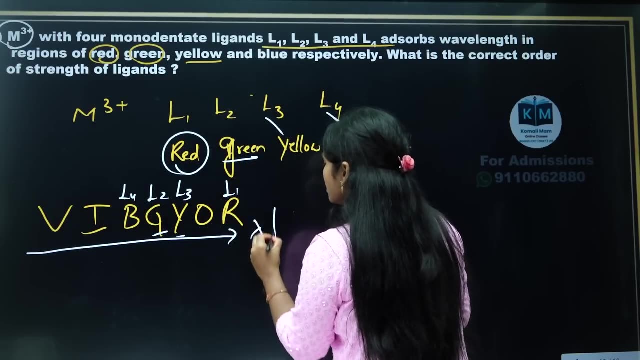 This is red color- L1,. this is green color, next one is L2, next is yellow, this is L3, next this is L4, blue color L4.. So here it is a more wavelength, less energy, less splitting, weak field ligands. 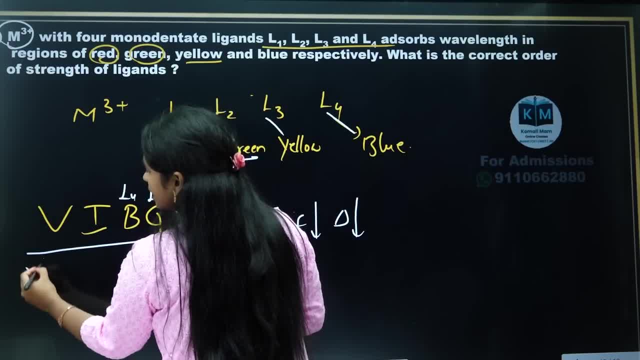 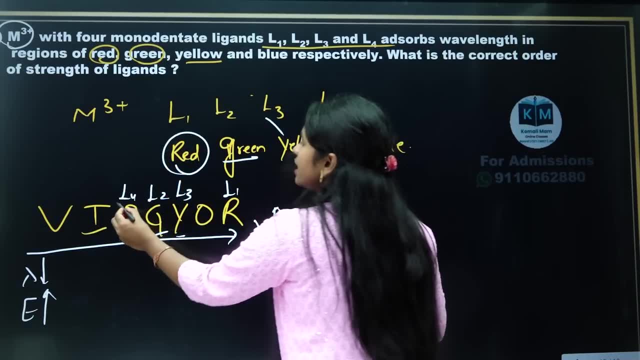 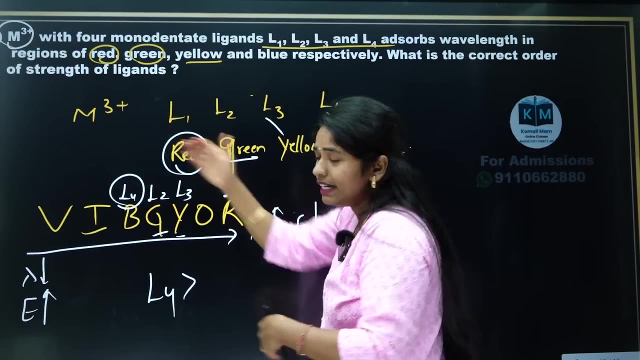 this side, Here, less wavelength region, it is less wavelength, more energy, because energy and wavelength is inversely related. So here this is an. L4 is a strong ligand: more energy radiation it absorbed, less wavelength light it emitted. Next one is L2,, next one is L3,, next one. 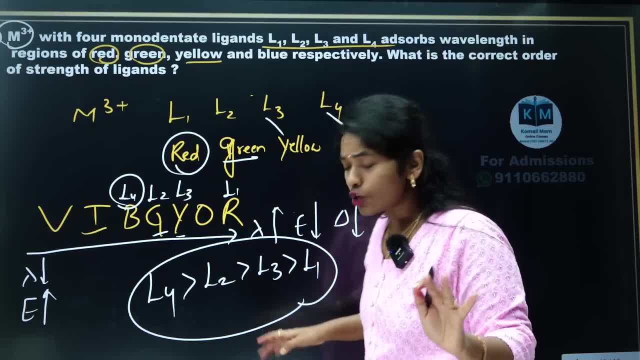 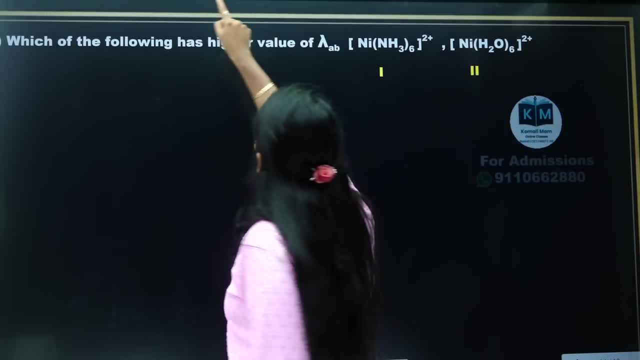 is L1.. This is a correct order. Very easily you can solve you, no need to, you know. worry about the color of the coordination compound. See the next one. Which of the following has higher value of lambda? They are asking wavelength. 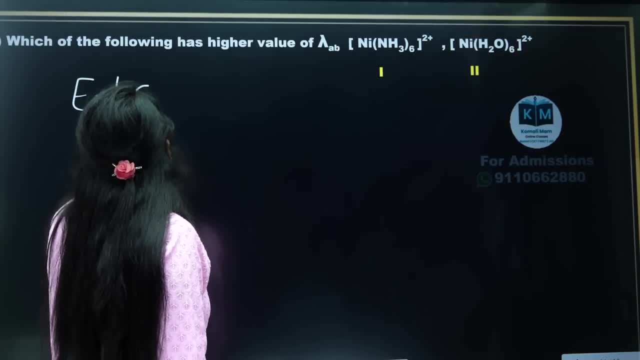 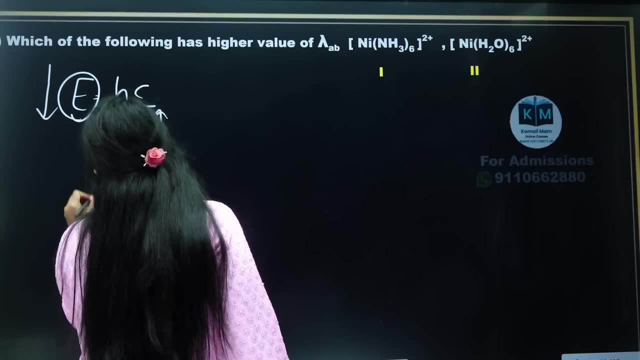 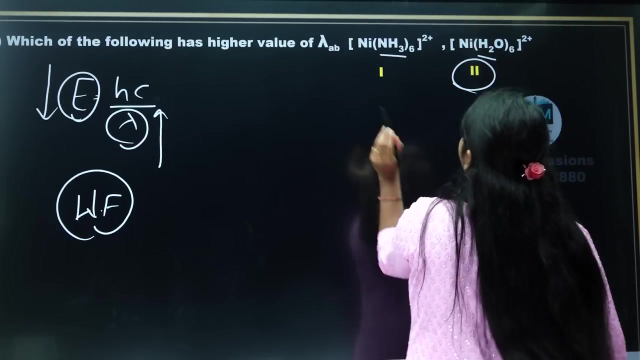 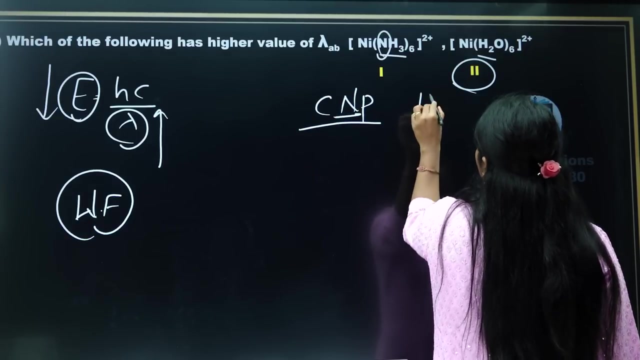 So E is equal to hc by lambda They were asking. more wavelength means less energy, means weak field ligand, weak field ligand. So in this two, which is having weak field ligand, water is weak field ligand, How I found here. nitrogen is a donor. Say no to chemistry and physics in hostile. 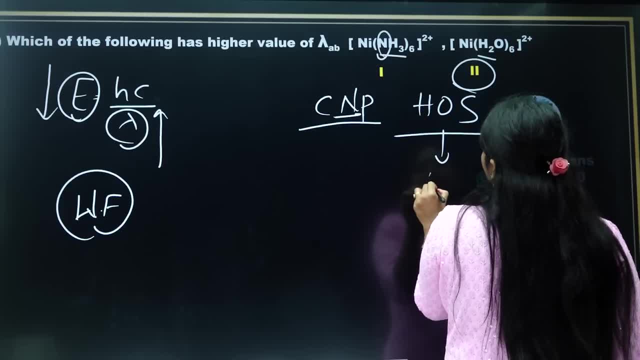 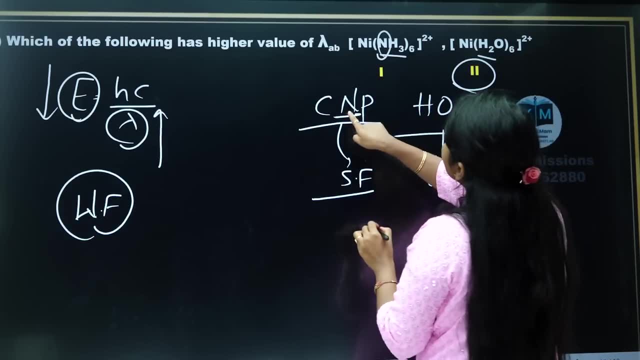 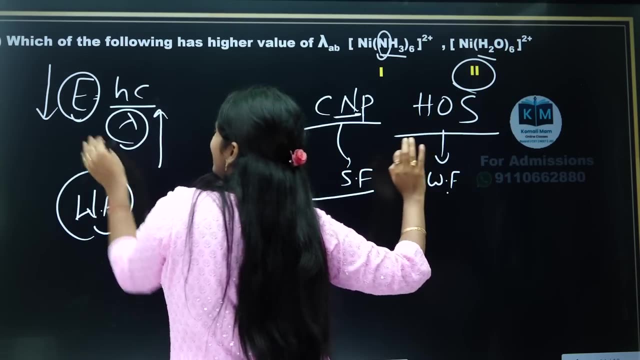 Hostile, hostile is weak field. weak, weak field- This is a strong field. Everybody following this is a strong field. this is a weak field. So nitrogen is a strong field. Strong field means more E- less wavelength. This is a weak field: less E- more. 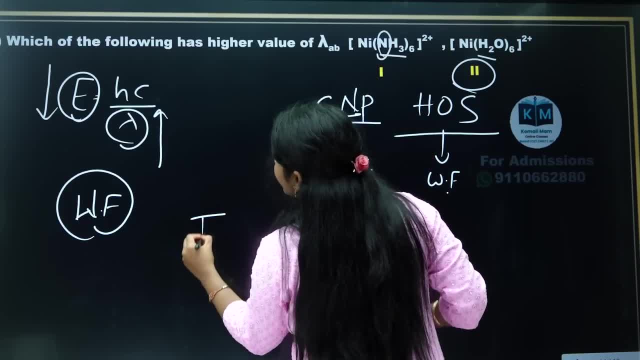 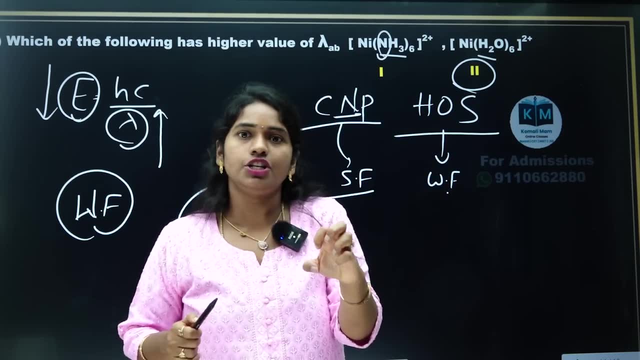 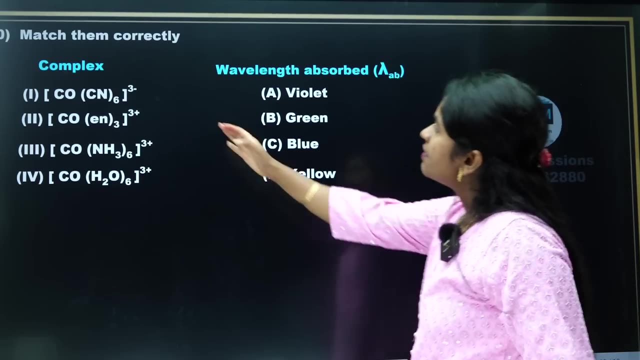 wavelength Are you identifying? So now, 2 is having more wavelength than the 1 because 2 is having more wavelength means less energy, less splitting, Got it? So 2 is greater than 1.. See the next question. They were asking us to match the correct order. How to match, In this case, this type of questions? 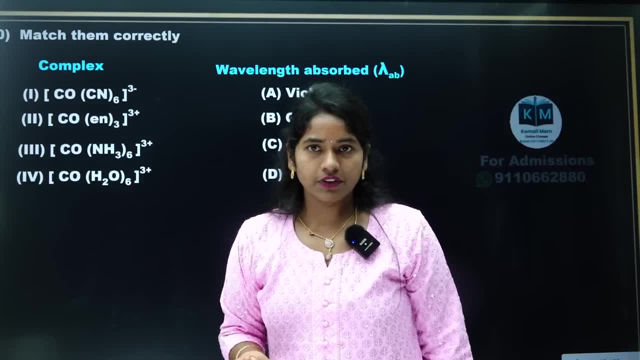 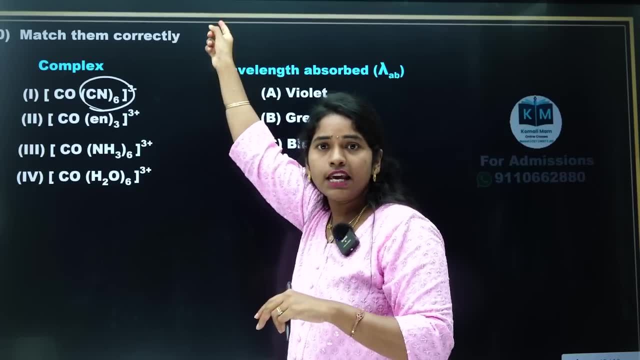 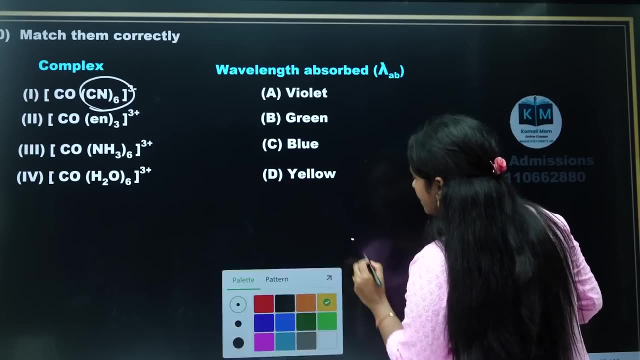 to solve. definitely, spectrochemical series will be helpful for you. Let us see the spectrochemical series order En Cn minus First, CO Cn minus En ammonia. What is that? CO, CO? Tell me CO Cn minus. You should practice this. 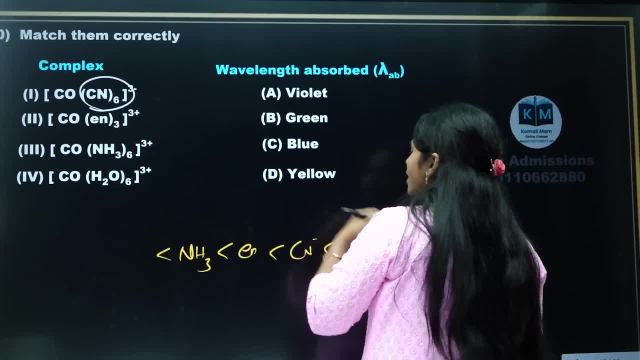 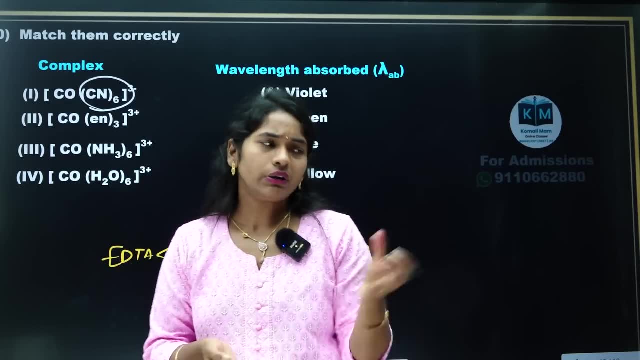 You have to remember very easy. You will be thinking that I should have some mnemonics to remember. Nothing is needed. 4 ligands and 5 ligands combination One time you read out and 5 ligand combination One time you read out. That's it, And like that if you read it easily. 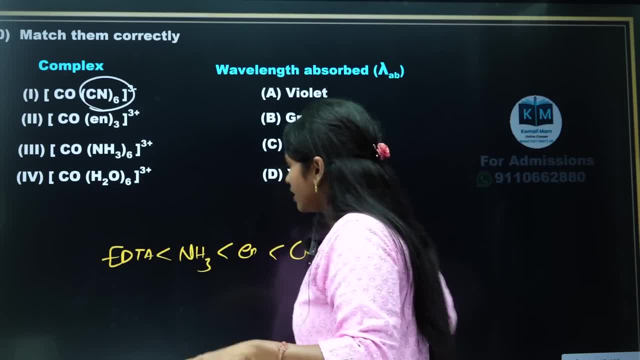 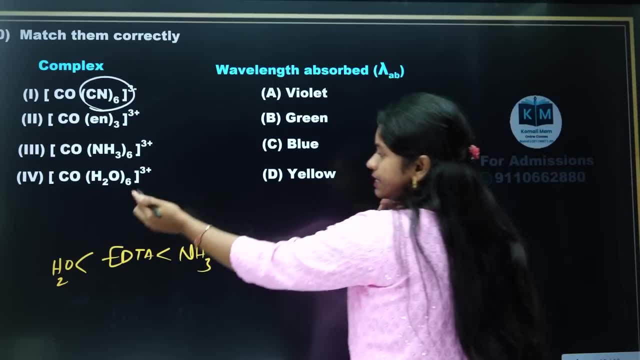 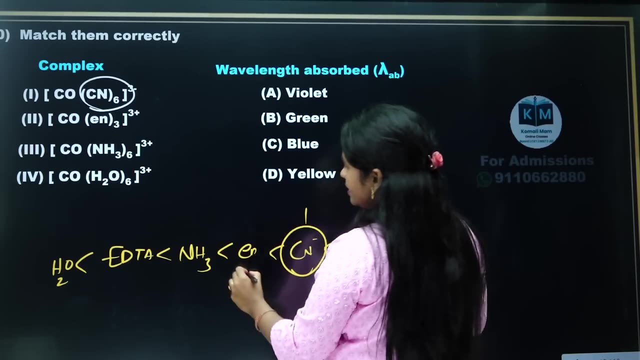 you can remember, it is not at all anything difficult. Okay, Now next one is water Correct And SCC and my NCS minus, then water Correct. I wrote directly: NCS minus, NCS minus, then water. Now, according to this, this is first one And this is next strong. 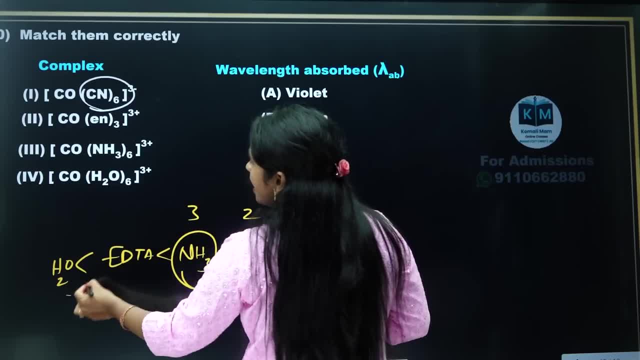 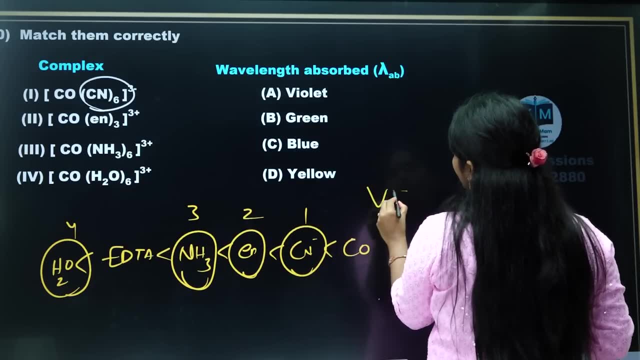 field again Next. this is next strong field again. Next one is: this is water: 1,, 2,, 3,, 4.. So, according to that order: Vib-GR, Vib-GR, Vib-GR. So which one is they have given Violet? 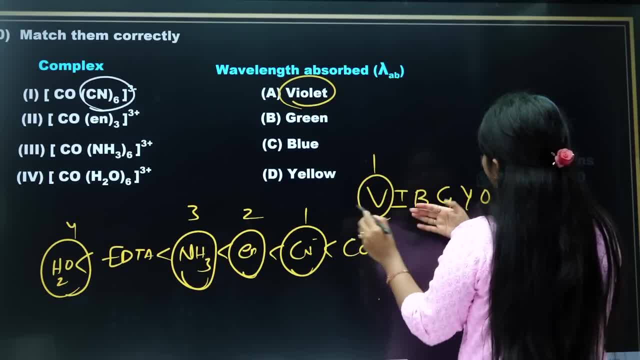 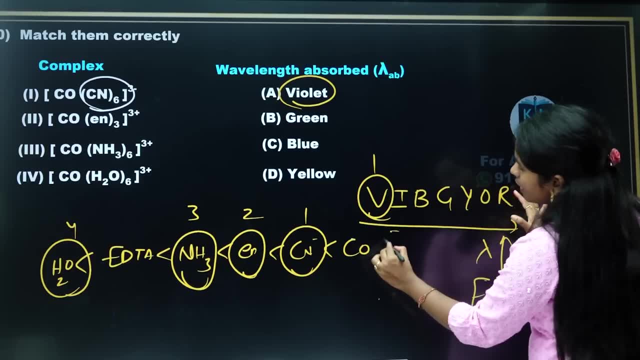 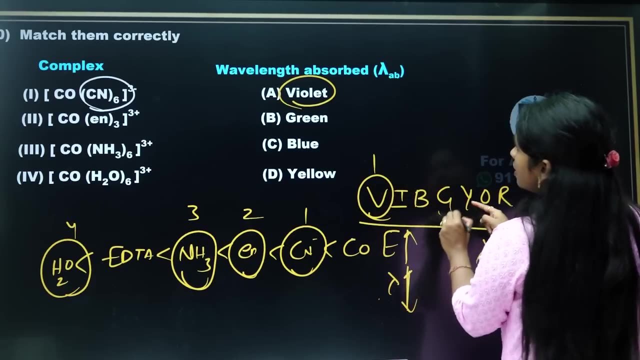 color Strong. Next one is: if you go like this, wavelength is increasing, So here wavelength is increasing, Energy is low energy, Here more energy, more wavelength. Sorry, less wavelength. Okay, So this is first position. Next we should give second position: This is blue, also there. 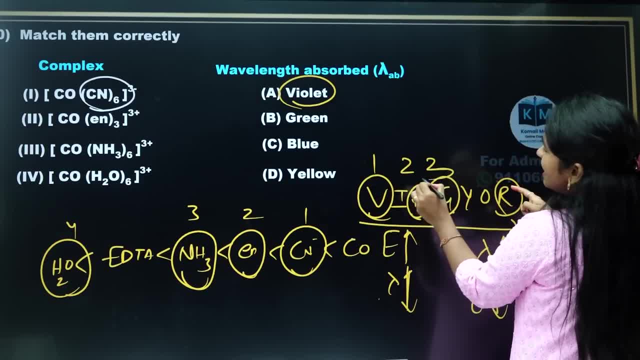 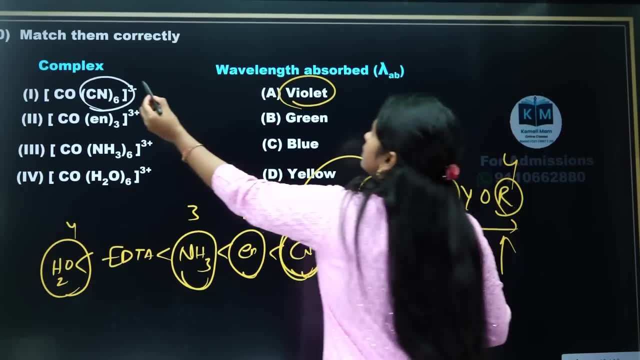 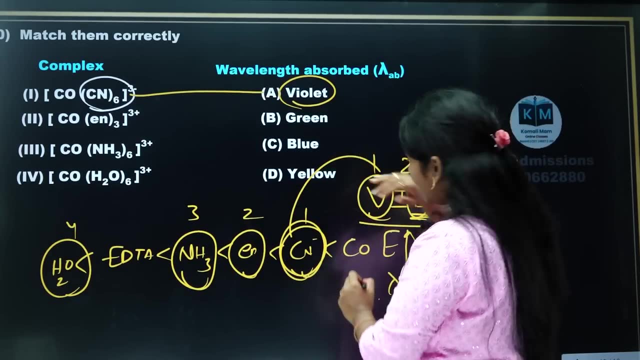 Yellow also there. So blue, we should give second position Green, third position Yellow, fourth position- See how I am doing- CN minus 1. first position Violet, I mean this one. Next. blue is series, next to more energy, That is which one That wave, the wavelength order, is less. 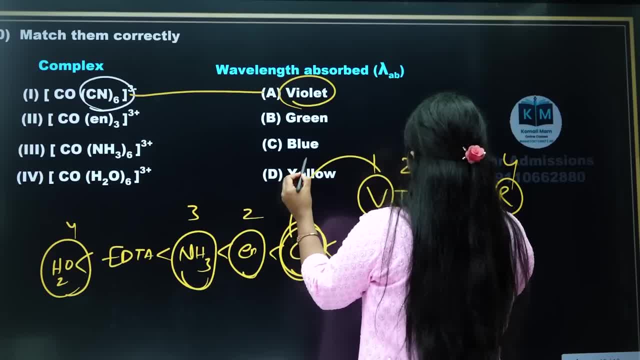 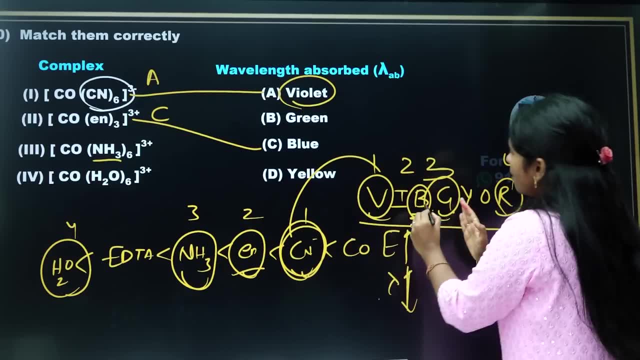 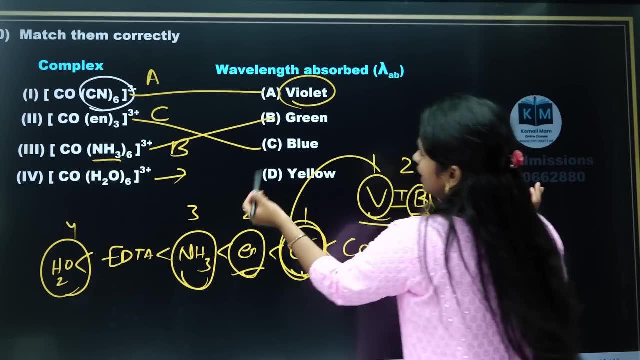 here Blue color. Blue is which one EN which is having EN. So this is a C. First one is A, Next one is C. Next, ammonia, Ammonia is which color? Green color Like this. only you have to solve You, no need to. last one is red. That is which color? Last one is not. 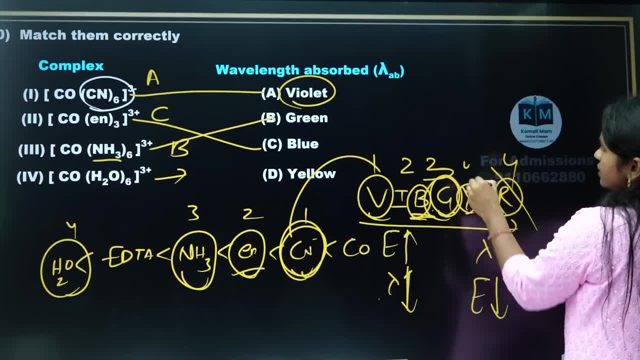 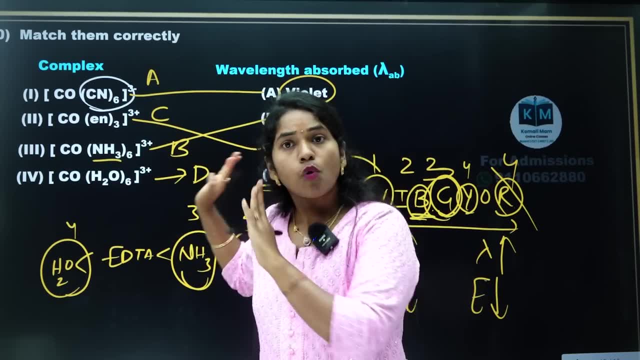 Sorry, It is yellow color. No, I marked Red color, So this is 4.. So this is D What I want to tell You. no need to by heart it. Whatever I am covering in this video, if you just follow it, it is enough. See the next one. 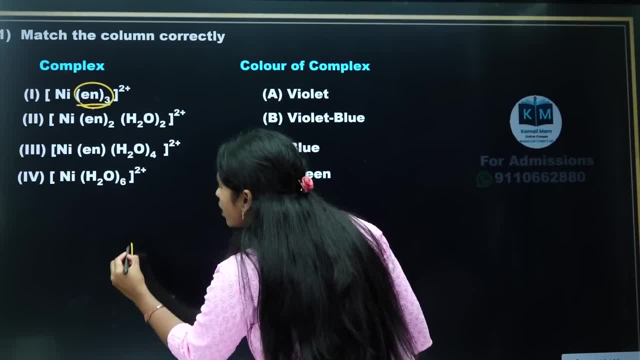 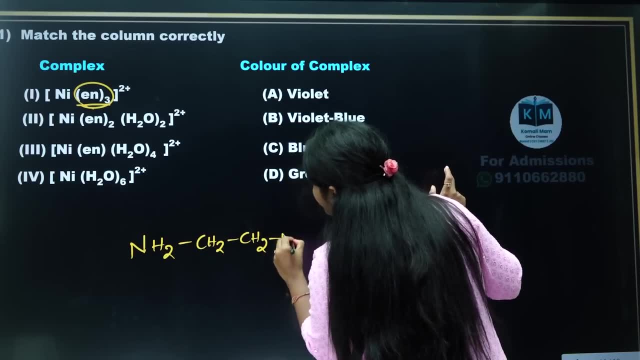 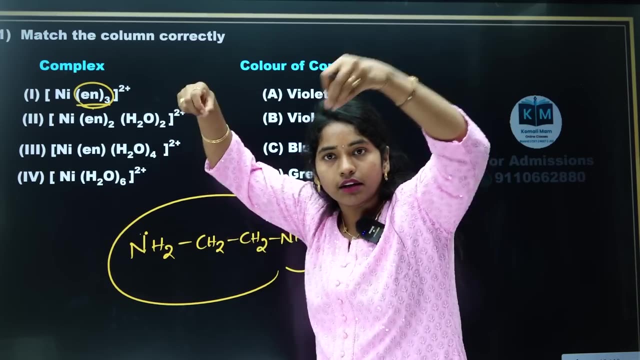 In this case there are three ethylene diamines. What is the structure of ethylene diamine? students See NH2, CH2, CH2, NH2.. This is what ethylene diamine. There are two nitrogens, So two strong fill ligands. A chelation will be formed. Two ligands donate at a time. 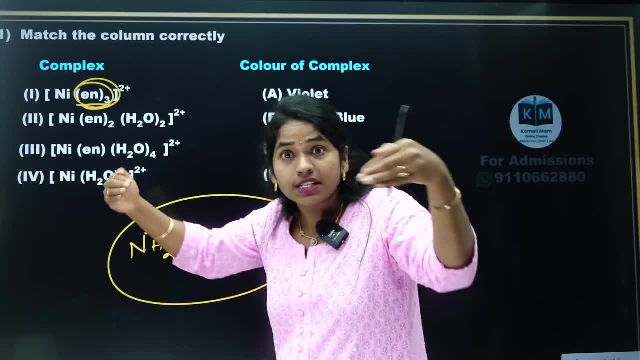 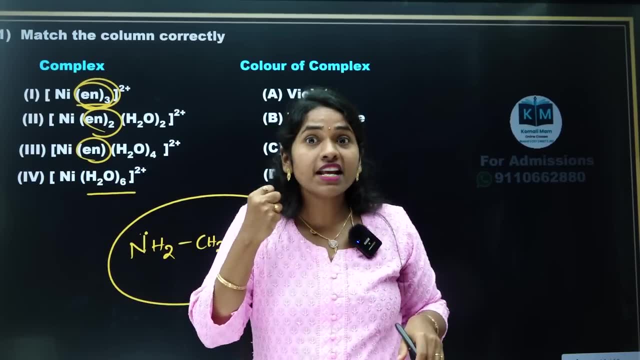 So here two ligands of three ligands are there. which is donating, Chelation is more Here, two ligands Here, just one ligand. Here there is no chelation. More is a chelation, More is a strength of ligand. I mean like a strong fill ligand It is already strong fill. Two: 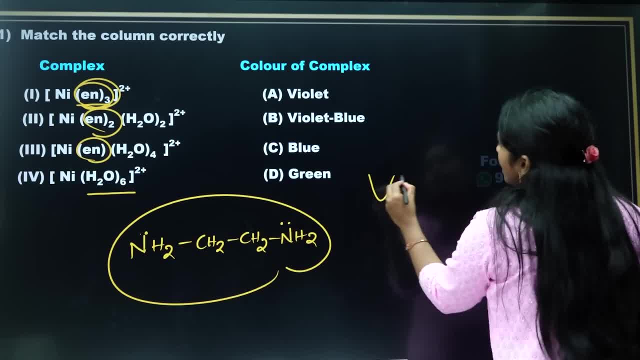 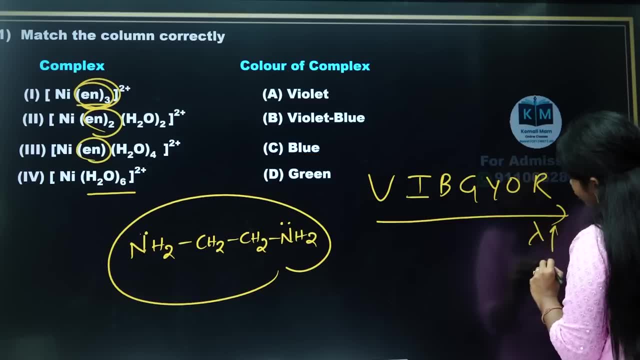 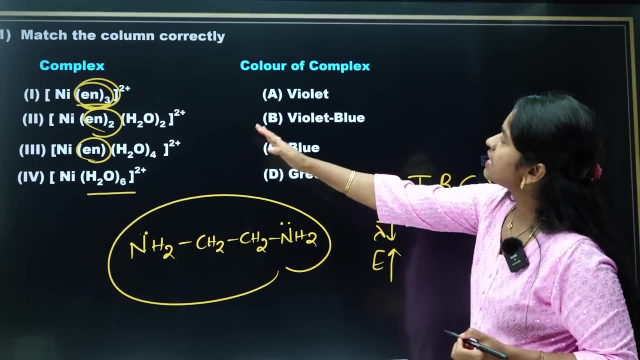 nitrogens, And that two, three ligands are there. So see this color Web GR, See how, or see how easily you will solve in this which is side. this is more wavelength, so less energy is inversely proportional to wavelength. here, less wavelength, more energy. now they were asking us to. 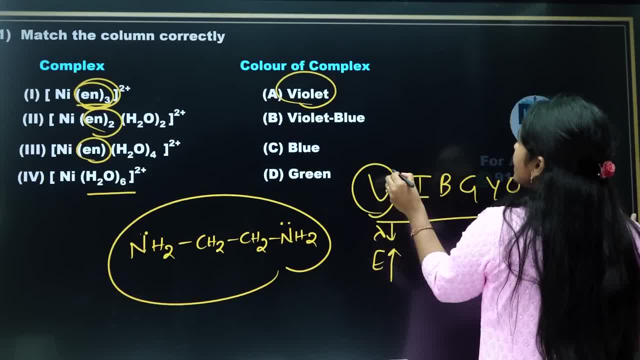 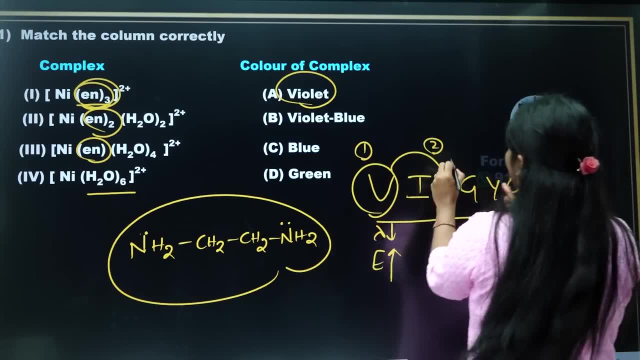 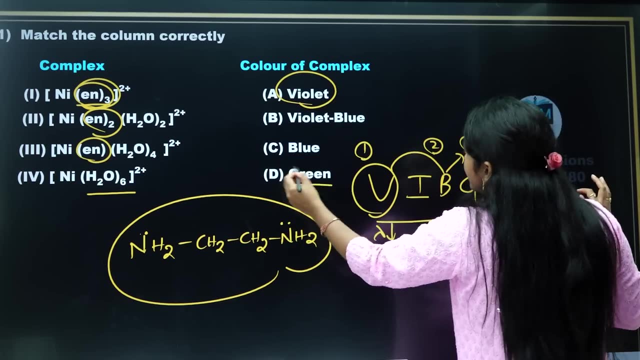 match correctly. what are the colors they have given? violet next to violet. this violet is first one. violet, blue combination. second one: it should be. next is blue, only blue. it should be third, because if you go like this wavelength is decreasing, then it is a weak field. next it is: 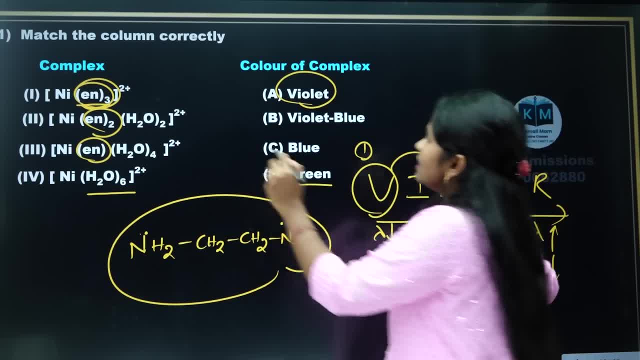 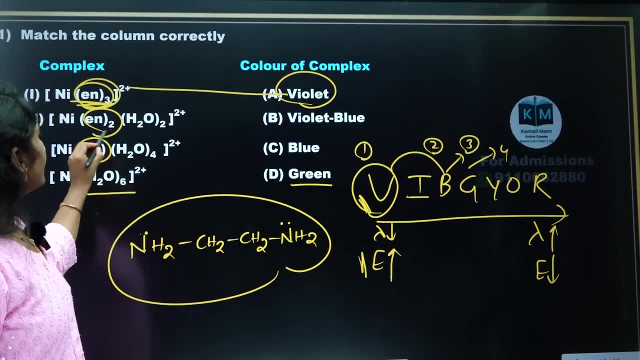 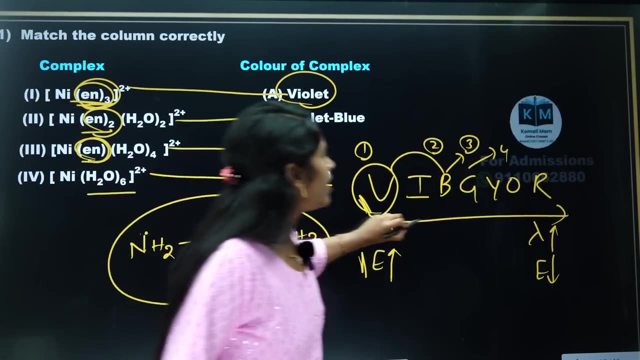 green is four. how i wrote this? more strong field ligands, more splitting violet color. see the next one. two ligands are there here, violet, blue. here only one. as number of strength is decreasing, wavelength is increasing. understand, clear, everybody. see the next one. easy, no, easy, no. 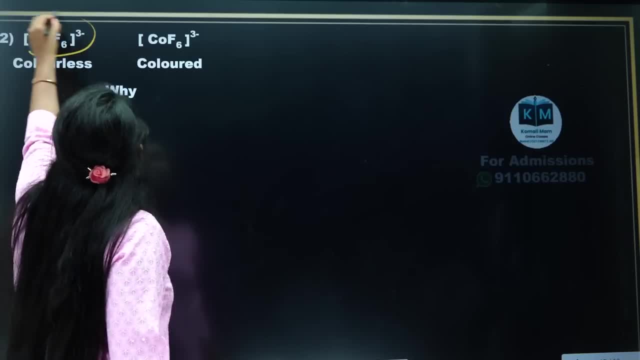 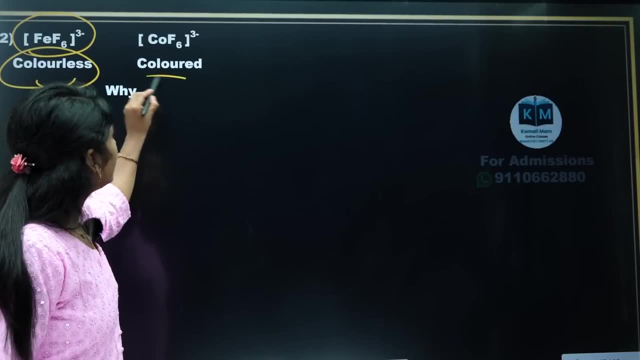 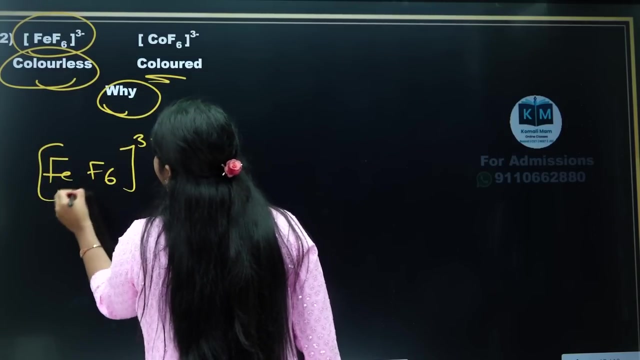 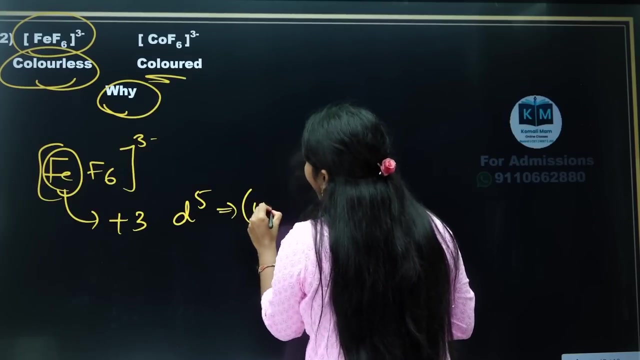 here one question: is there fe f, fe f six, three minus, co f six, three minus. it is colorless and it is colored. why? that is a question. in fe f six, three minus, if you observe, ion is in plus three state means it is a d5, d5 with a weak field, halogens are hostile. in hostile h stands for halogens. 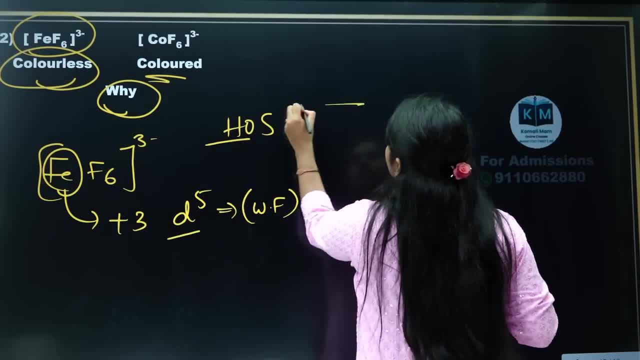 halogens are weakness of the unlimited royal Rams are hostile orажу m in hostile. Ace c is a sweeper in shuttle. h stands for halogens, h stands for thief principle now. so grapes with that colors also have some weak field. d5 combination with weak field. this is actually symmetrical. it don't like to jump. 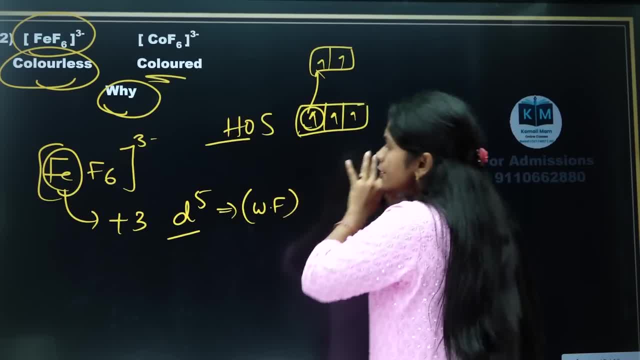 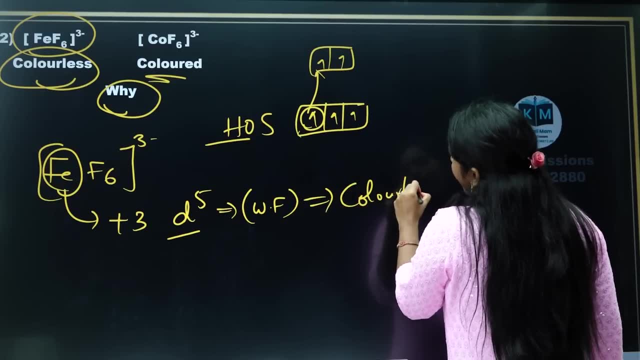 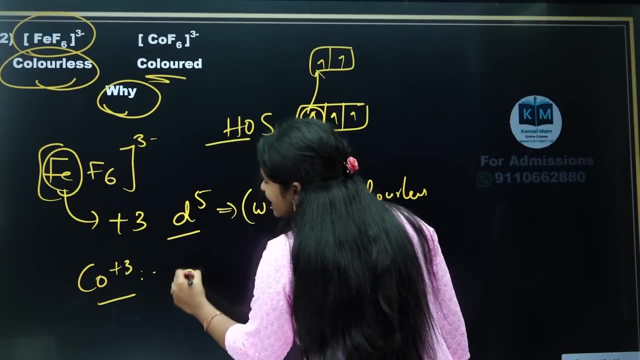 the electron from here to here because it lose its symmetry. so no dd transition and it is colorless. that is the reason it is colorless, correct. and it is having d5 configuration. in cobalt it is in plus three state, so 3d7, 4s2, d6. so in this dd transition takes place and it will be colored. 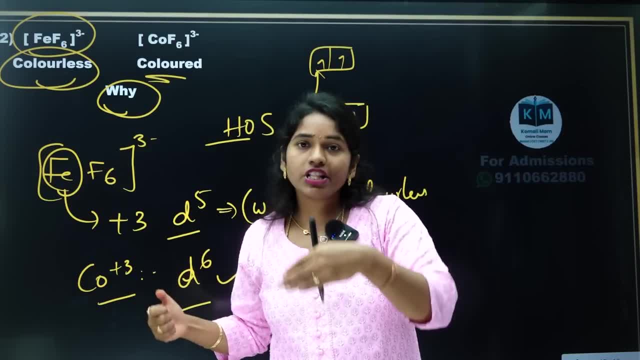 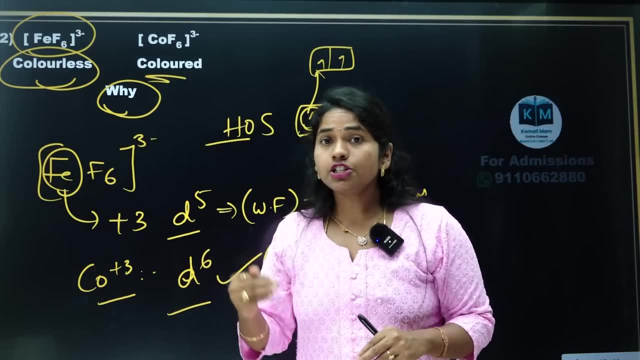 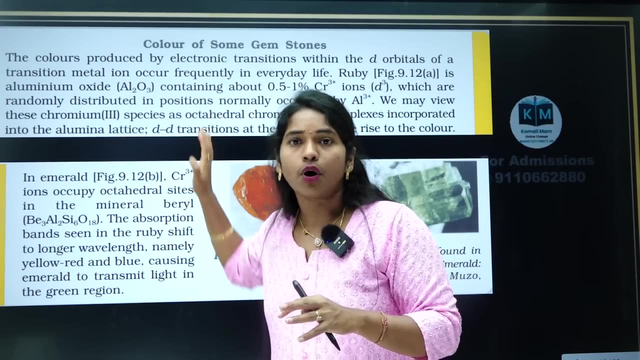 if, in any case, even though it is d5, even though it is d0, even though it is d10, if it is colored, means that is due to charge, transfer, transitions, clear, and here ncrt. one paragraph is given, so i want to cover this also, so everything will be covered. 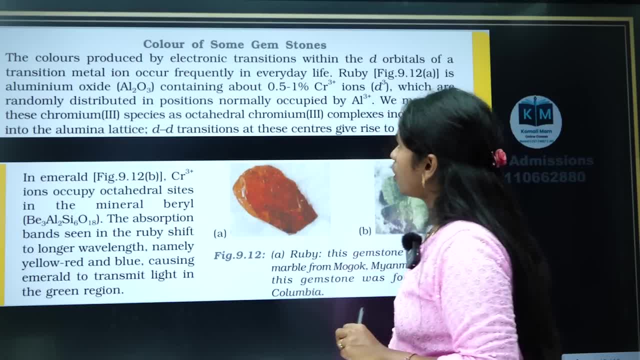 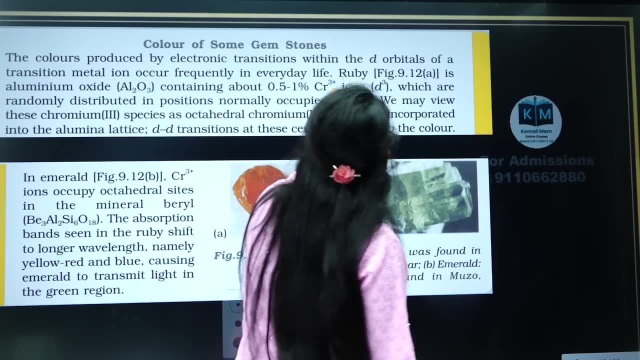 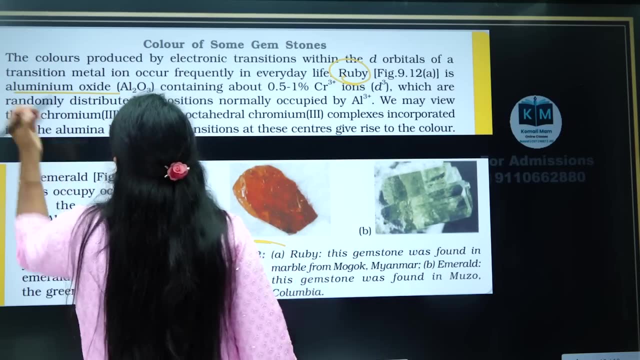 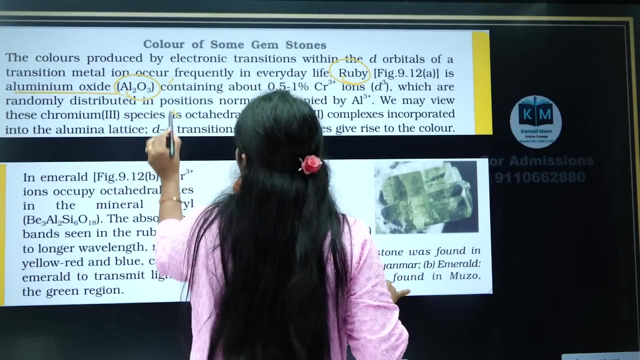 any question you can be easily will be able to solve. see gemstones: if you observe gems like ruby, this is ruby ruby. it is like reddish color. this ruby is nothing but aluminum oxide, al2o3. in this al2o3, if you see in this al2o3 some aluminum, some chromium ions goes and 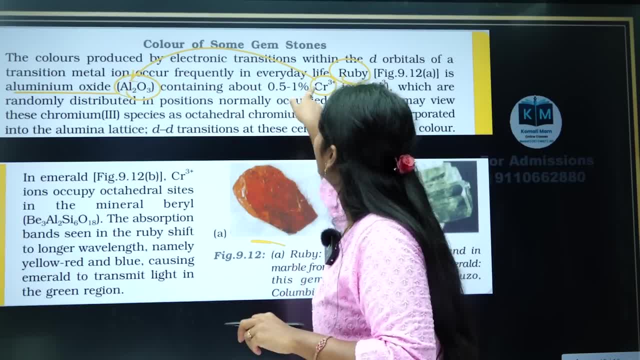 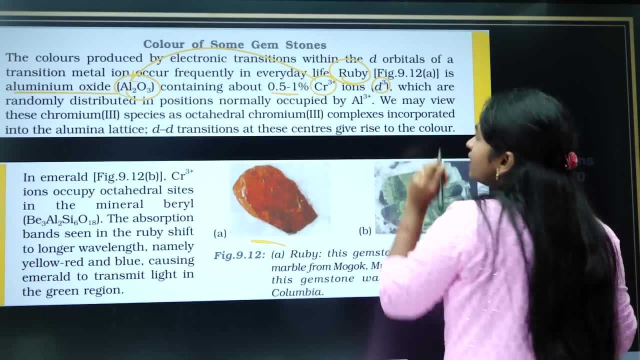 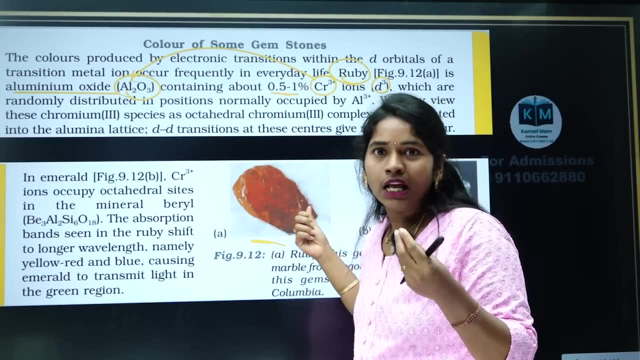 this aluminum ions, some chromium ions will be there, like around 0.5 to 1. because of this chromium ions in cr3 plus there are three unpaired electrons. because of this, dd transitions takes place and it gets this reddish color. okay, this is one question and another question: see, uh, see, this is ruby is. 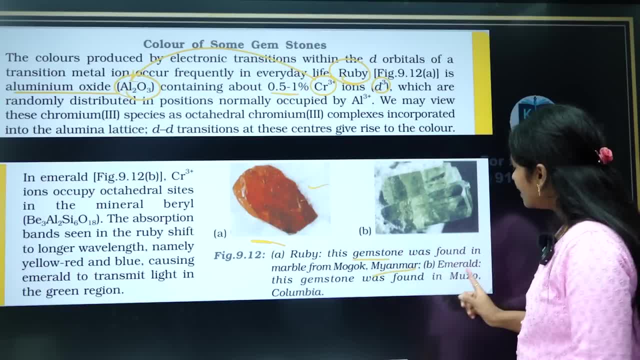 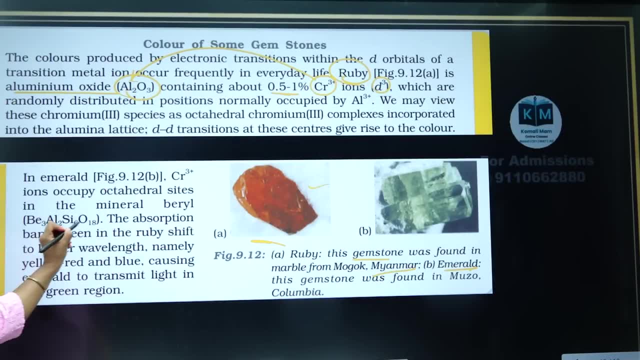 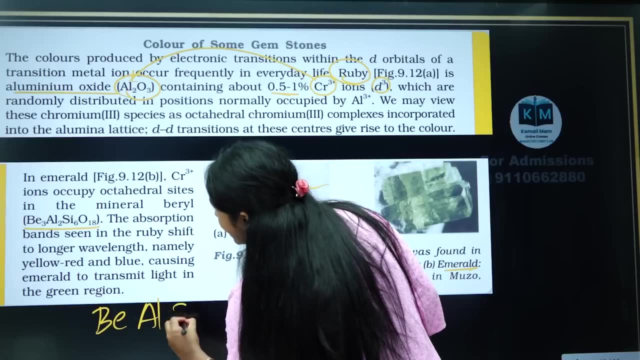 one of the gemstone which we get in mynmar and another one is emerald. emerald is another gemstone which is available in the form of beryl. see the formula of beryl: b e a l s i o. okay, b e a l s i o. 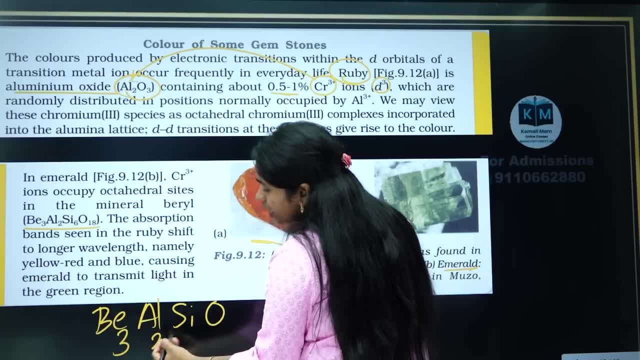 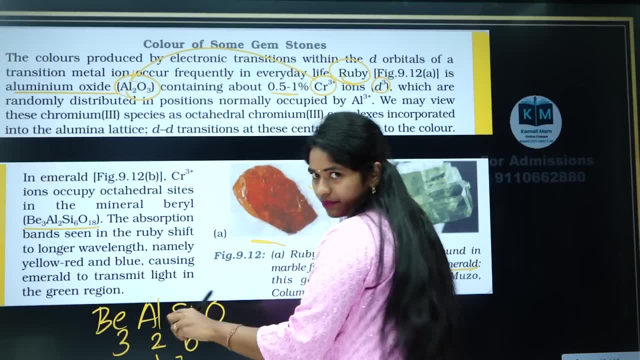 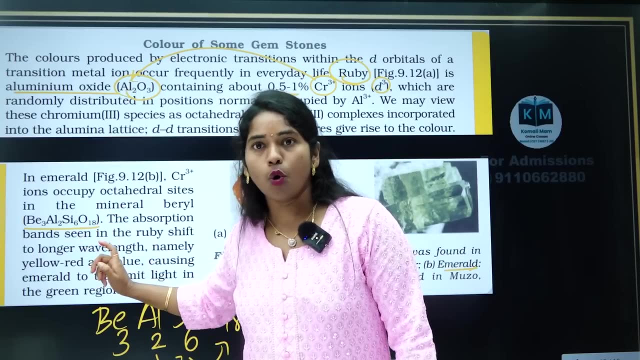 how i'm writing is 3, 2. i'm writing 2, 3, 2. okay, 2, 3s are 6, 2. i'm multiplying 2 with the 3. 2, 3s are 6, 6, 3s are 18.. b e, 3, a, l, 2, s, i, 6 o 18. this is a mineral. 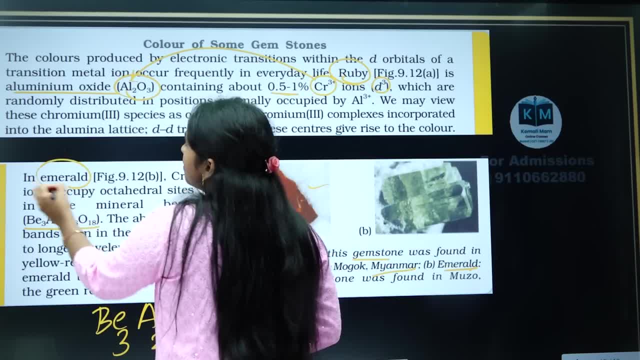 in this mineral? we will. this is called as emerald, which is having chromium ions. this chromium ions goes and occupy the spaces in the todo condition of this. that errol, which new it is. chromium ions goes in the occupy Khara and this few other people with chrome. 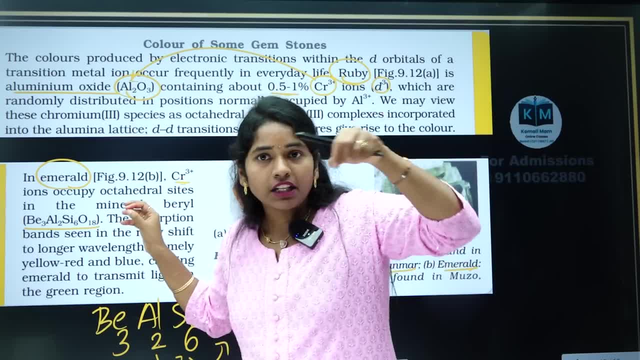 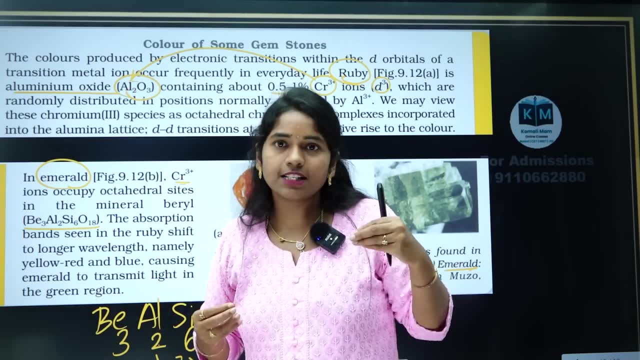 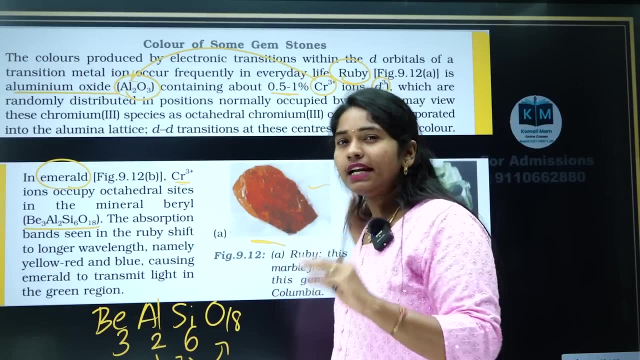 and the ones, and because of that it goes and occupy the octahedral sites and all in both. so because of that it gets, the color transitions takes place and this color will be like green color. we can't see in ncrt that much green color, but usually it is light green and dark green color, gemstones also. 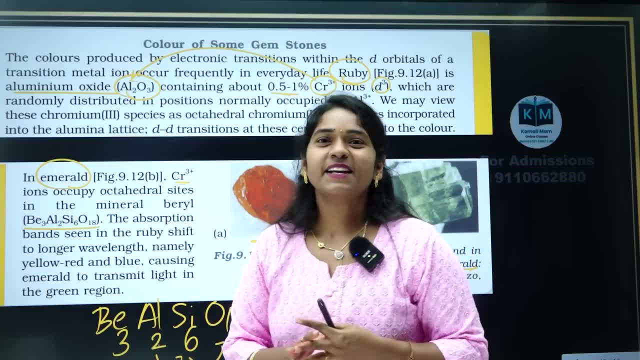 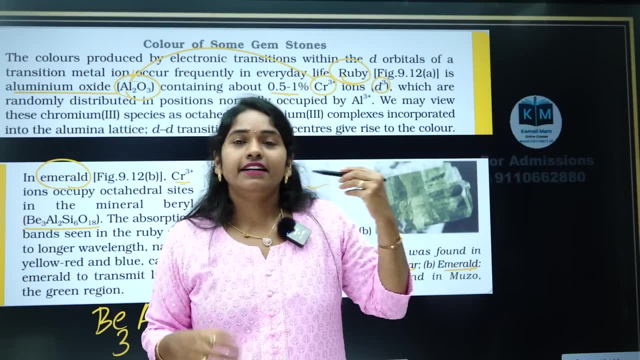 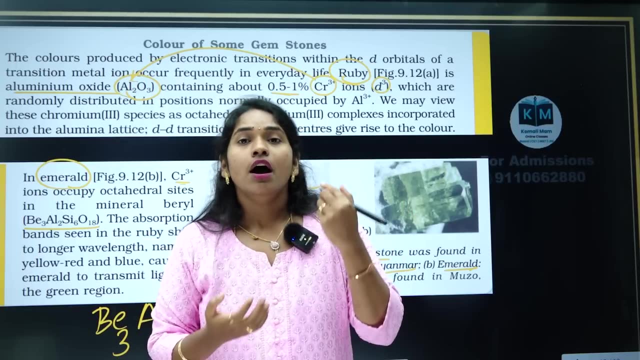 available. that's it. i hope you like this video. thank you so much for watching this video. if you are watching for the first time, go through komali ma'am channel. so many tricks are there. this tricks will make you understand the concepts in an easier manner. if make the notes. notes of 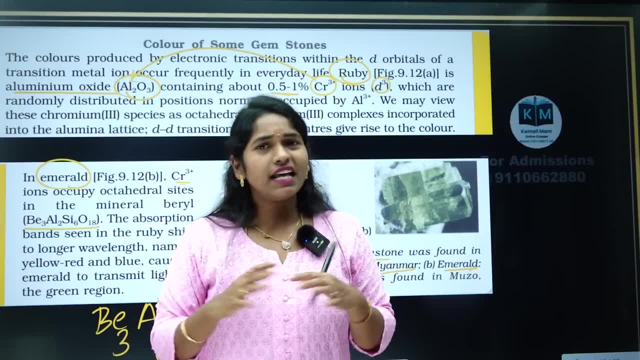 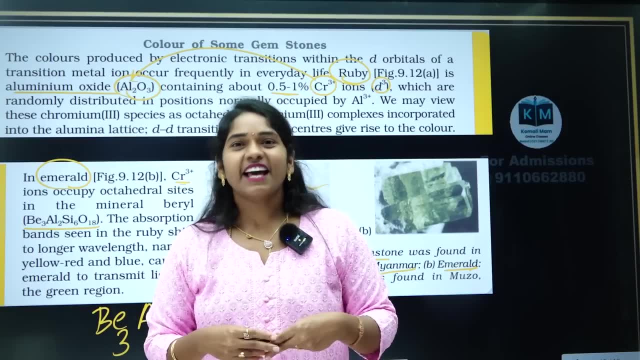 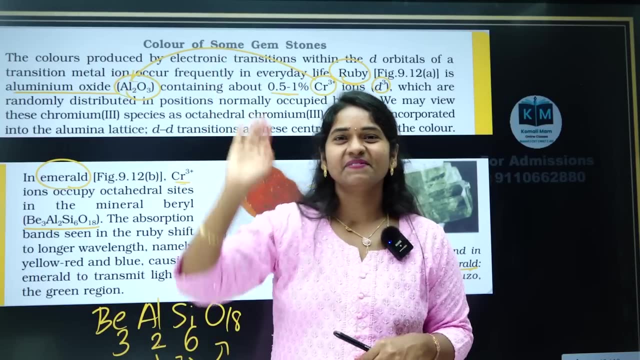 this solve the questions. whatever i have given in this video, that's enough. you will solve almost all the questions, from color, from the coordination compounds. thank you so much for watching this video. see you in another video with excellent concepts and techniques. bye, bye, all of you, take care.